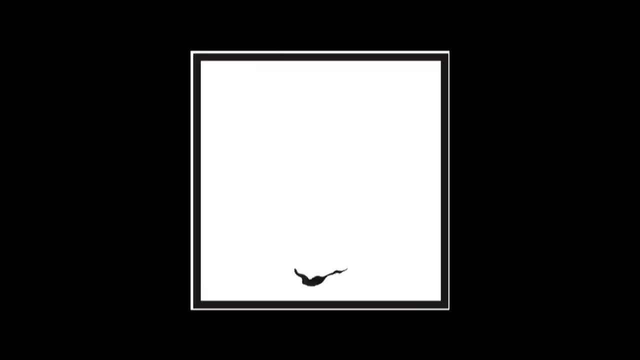 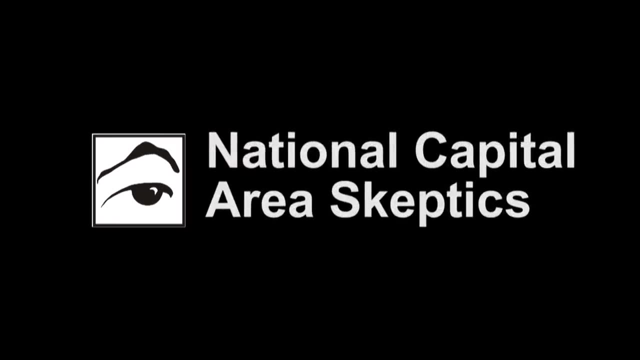 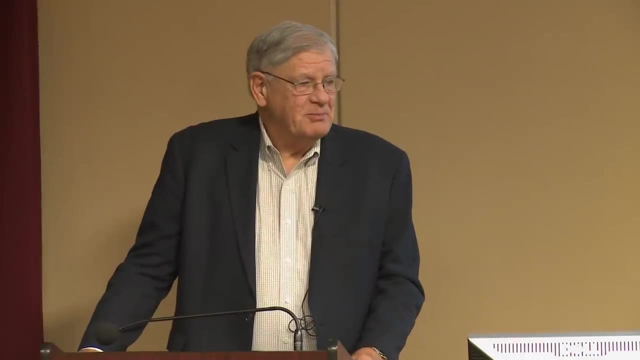 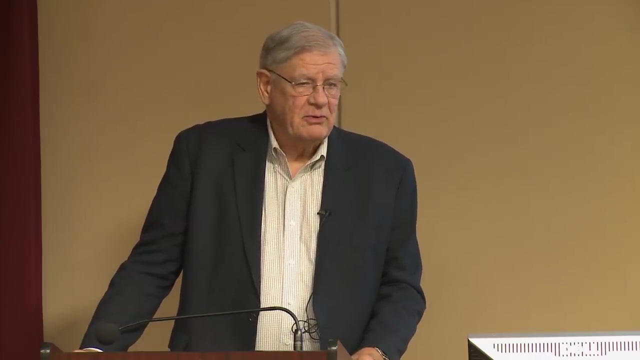 Thank you. It's a pleasure to be here and I can talk a little bit about a subject that's kind of been near and dear to my heart for about the past 42 years, and that's nuclear safety. As Marv said, I actually started before there was a Nuclear Regulatory Commission. 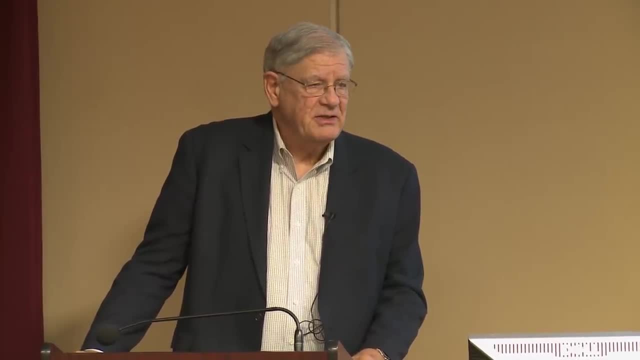 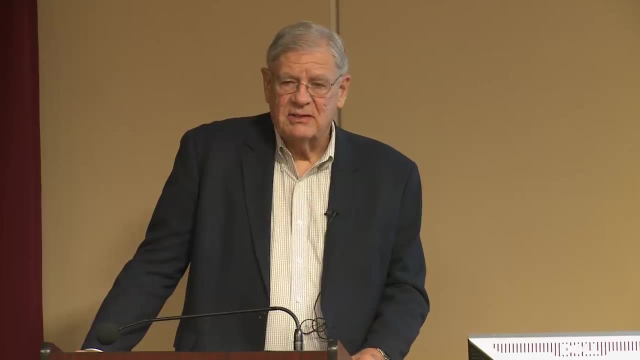 There was an Atomic Energy Commission and I started there in 1973 and started working on breeder reactors, which are liquid sodium reactors. However, that was premised on a thought that we only had 25 years of proven reserves of uranium and therefore we needed to breed plutonium as a fuel, But since then it was discovered a lot more uranium reserves, so breeders were not as urgently needed And also because it was a new technology, utilities quite honestly are very hesitant to just jump in and say, hey, I'll be the first one to. 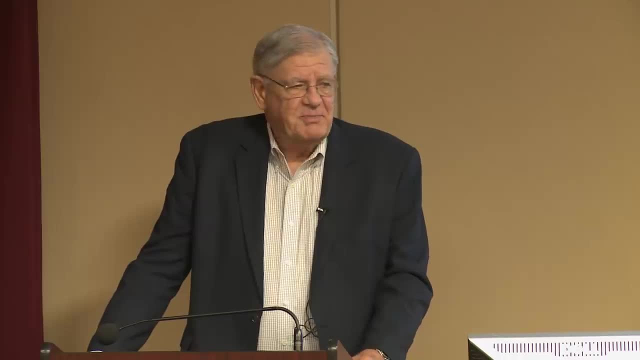 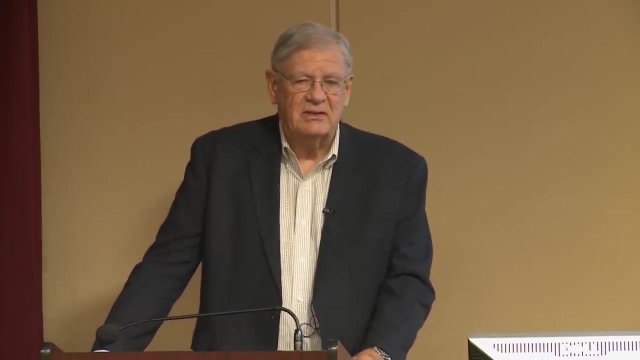 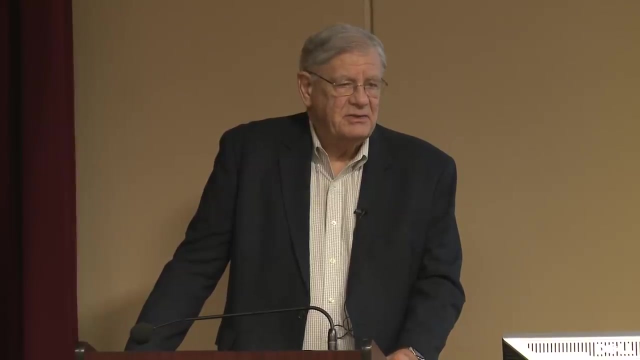 do that. They want to demonstrate it. So, anyway, I spent most of my career working on current-generation water reactors and I happened to be in a position at the Nuclear Regulatory Commission when TMI happened. that I was – I got heavily involved in the accident, analyzing what happened, trying to determine. 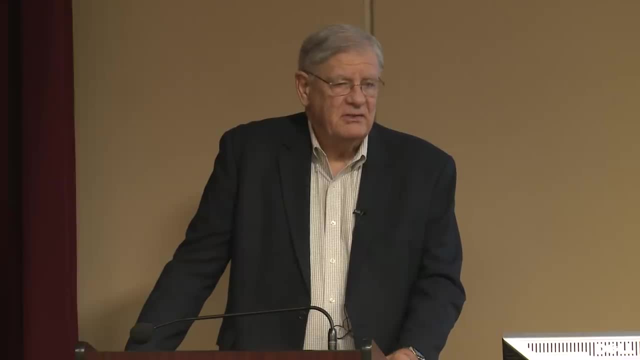 what the lessons learned were, what needed to be done differently, and they were all going nowhere And I had a lot of technical issues that came up. Then, in 1986, Chernobyl happened and I was in an office, I was a deputy division director. 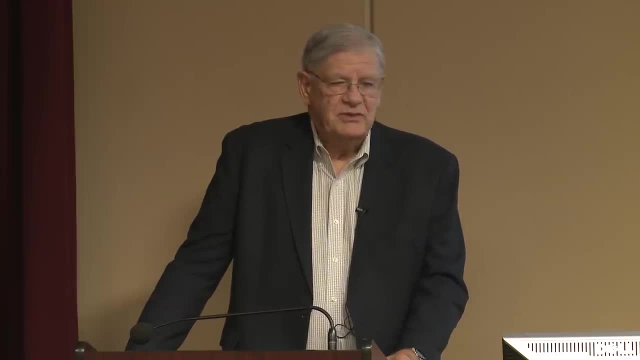 in an office that was charged with basically trying to understand what happened and what does that mean for US reactors. So I was heavily involved in Chernobyl. I was on the US team that went to Vienna in August of 1986. 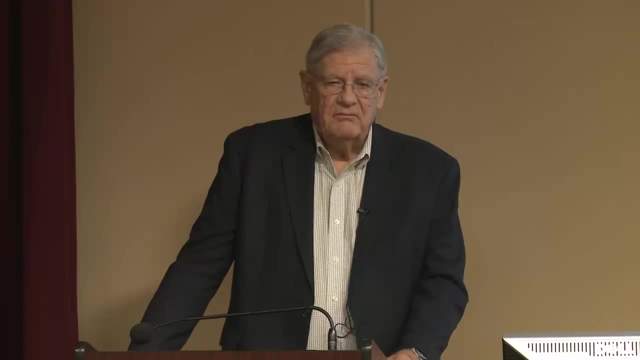 when the Russians finally announced their side of the story of what happened, And then, most recently in 2011, when the tsunami hit in Japan and Fukushima reactor had the meltdown. actually, the three of them had meltdowns. I was heavily involved in that as, again, part. 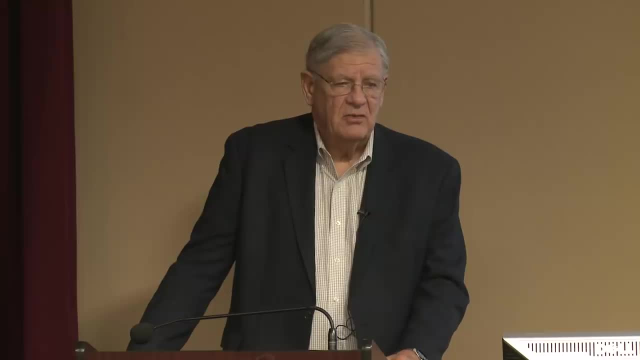 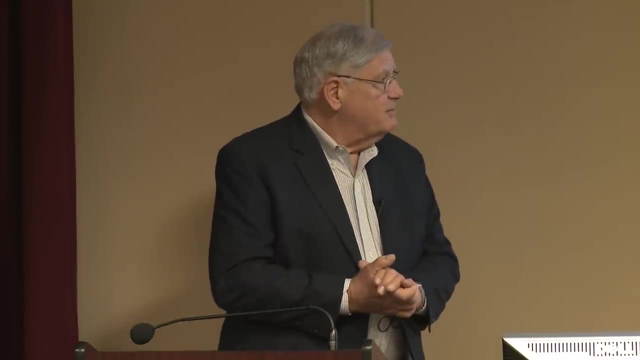 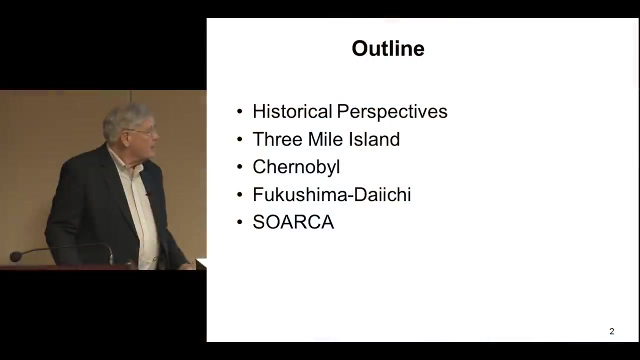 of the research office, again trying to understand what the implications were for US reactors. So that's kind of my background in terms of where I got all my information and I've accumulated this over the years. so we'll start The last item there. that's not a reactor. 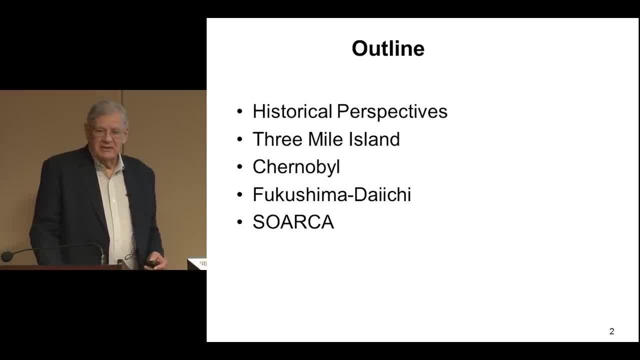 SORCA is an acronym. We live in acronyms in the government. It's state of the art. It's a state of the art report on severe accident analysis. That's a SOR actually. it's consequence analysis. state of the art report on consequence analysis. 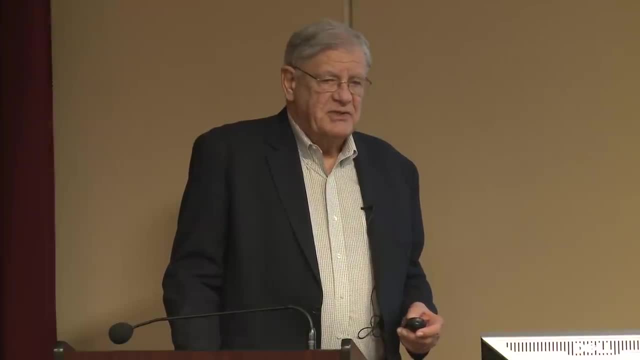 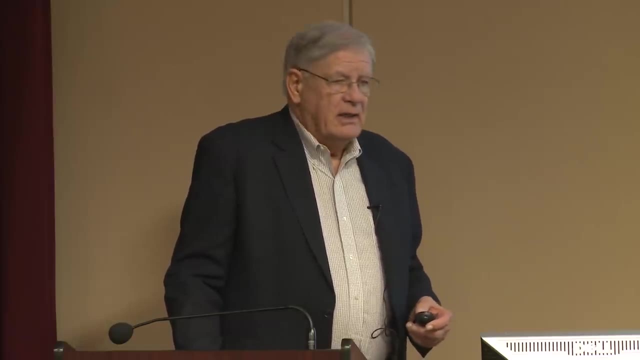 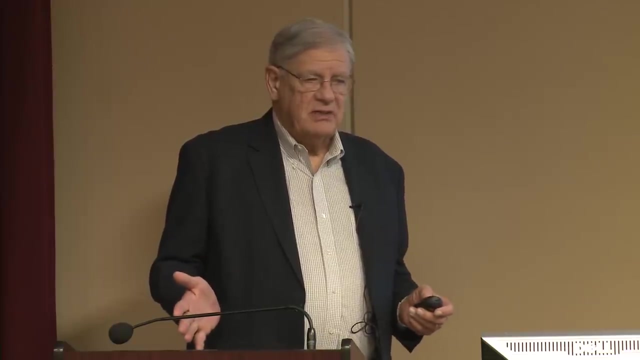 And what that is is a study we did, my office did- we were just finishing it up- actually we had just finished it right before I retired- on what we believe the most realistic consequences would be If there was a core meltdown in the United States at a reactor. and I'll talk a little. 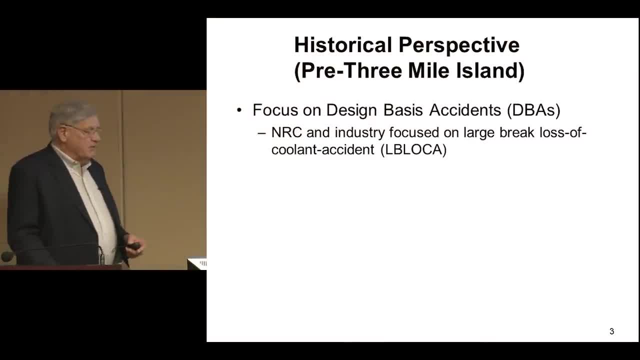 bit about that. Let me first talk historical perspective, and this goes back to when I first joined the agency back in. I actually joined in 76,, the Nuclear Regulatory Commission. But when I got there what I noticed was their focus was on what they call a design basis. 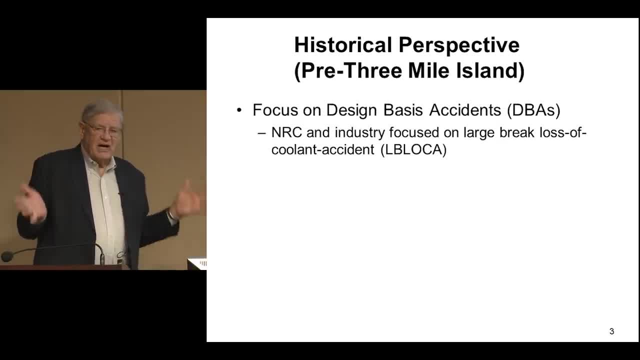 accident. What's that? Well, that's something that you design a plant to withstand and it's a very stylized accident, And at that time, the design basis accident for nuclear plants was called a large break: loss of coolant accident or a large break LOCA. 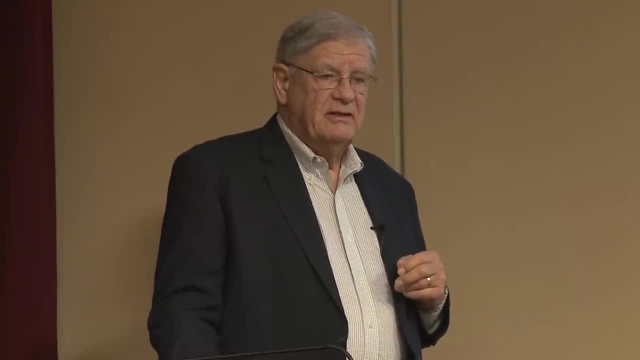 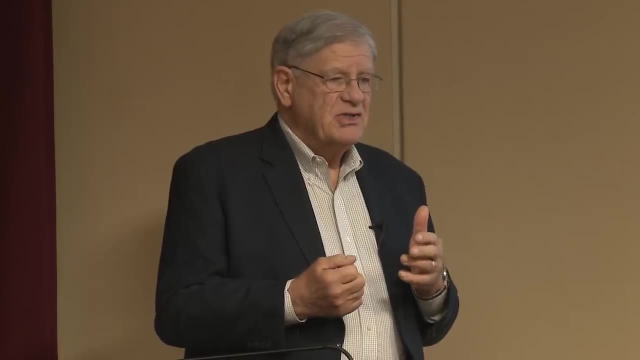 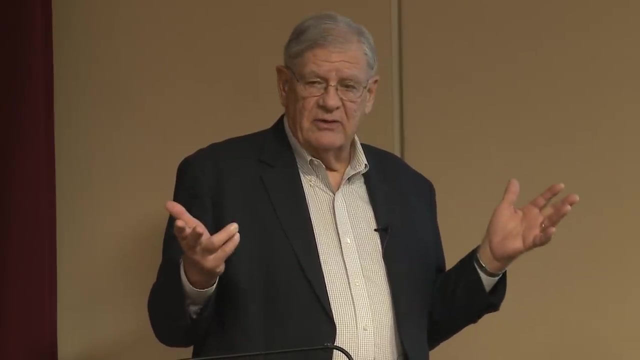 And what that was, was you postulated that the cold leg in a reactor, which is the water going into the reactor before it gets heated up Suddenly, it's about a 30-inch pipe, okay, they're very big, And these reactors run at anywhere from like 2,200 pounds pressure, which is very high. 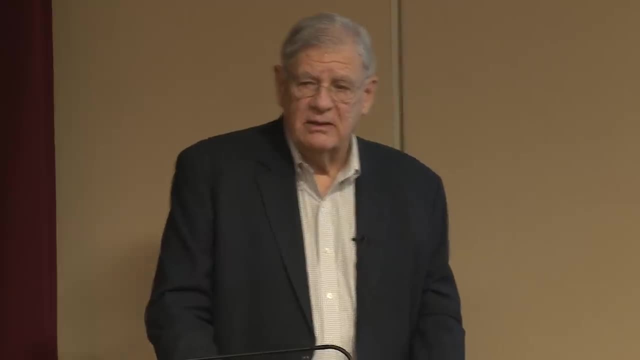 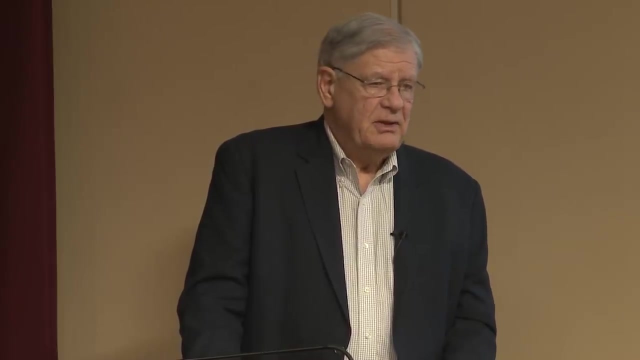 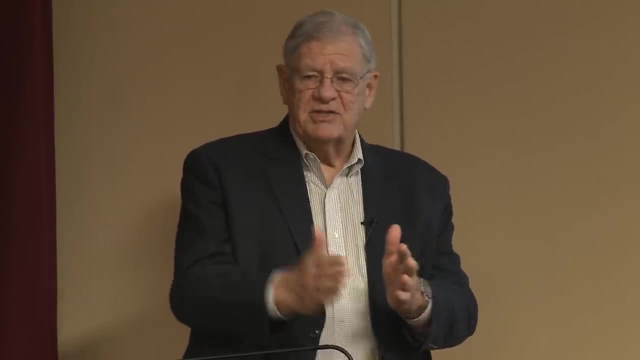 for a pressurized water reactor to maybe about 1,100 pounds pressure for a boiling water reactor. But what you assume in this scenario is that this pipe suddenly has a guillotine break, like somebody could take a water pump. Somebody could take a butter knife and just cut straight through. okay, And this pipe would suddenly separate. so water would, this high pressure water would gush out of both ends of the pipe and you would lose cooling to the reactor. And so that was the design basis And what the designers at the time- Westinghouse, General Electric, Babcock and Wilcox- and 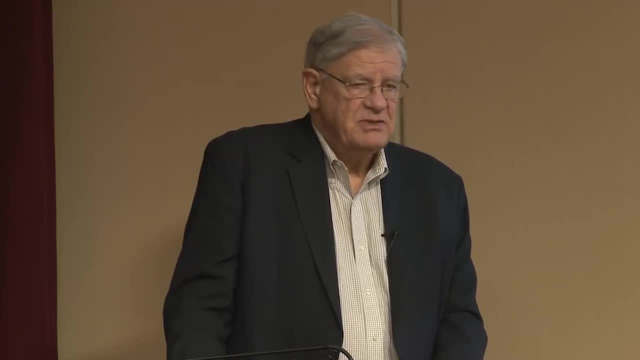 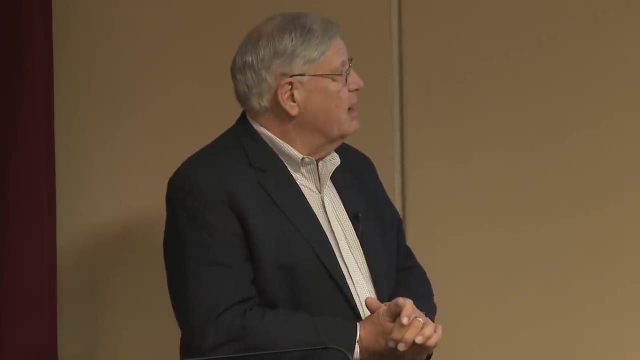 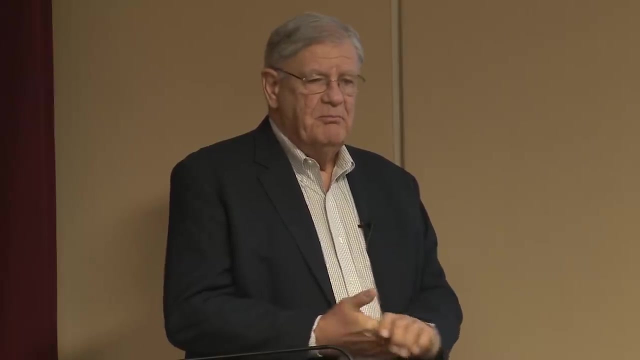 Combustion Engineering had to do was put in safety systems that would protect the fuel so it wouldn't melt, And that was the design basis, And we focused all of our time and energy on trying to prove that. There was millions of dollars of tests run at facilities around the country where they 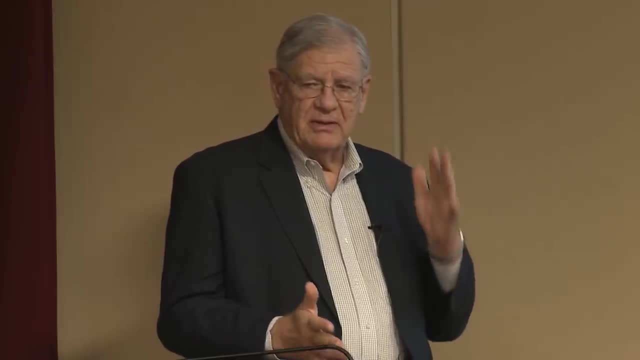 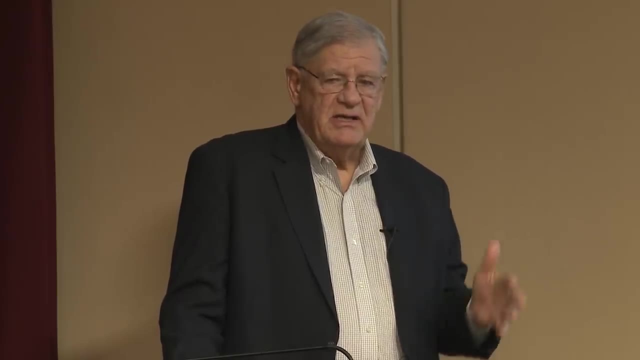 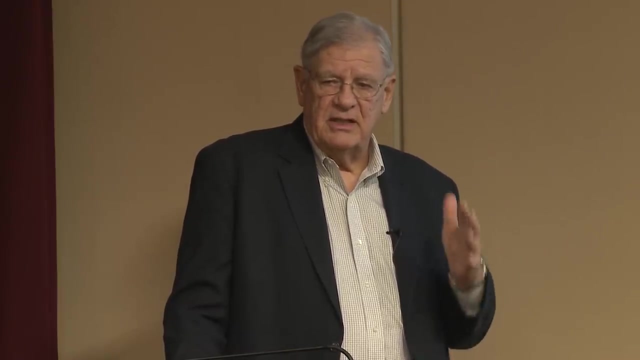 would try to simulate this breaking of a pipe and watching what happens. There were heat transfer loops where they had electrically heated bundles, fuel rods, but instead of being nuclear they had electric current going through them to simulate the energy, And they culminated it with a facility out in Idaho at Idaho National Engineering Lab. 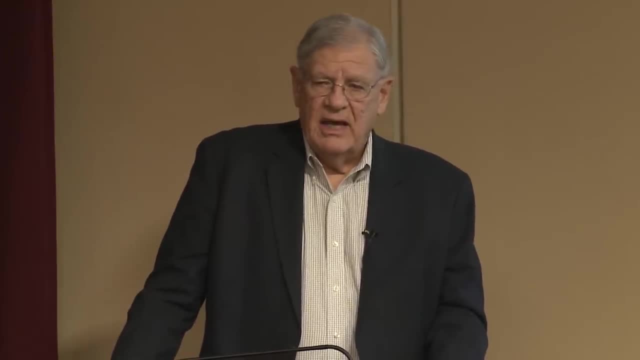 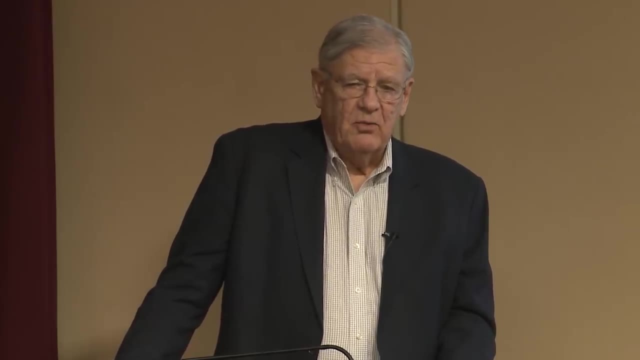 called LOFT, which is the loss of flow test. And that was a real reactor. okay, nuclear, had nuclear fuel, But it wasn't a full-scale reactor. The core was not as tall and it wasn't as big. It was a small scale. 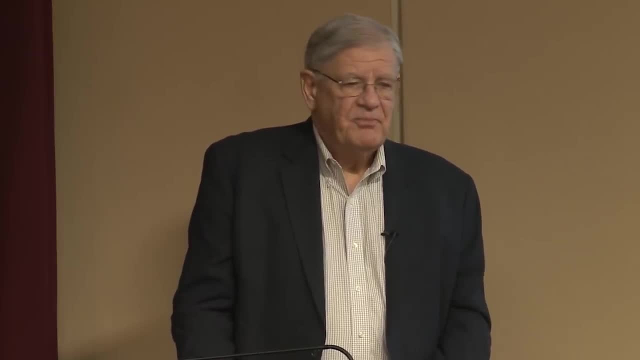 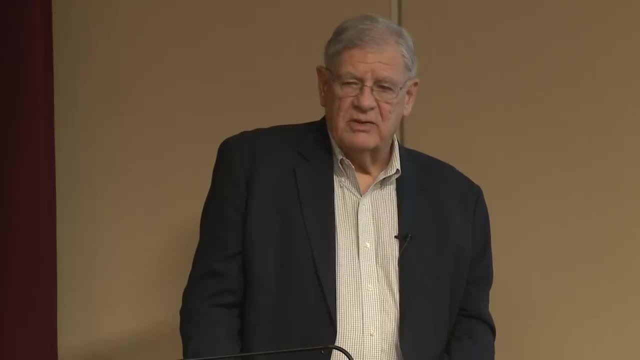 Obviously it wasn't a full-scale reactor, Obviously because of the costs, But they actually ran a test where they simulated breaking a pipe to see whether or not this fuel was going to melt or not or whether the safety systems would actually kick in. and 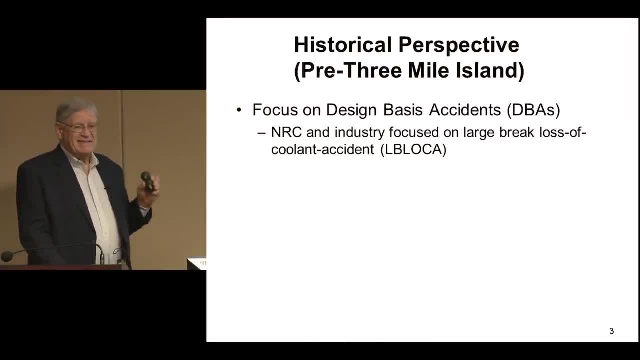 keep it cool. So that's the basis. That's what plants- nuclear plants- were designed to And that's what everybody focused on back in the 70s. It was based on what they call a defense in depth strategy, and that is that you don't. 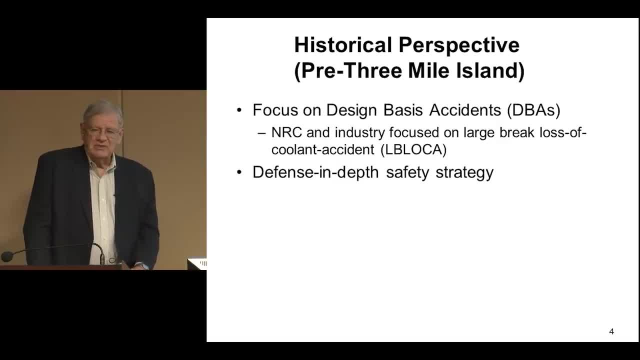 rely on any one system. So we always had a rule: back when licensees had to analyze the safety of their plants, they had to do a thing called the worst single active failure, And what we made them assume is: not only did you get the accident, but the most critical. safety system that was designed to protect against it failed when it was called upon, So there was a lot of redundancy. So if you had a pump that had to come on to push water into the core, you didn't have one pump, You had two. 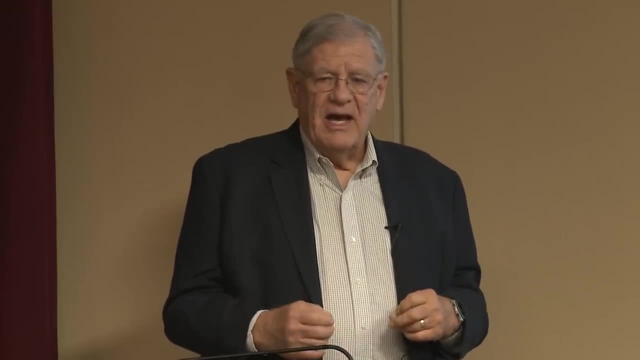 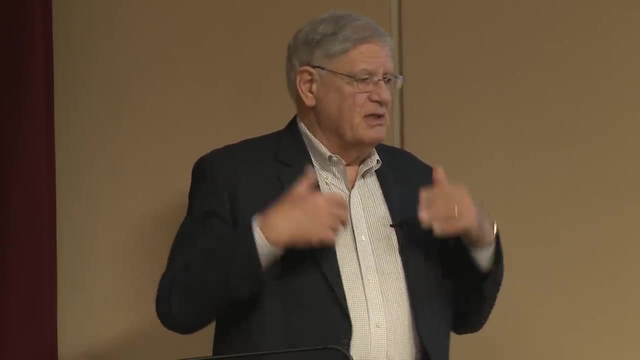 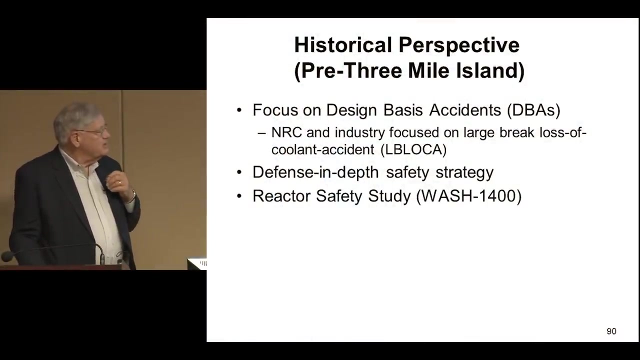 And they had to have separate electrical trains. They had to be diverse. It couldn't even be from the same manufacturer, because there may be a common mode failure. So there was a lot of that thinking going on And at the same time the NRC started what was called the Reactor Safety Study. 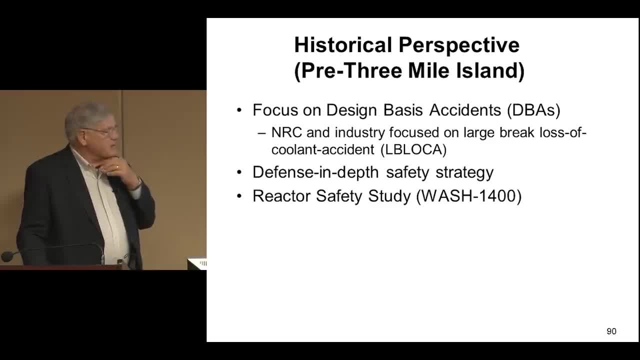 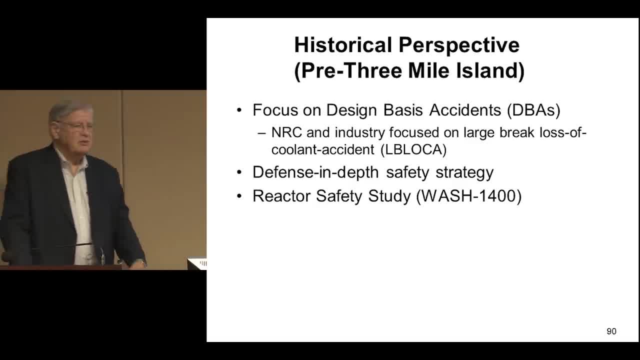 He was a professor at MIT. He was a professor at MIT and had a number of experts in probabilistic risk assessment, which was still kind of a new thing then. And what they did is they did a study to show what are the risks from nuclear power. 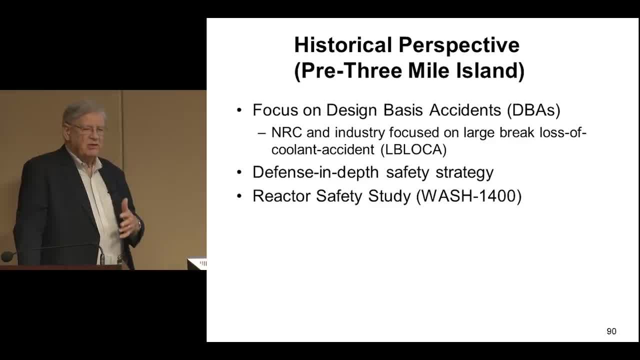 If I have a reactor, what are the failures from a probabilistic standpoint that are going to cause a reactor melt? And lo and behold what they came up with. What they came up with was that this large break loco that we were designing these plants. 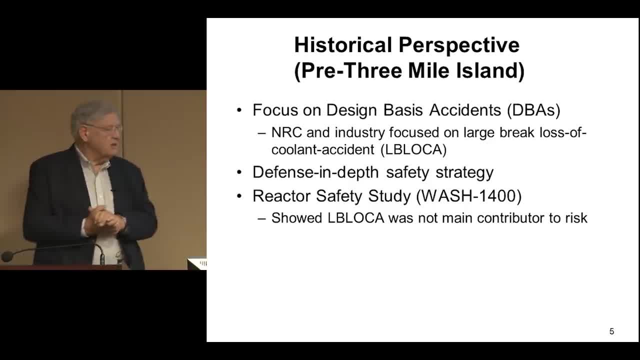 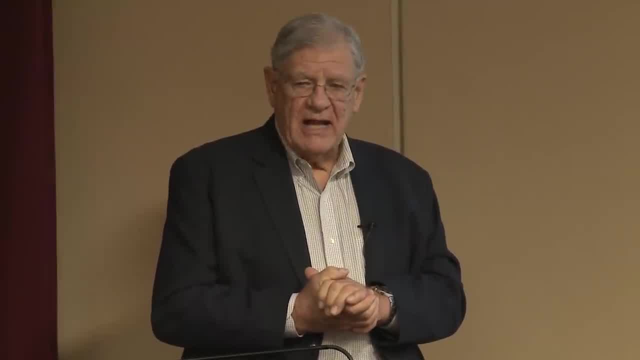 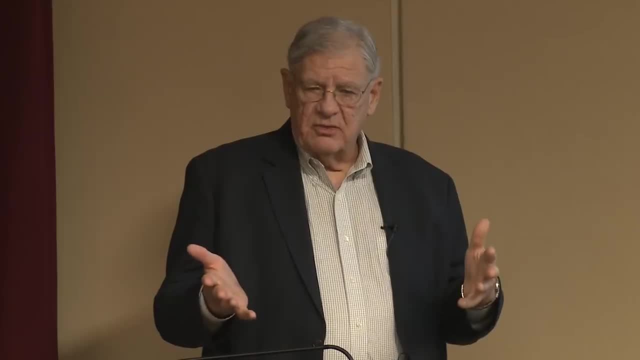 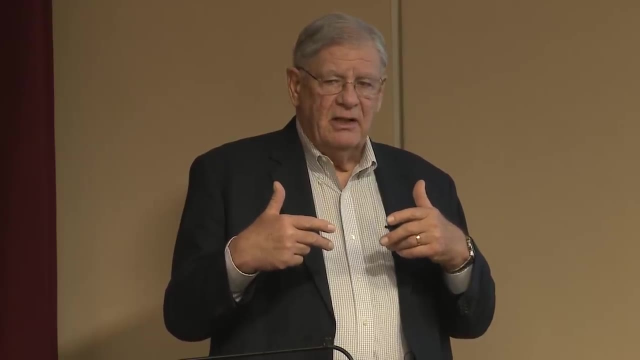 to and spending all these millions of dollars on testing was not the main contributor to risk, It was other things. It was called a station blackout And that is where you assume that you lose the grid, the transmission lines, because nuclear plants require electricity to keep running even though they're shut down. And so when they're shut down, energy from the grid comes in through transmission lines to the plant to keep pumps and everything running. You assume that they lose the off-site power. and then you also assume that the diesel generators that are designed to start up and supply power to keep the pumps and everything going to. 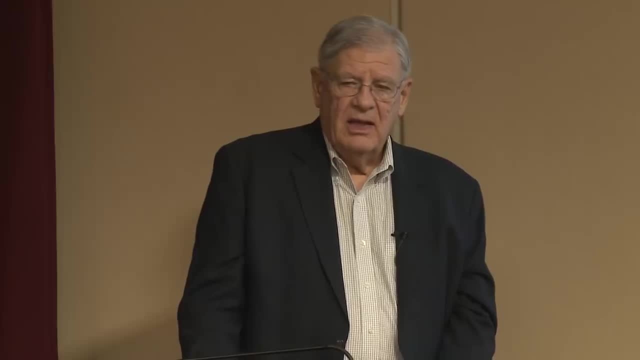 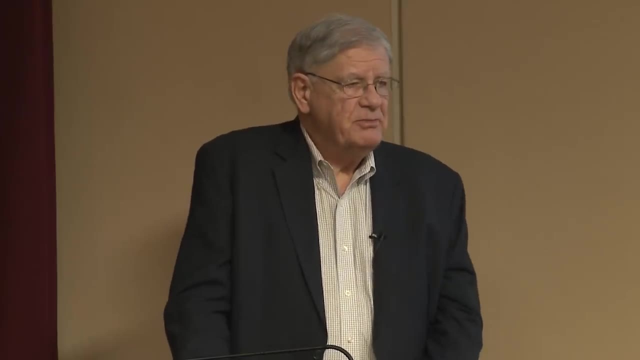 put water through the core, you assume they fail, And so you get what we call a blackout. You lose all electricity. OK, That is the problem, And that turned out to be a much higher contributor to the risk of a meltdown than this large. 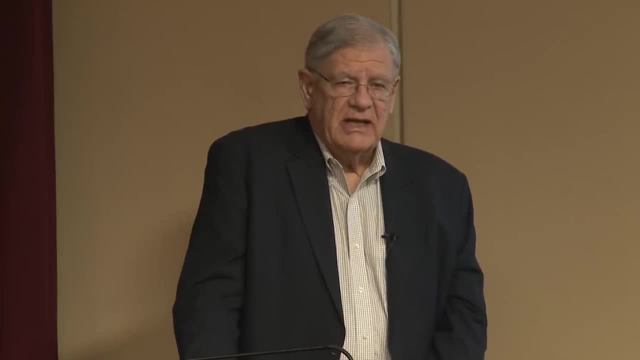 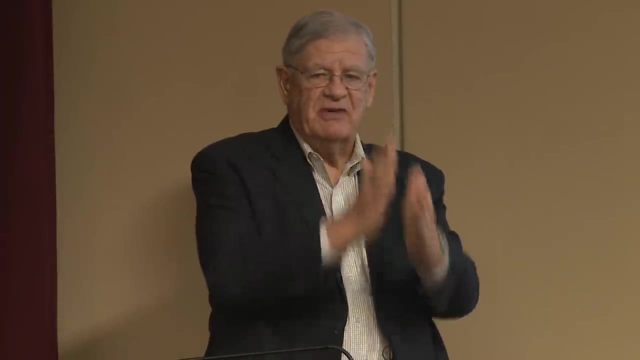 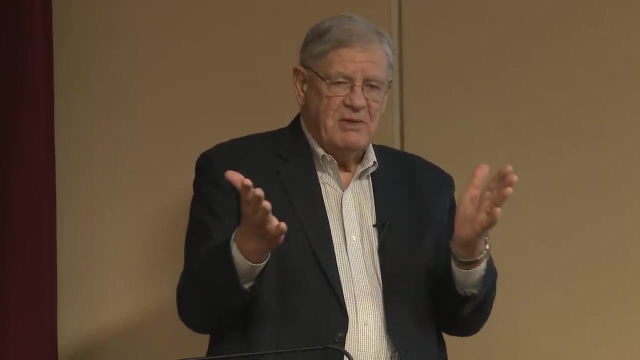 break loco, Small break, loss of coolant, accidents- not this stylized break that somebody you know. pipes don't break by just severing like that. OK, If a pipe's going to break, it's probably going to either corrode or it may fish mouth. 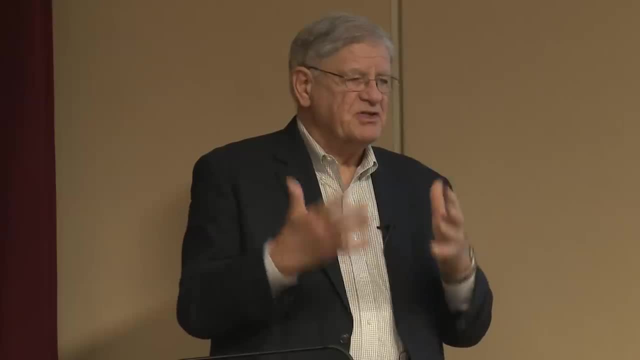 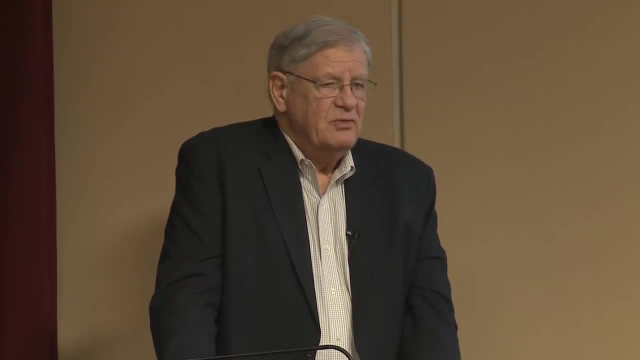 but it's not going to be a double-ended break. It's going to be a different kind. It's going to be a smaller area. You won't lose as much water. The bottom line is: what we learned from that study at that time was that this large break. 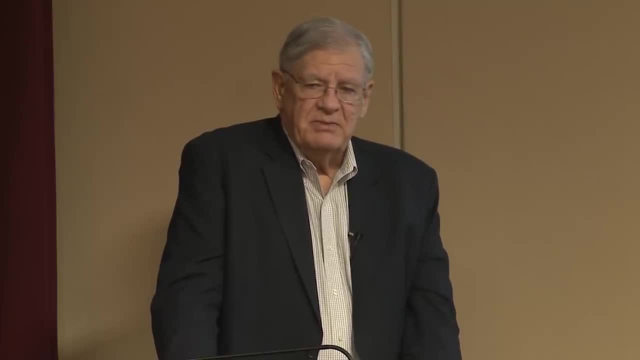 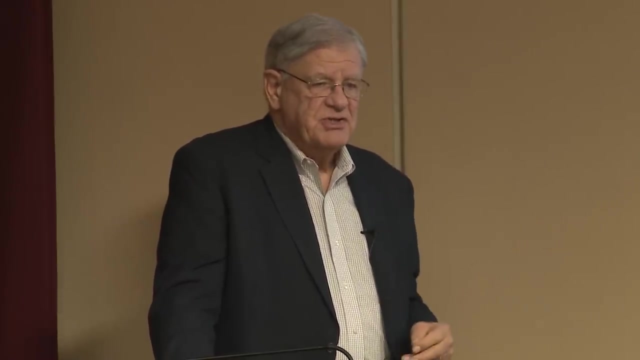 loco that we were studying was not likely to be the accident that was going to get us OK from a risk standpoint. It was going to be a small break accident. a small pipe is going to break and systems are going to fail, or we're going to have a loss of electricity and our diesels won't. 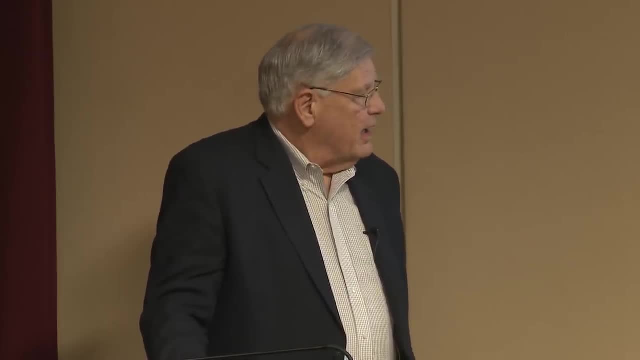 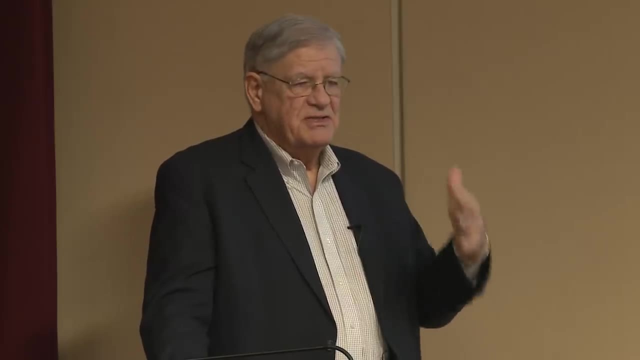 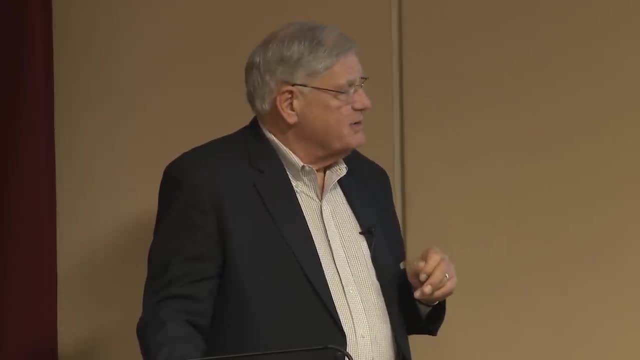 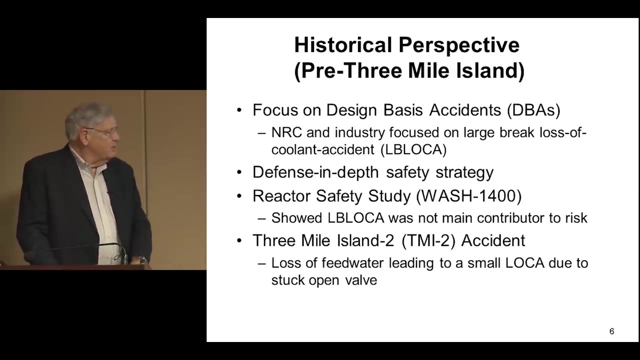 in the industry focusing on this large break accident. And lo and behold, Three Mile Island happens. And what caused that? Well, that was a loss of feed water. This is the water that goes into the steam generators. In other words, if you remember, there's a pressurized water reactor. way it works is the water is circulated through the core, it's heated up, but it's under pressure, so it doesn't boil, okay, but it gets very hot. that's why they keep it at very high pressure, so it can get up around 500 and some odd degree or. 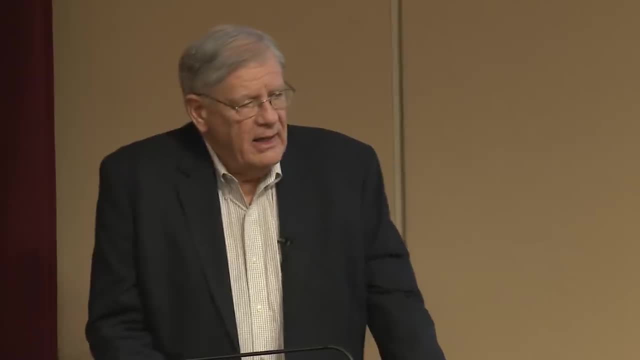 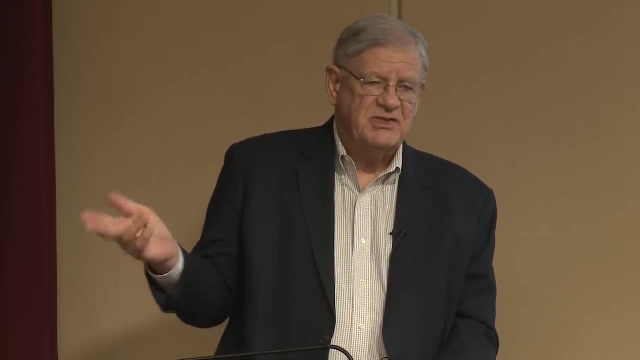 600 degrees- actually, no, 500 degrees or so. then it goes through a steam generator and as it goes to the steam generator it gives off heat to the secondary side, but the secondary sides at a lower pressure, so that water boils because it's at a lower pressure and it's that steam that is used to turn the turbine which turns the generator which generates electricity. once that steam comes out of the turbine, it's at very low pressure, but it's still steam and it's condensed. that's where they take water out of a river or a lake or whatever and they use that water to condense the steam back. 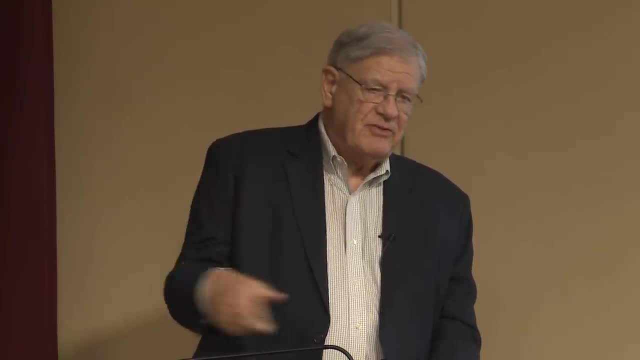 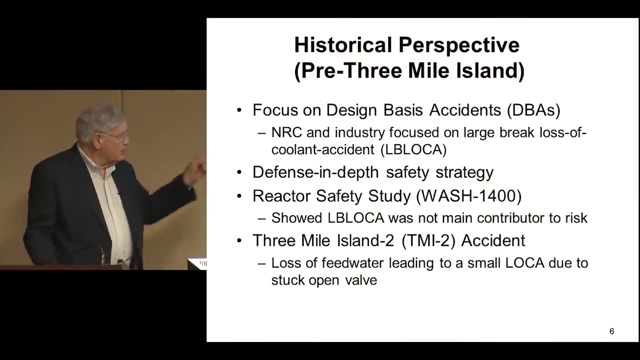 to a liquid and then it is pumped back through the steam generators. okay, and it's now it's called feed water, okay, and so that is the feed water that I'm talking about here, and what they did is they had a loss of this feed water one. 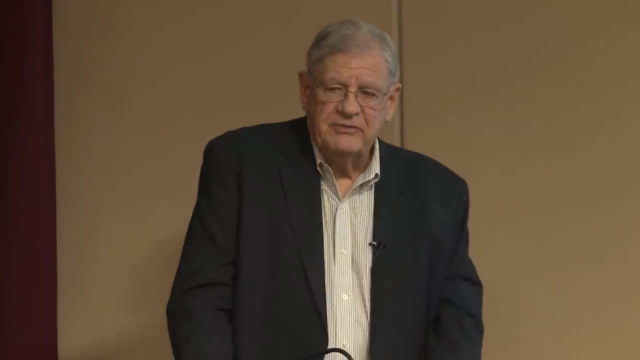 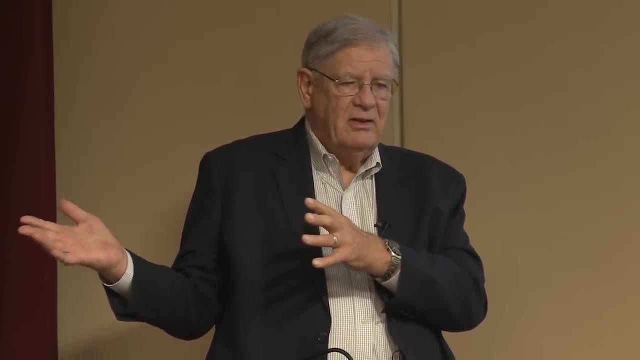 of the pumps failed. okay. and what happens if you are generating a lot of energy in a reactor and all of a sudden you can't get rid of it? okay, well, you start storing it up. you know how do you store it up when you have a reactor? 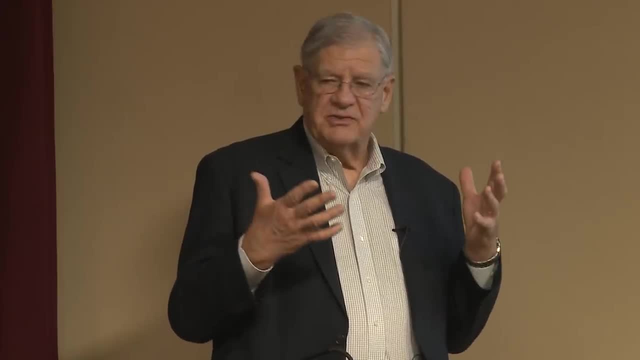 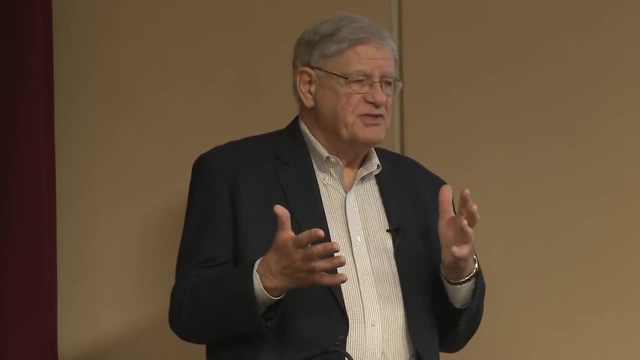 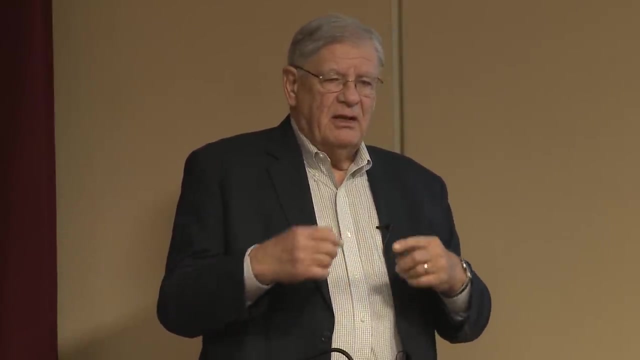 well, the water temperature starts to go up, which means the pressure goes up, just like a pressure cooker. okay, and so what happened is that, as the pressure and the primary system started going up- because it couldn't pass this, couldn't, it couldn't reject the heat through the steam generator- it reached the safety. valve set point. the point is is that they have safety valves on reactors for that very purpose, so they don't over pressurize. but they don't like them to open, because safety valves are a passive system. they open and sometimes they stick, especially if they're not used. a 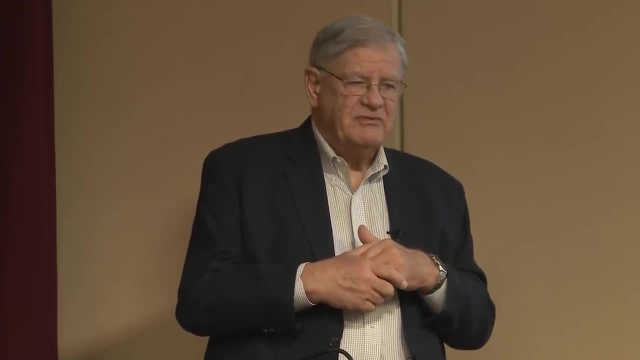 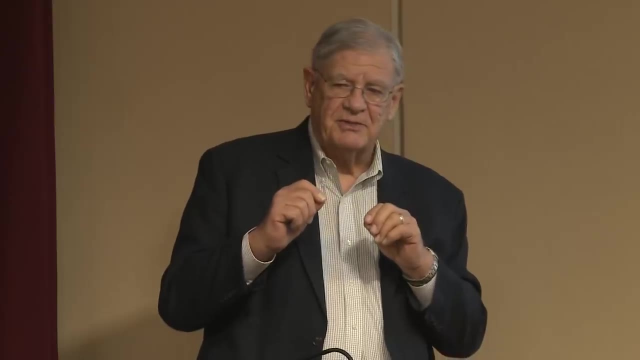 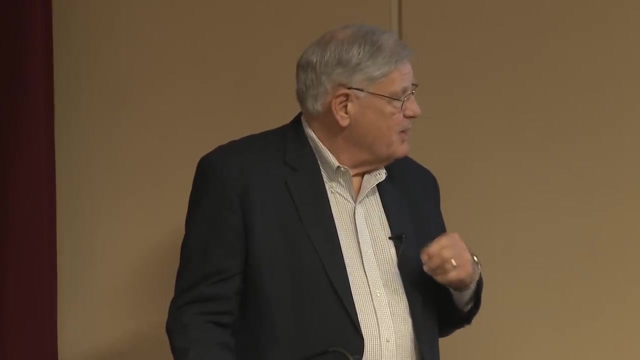 lot, and so to protect the safety valves from opening, they had a different kind of valve called a pilot operated relief valve on these reactors and this was set at a slightly lower pressure and these valves were designed to open first so they didn't challenge the safety valves. so what happened is the primary system. 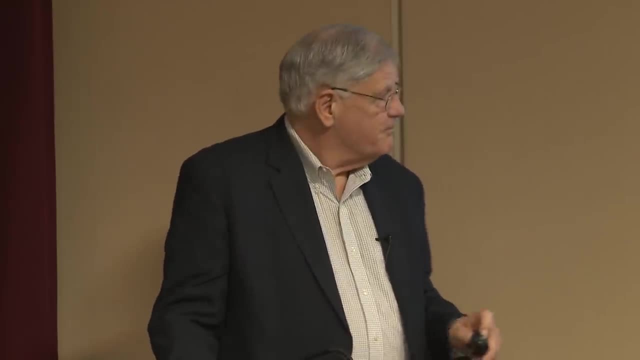 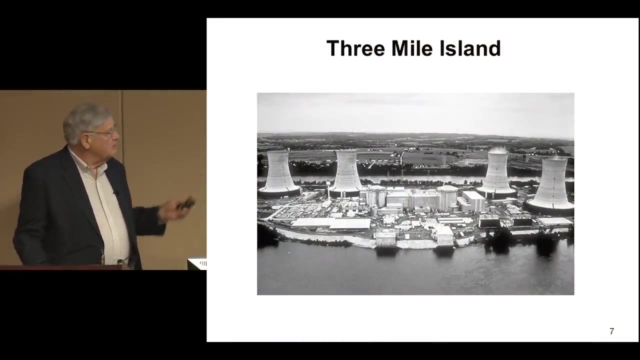 comes up and this pressure operated relief valve goes open and it's sticks okay. here's a picture of the Three Mile Island plant up in Middletown, Pennsylvania. if you ever go up to Harrisburg and go along the New Jersey, the Pennsylvania Turnpike, you can see the cooling towers. if you look off to the 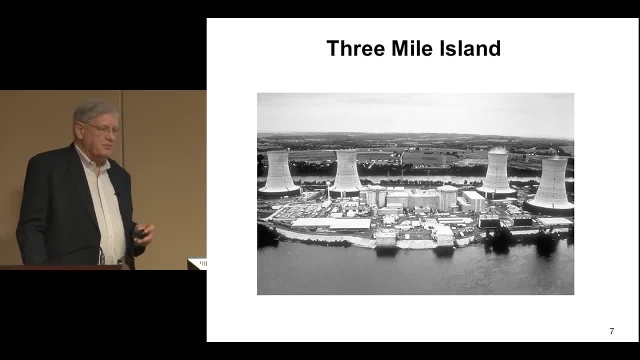 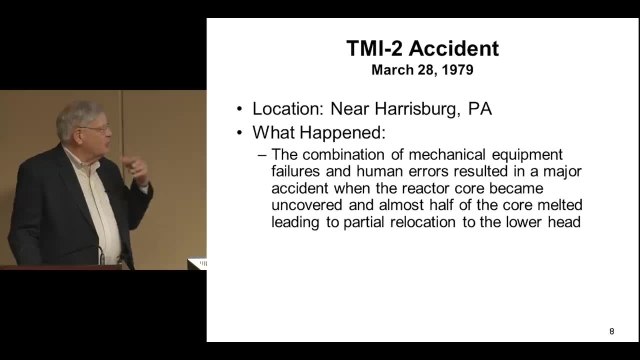 right stuck in the open position. so what happened was that and this. it's a little more complicated than that on why this feed water failed, but you know it was a combination of mechanical equipment failures and then there were human errors that were also involved, and I'll finish up a little bit. 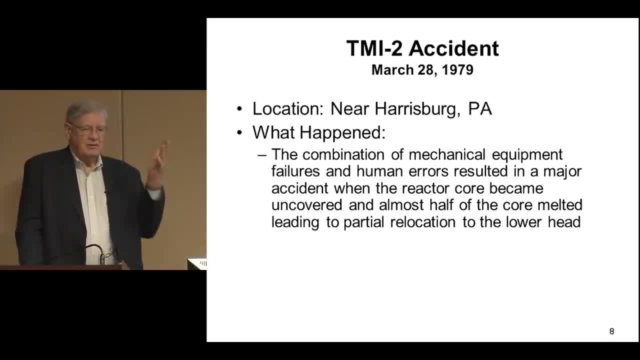 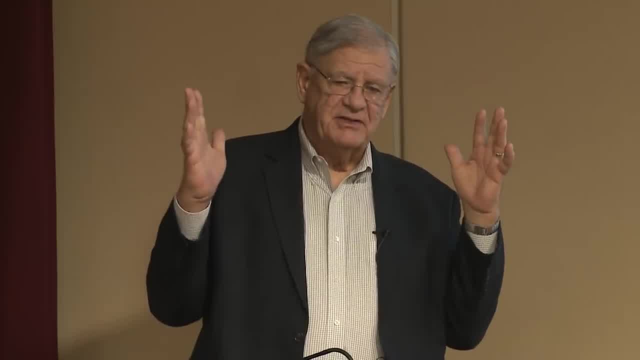 more in a scenario. what happened then was that, as the as this valve stuck open and it was in a tank called a pressurizer- there's a big tank that is connected to the primary system of the reactor, and what they do is they actually that's how they keep the pressure up very high. 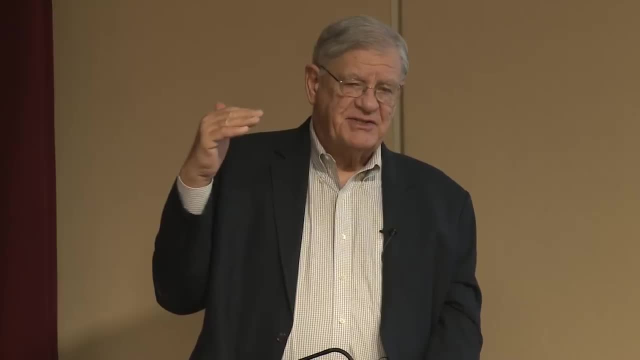 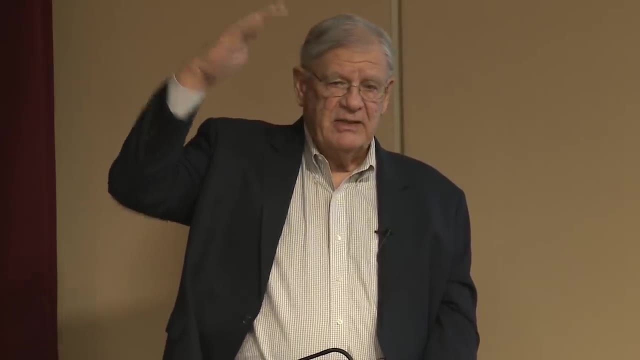 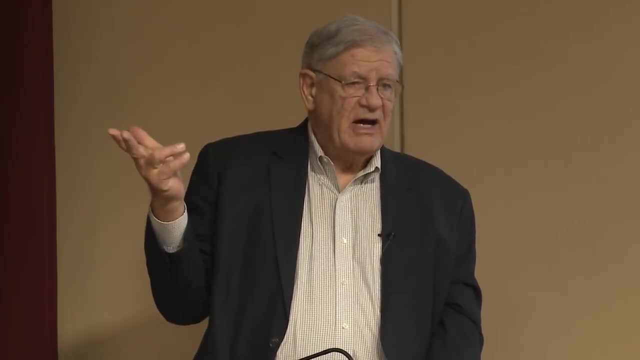 they actually have heaters in it. it pressurizes the system so the water won't boil, and the way they tell and it's up high, so the way they tell the system is full, is they have a level gauge in there. and what happened is this PORV. this valve opened up and all of a sudden started letting water out from the. 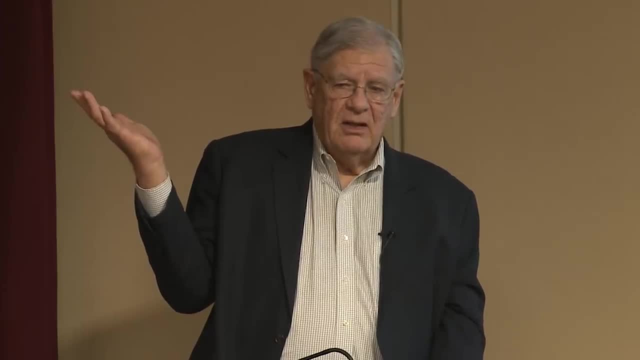 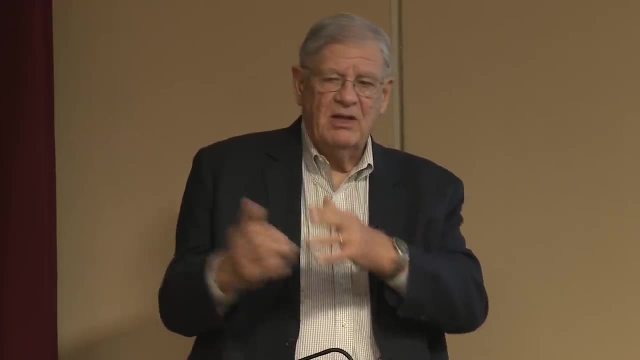 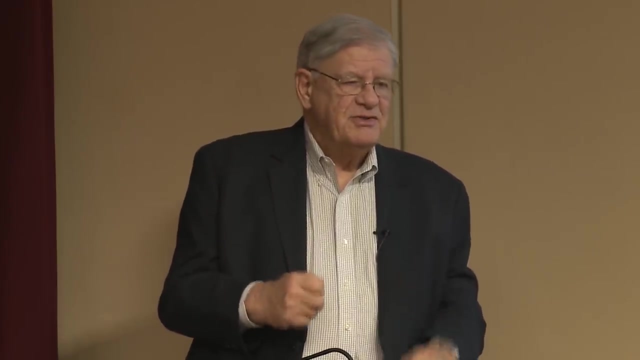 primary system. who's losing water was a small break, okay. however, the water is now, because that's the, that's the low pressure point. now, where this hole is, it's bringing water up through the primary system, okay, into this pressurizer tank. so when the operators are sitting there looking at the level gauge, they still see like the. 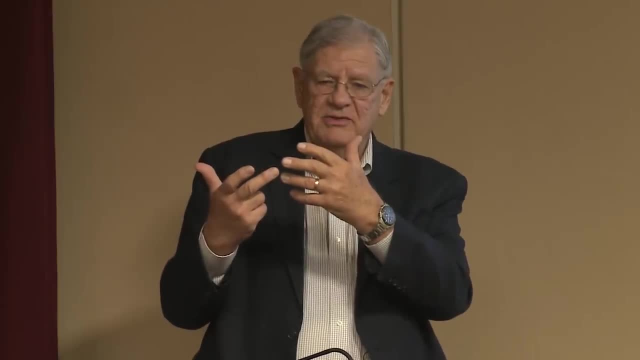 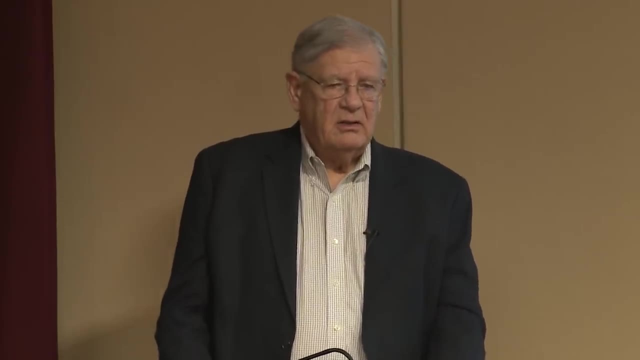 tank is full because water is being sucked up into it, okay, from the primary system, because it's going out the hole, because that's the low pressure point. so they're looking and they're going. oh you know, they didn't know the valve was stuck open. because they looked and they said gee. 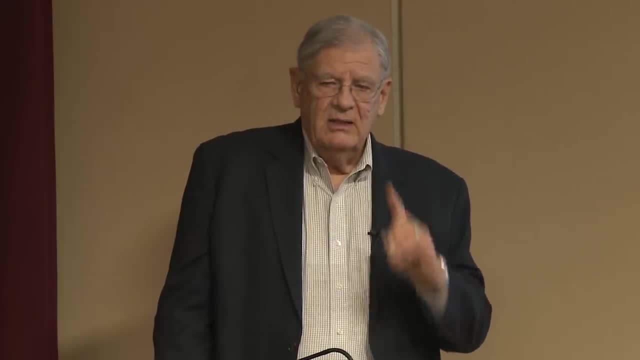 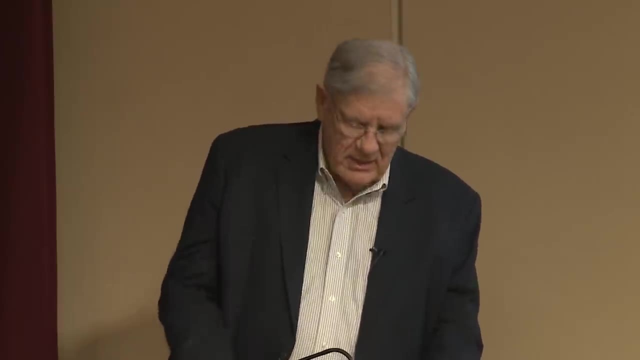 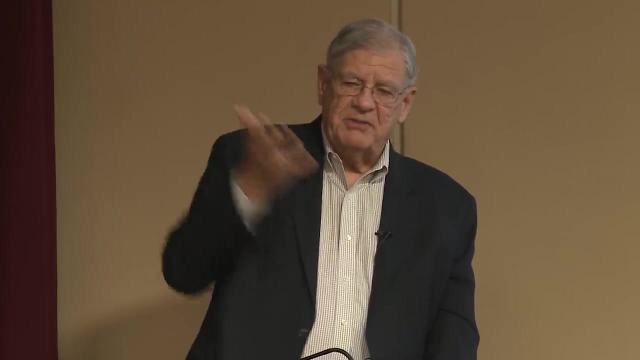 we have a level in our pressurizer. what they didn't look at was the primary system pressure, which was coming down. okay, and the water is at about 523 degrees or so. the primary system pressure is coming down because you're losing energy through the hole. okay, what happens when that pressure comes down to? 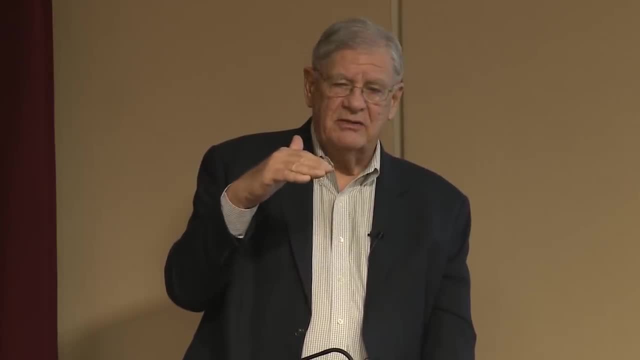 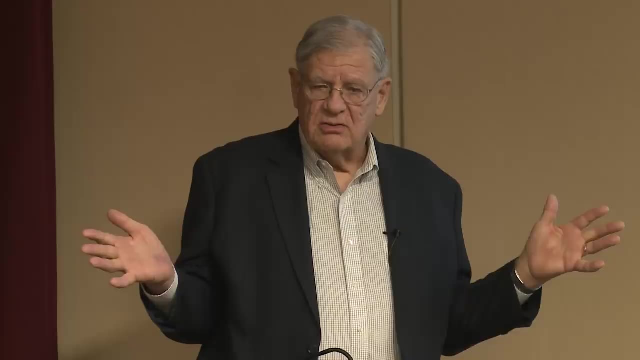 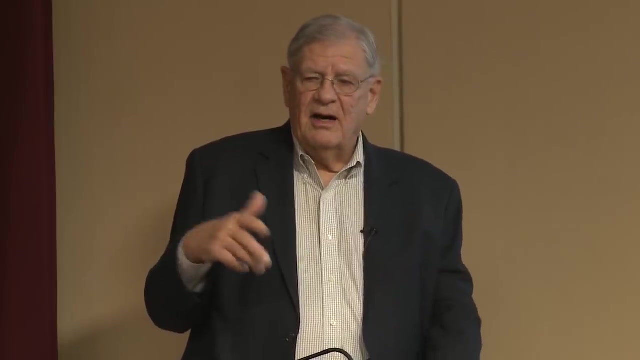 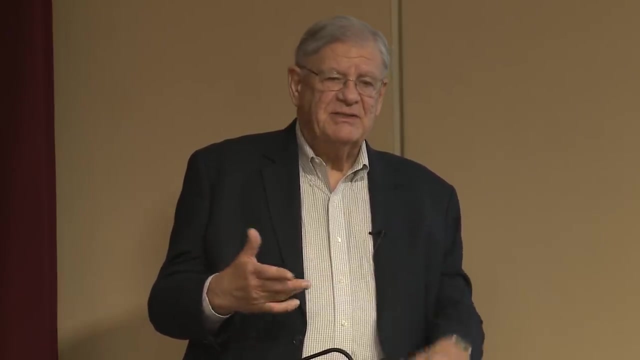 the saturation point at 523 degrees, that water boils, okay. and so all of a sudden, you now start getting two-phase mixture- steam and water- in the primary system. okay, so that's circulating around. remember, this is a pressurized water reactor was not designed to have steam in it, and what happens is that the pumps are still running. okay. well, if you've ever run a pump and you get air in it, okay. it doesn't like that, okay. it starts to vibrate, it makes its way up the airway and the water starts to vibrate too, makes funny noises. the current fluctuates and cavitation. 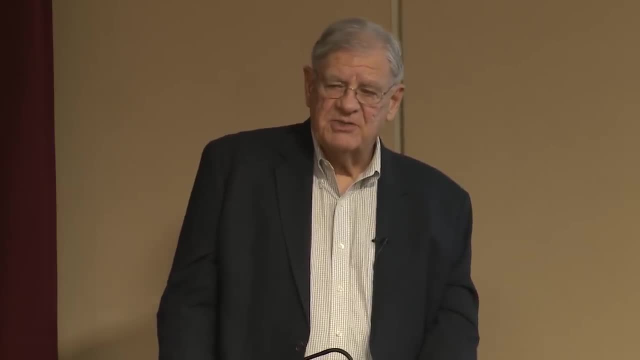 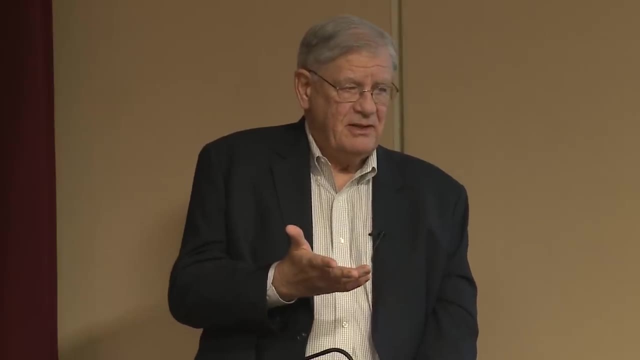 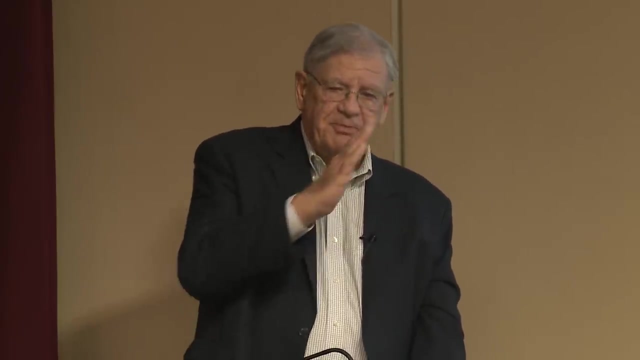 That's what happened is because they generated steam in this primary loop. the steam started to cavitate the pumps because it was being pumped through the pumps. it was a mixture of steam and water in this primary system. The operators are sitting there and they're going. hmm, they're looking at the pump. 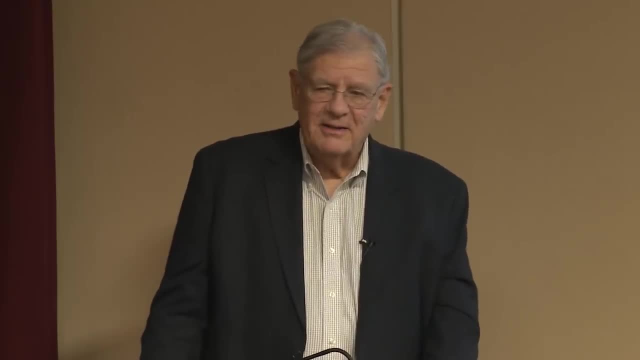 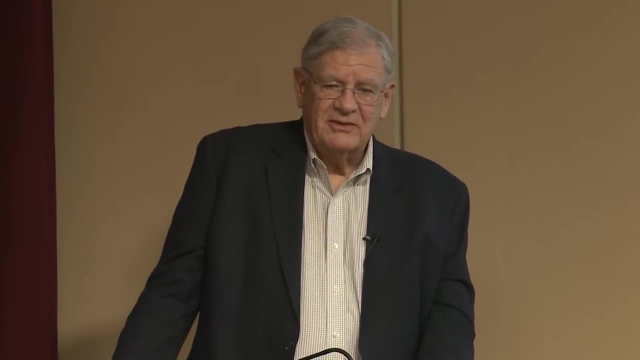 current gauge and it's doing this and they're like: these are like $4 million pumps. So these guys don't want to mess up a $4 million pump or whatever. So they're starting to worry. So they go: hey, maybe we'd better turn these pumps off. So they turn the pumps off. and what happens when you quit circulating steam and water in a mixture around a loop? Where's the steam go Up, Where's the water go? It settles down, Everything separates out. OK, So what happens? 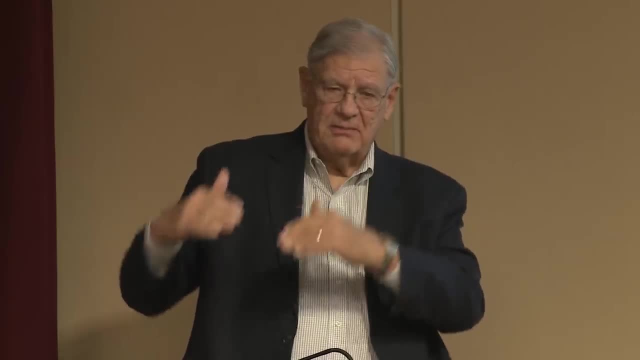 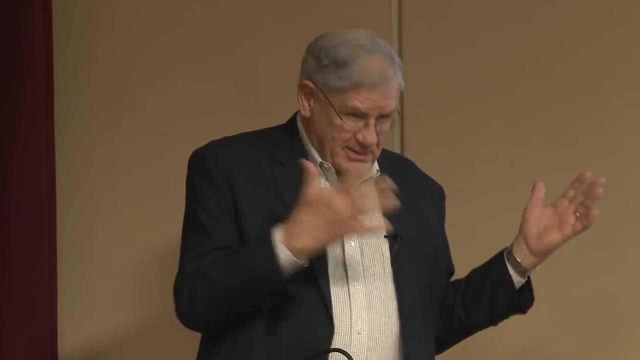 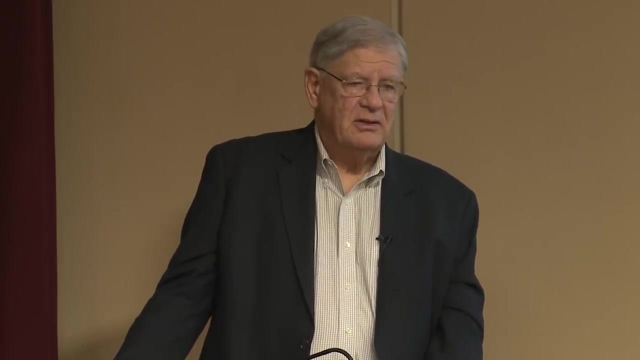 The water that's in there drops down to the bottom of the vessel and the bottom of the lower pipes and everything. The steam goes up and what happens is you uncover the core And they uncovered the core. And once you uncover the core, you cannot remove the energy in the core with just steam. The heat transfer characteristics are not enough. In order to get the right amount of heat out, the fuel temperature has to go down It's way up to get the heat transfer. Now you've got to remember the reactor is shut down. The operator shut the reactor down, OK, But you're saying: well, where's this heat coming from? Well, reactors have a thing called the K-heat, and that is that once you shut a reactor down, you stop the nuclear reaction. But the fission products that were generated during the reaction. those fission products also are radioactive And they decay. And they decay with certain different half-lives, OK. And as they decay they give off energy. So when you shut a reactor down, you put the control rods in, you shut it down, OK, 7%. of the initial energy that that reactor was producing is still being produced after it's shut down And you've got to remove that energy. OK, Now that decay energy slowly decreases, Slowly decays away over time. OK, Usually takes months before. But you have to keep the fuel cool. That's the biggest concern with US reactors. It's not, you know, when the reactor's at power, It's when you shut it down. you still have to remove 7% of that power. 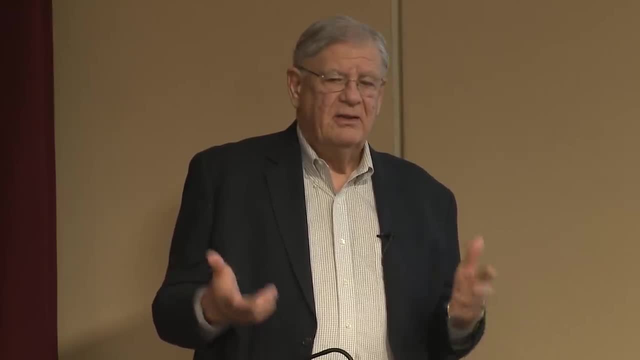 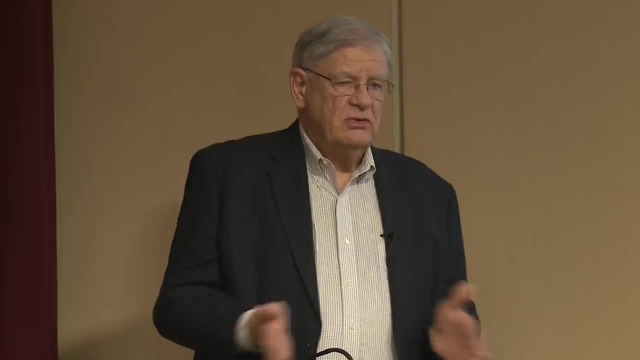 And if you're talking 1,000 megawatt plant, OK, 7% of 1,000 is still 70 megawatts of power You have to remove, So you have to have coolant always flowing past the fuel rods to keep them cool. 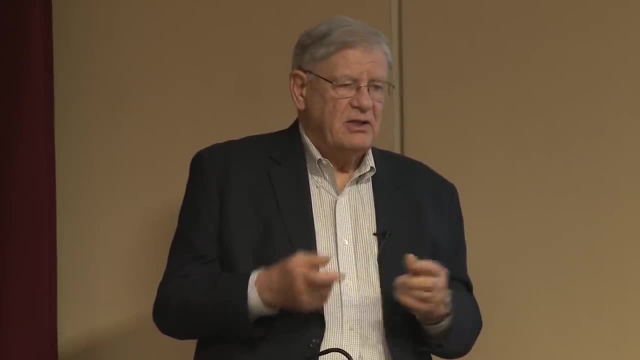 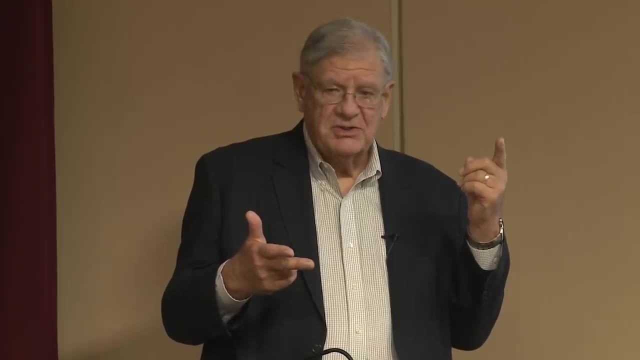 And if you have steam, go past it. you lose the cooling. OK, In order to get the right amount of heat transfer, OK, the fuel temperature has to keep going up, And it will. It'll just keep going until it melts. 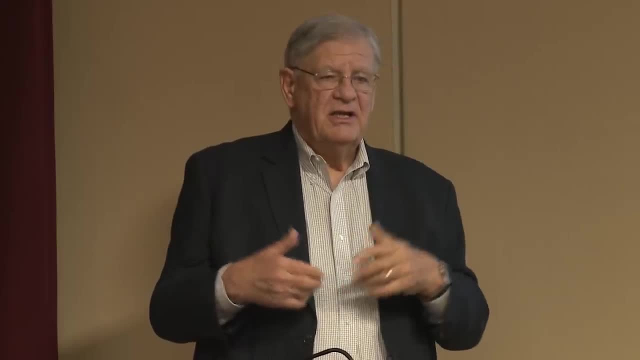 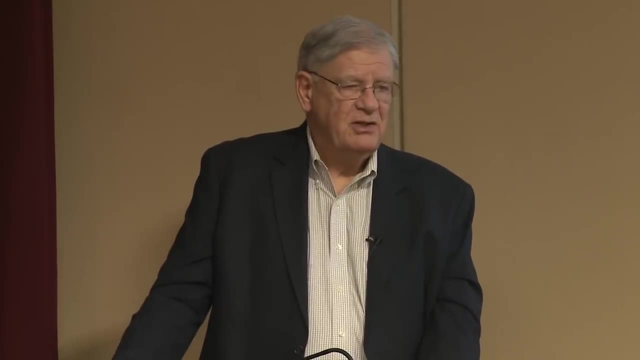 And that's what causes a core meltdown is when that fuel just keeps generating energy and the temperature will go up. That's why you hear about the temperature, The China syndrome. That's what that means. you know that the fuel OK, because it's continuing to generate. 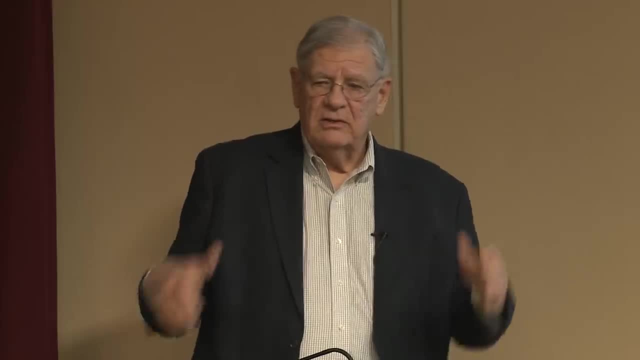 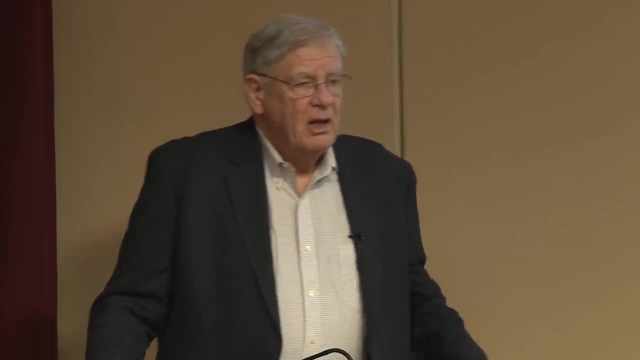 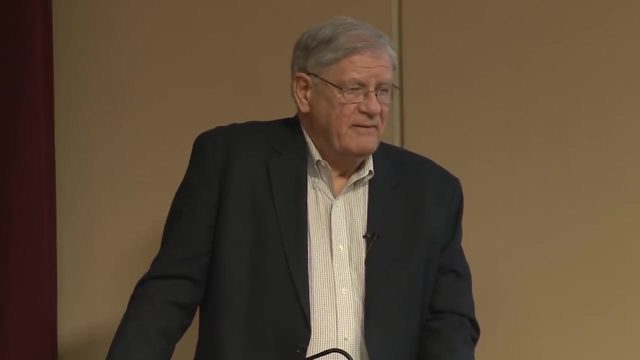 energy OK, and won't stop OK- would literally burn its way through to the center of the Earth. Once they had figured out what it was, what should they have done? What should they have done? Actually, what they should have done is tried to close that valve, OK. 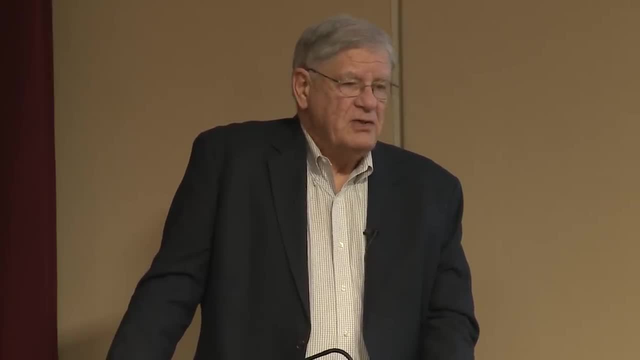 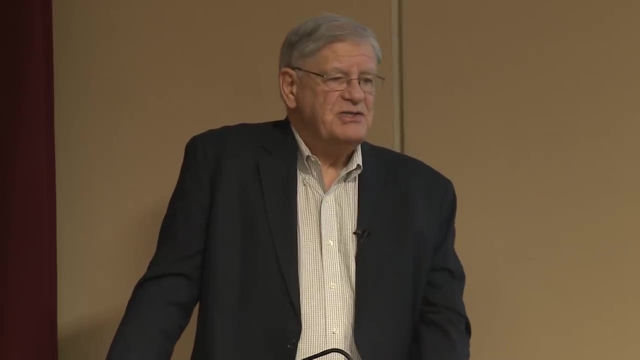 They didn't know the valve was stuck open. But even though they knew the valve was stuck open, OK, what they should have. and the other thing they did is because they thought that they had liquid, they had a full system, OK. 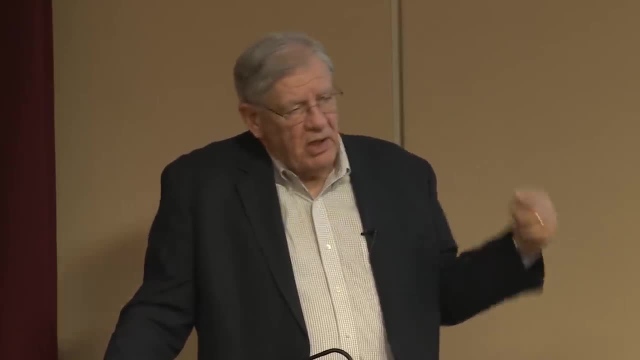 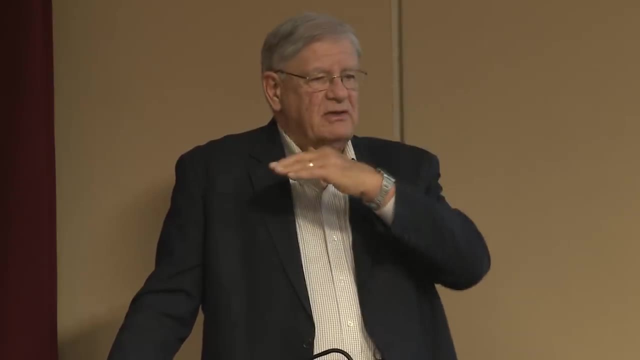 they turned off their emergency core cooling system that was starting to put water in the core because they said, hey, you know I don't have a small break here. Look, my system's full, OK. So they misinterpreted the symptoms, OK. 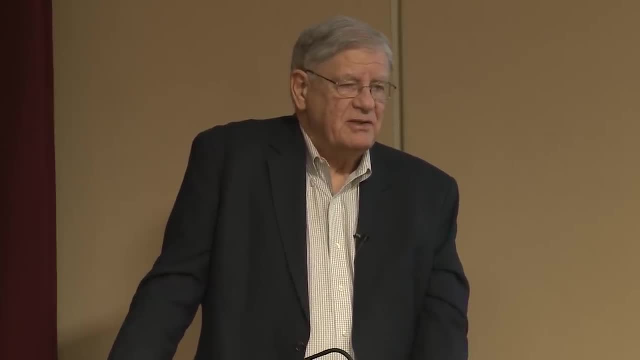 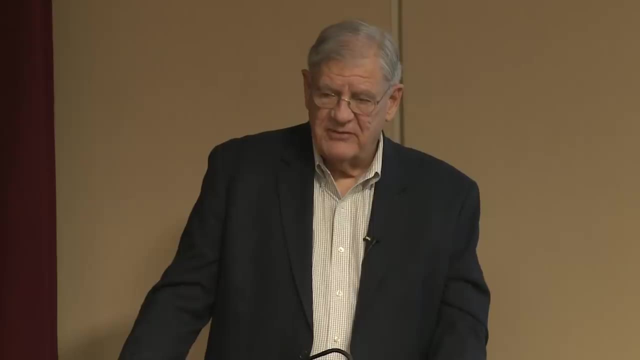 And that was one of the big lessons. That was one of the big lessons learned from this accident. OK, because all of their procedures in the control room were event-based. OK, In other words, they see stuff happening and they pull the notebook off the shelf and they 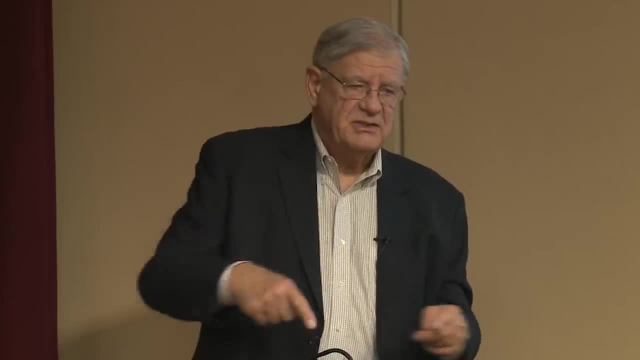 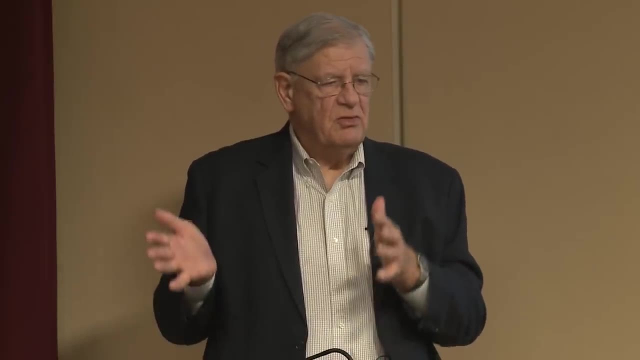 go. let me see, This is small break, loco. I do this, this and this. OK. One of the biggest things we learned from that accident was to change over their instructions to what are called symptom-based. Don't try and figure out what accident occurred, OK. 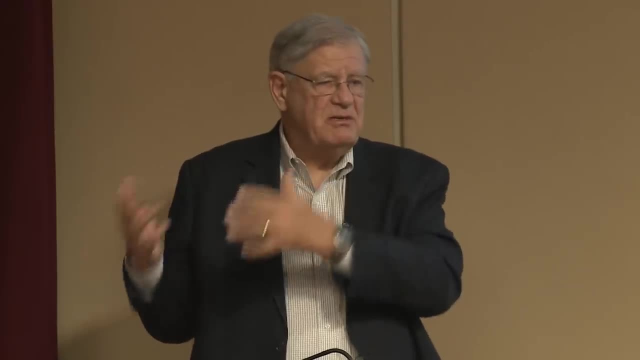 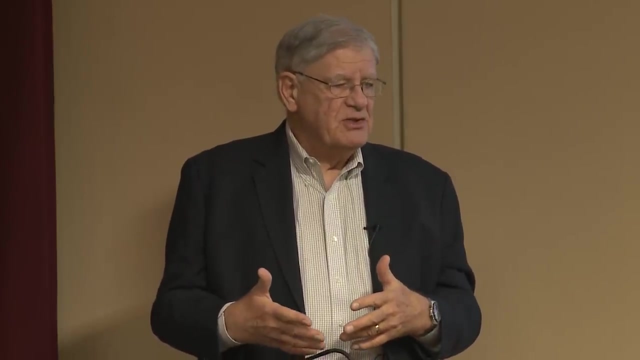 Whether it's a small break in a… Or a large break, or a steam line break, OK, or something you know, Don't… Just treat the symptoms OK. So, for example, if your primary system, if you lose the sub-cooling, OK, or the amount, 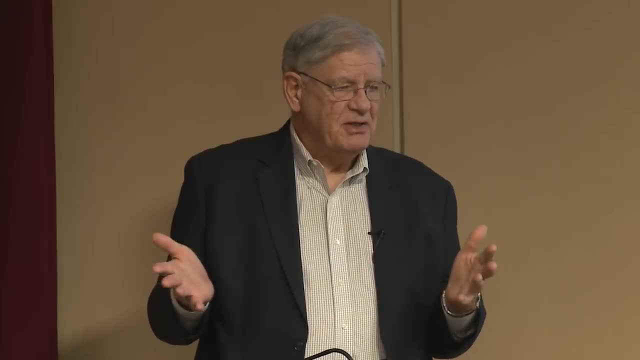 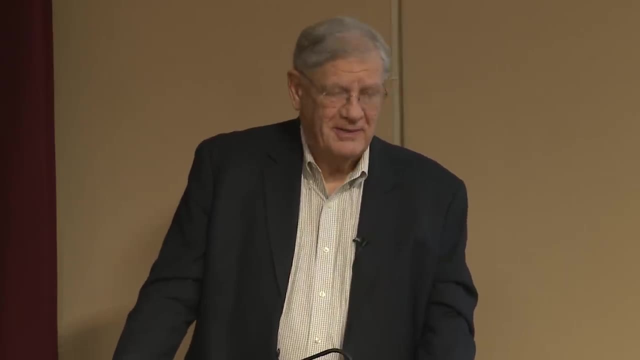 of you know. so you see that the primary system is saturated and has steam in it. OK, that's a symptom. OK, that you've got to hold. Don't worry about where the level is. OK, Put water in. 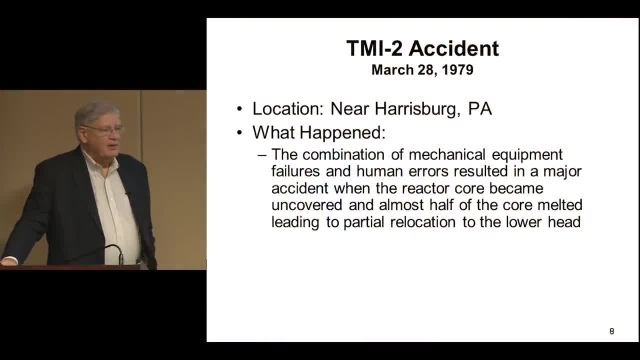 So, anyway, what happened is that they uncovered the… Uncovered the core. About half the core melted and it you know, when the core melts it starts to slump down. The hottest part of a core is in the center. OK, 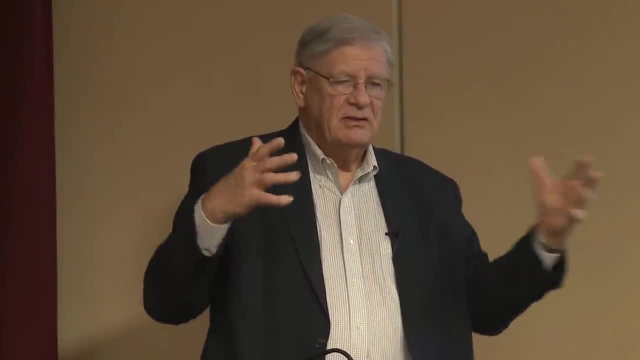 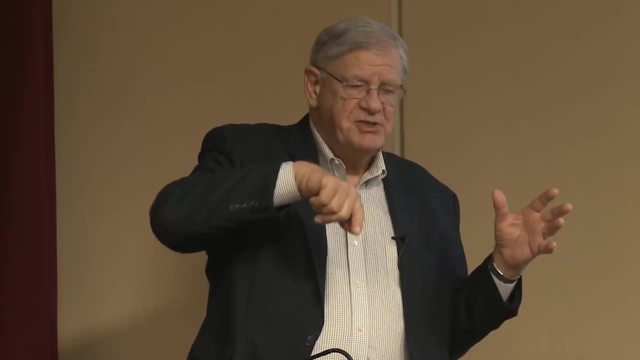 If you ever go through the math, the physics for a cylindrical core, which is the way they're designed. OK, the power profile is a cosine shape in the axial direction and well, it's part of a Bessel function. OK, 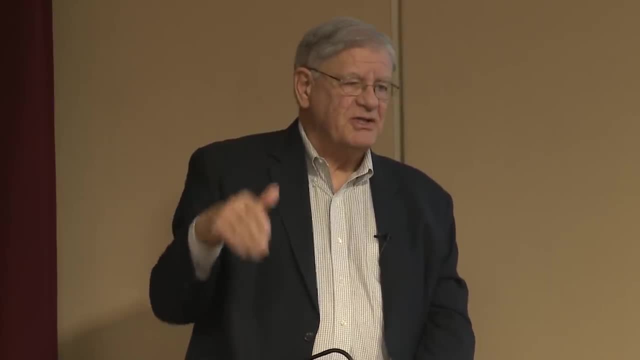 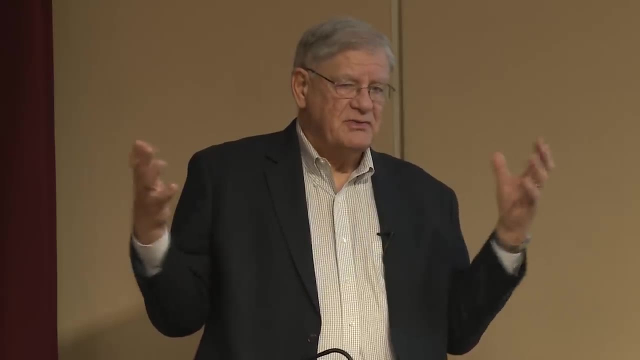 But it's typically it's almost like a cosine shape in the center, So the hottest part is right in the middle. That's the part that's going to heat up first. OK, So I used to call those like a chocolate-covered cherry. OK, 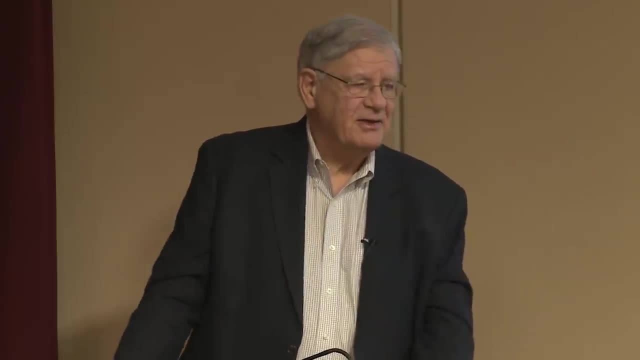 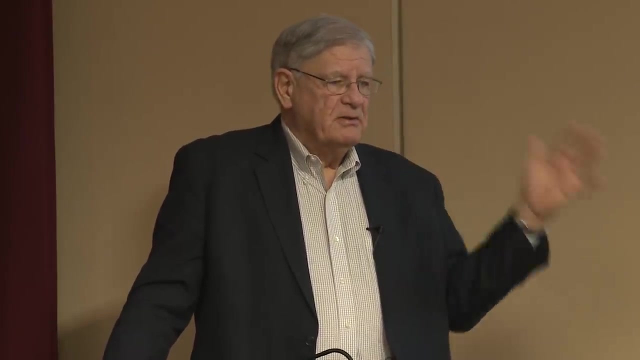 Center part's nice and soft and mushy, but the outer side's still hot, OK. And what happened is that it started to melt in the center, OK, It built up a crust on the outside, but once it reached a certain point, OK, it actually. broke through this crust and all of a sudden this molten fuel and material ran down and relocated in the bottom part of the Bessel head. OK, And now the big question we all had is: why didn't that lower head fail? Because steel melts at what? 2,500 degrees or so, and this stuff is over 3,000 degrees. Fahrenheit. There's a lot of theories. It still hasn't been conclusively shown. OK, But the theory is the best one right now is that there was a layer of water that got trapped in there and, even though it may have generated steam, it was enough to insulate the lower. head from the melt, actually heating it up to the point where it failed. So fortunately the lower head didn't fail, But the consequence is that about 144,000 people were evacuated. It scared the bejesus out of a lot of people. 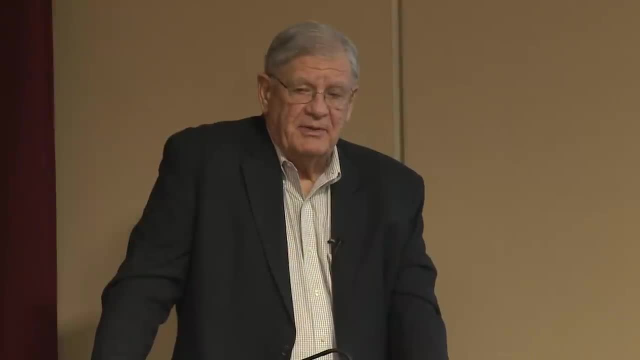 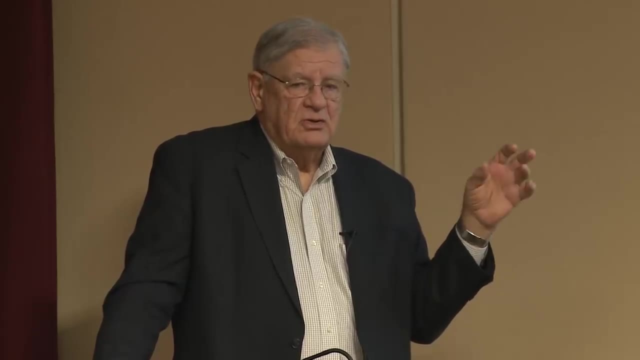 It was a public relations nightmare. The other thing that happens in these plants, by the way, is that the fuel is clad in a material called zirconium- OK, It's called zircaloy- And what happens is when steam reacts with zirconium at very high temperature, it generates. 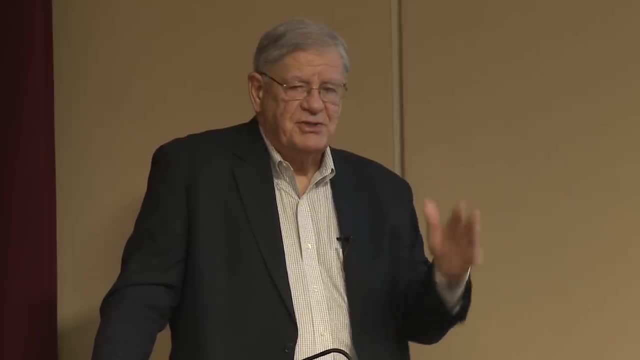 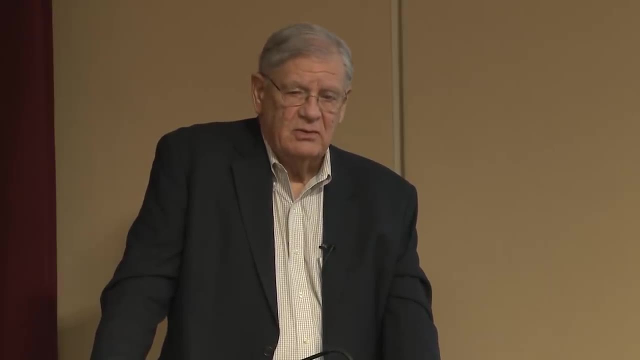 hydrogen. OK, You get zirconium oxide and hydrogen And the hydrogen, as you know, at about, I think, 8% will detonate, I'm sorry, will deflagrate, which means it'll burn, And at about 12% or 13% it detonates. 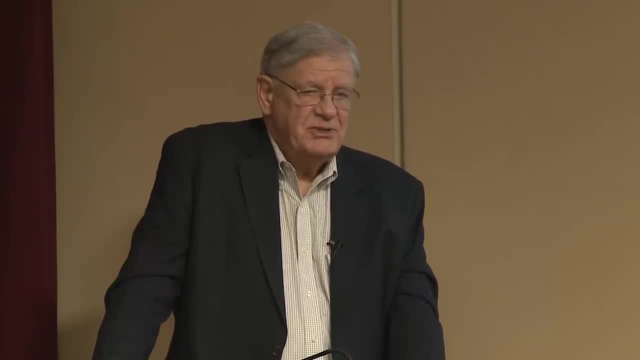 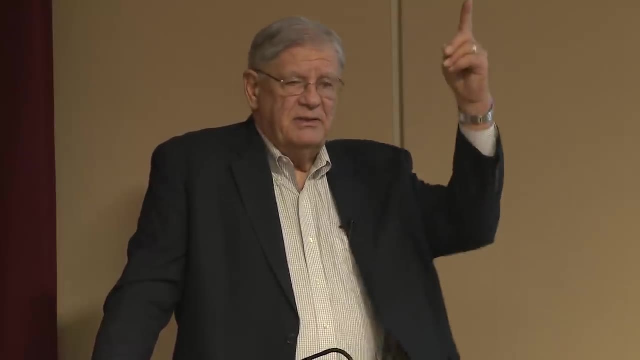 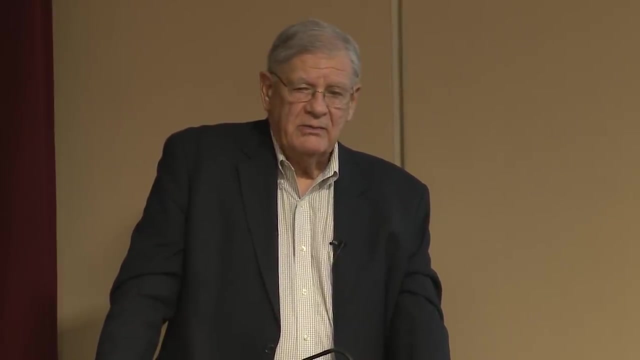 Which means you've got an explosion And this hydrogen that was being generated in the core from this zirconium water reaction actually went out into the upper part of the containment building, which is that big concrete building that you saw there, And in one point there was actually we saw a big pressure spike, which means there was 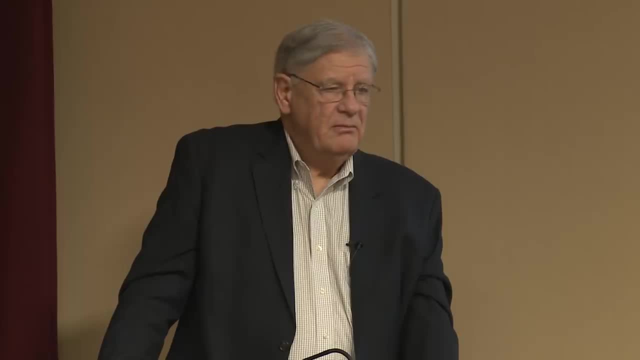 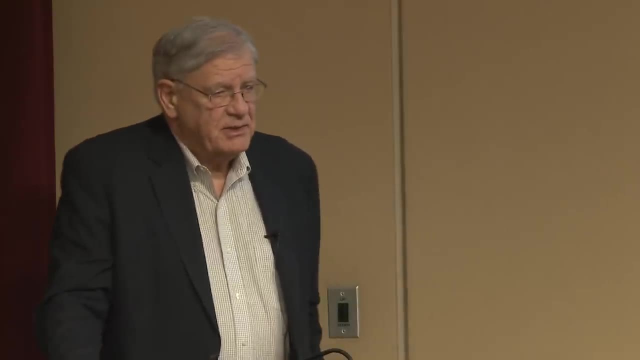 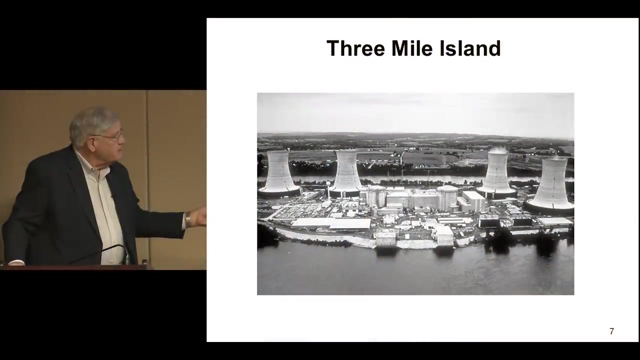 a detonation. It did explode. This was coming through that open valve, Yes, But yeah, this was a nasty accident. OK, The best thing I can say is that let me go back. These are the containment buildings. these big, these things are very, very thick. 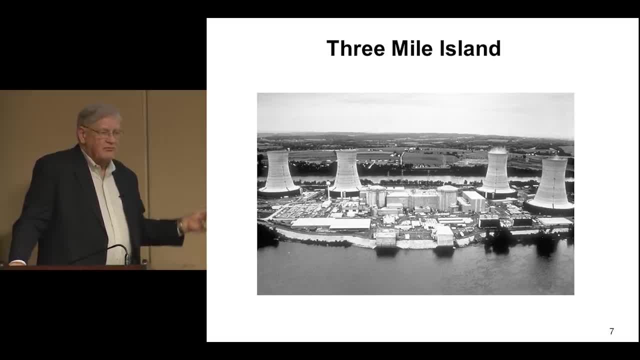 The walls are like about eight feet of concrete, OK, with reinforcing rod in there. They're designed to hold. they're designed pressure for the ASME boiler and pressure vessel codes around 50 psi. What that really means is that their ultimate pressure, when they really will break, is 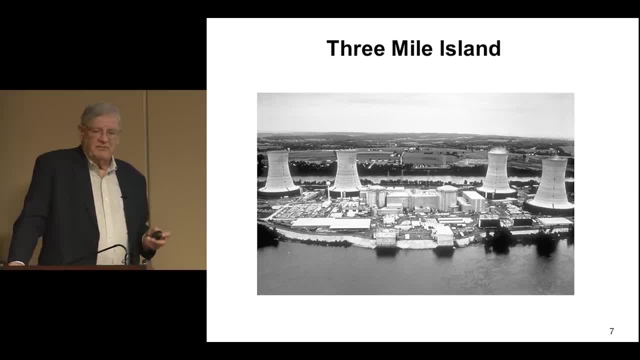 probably about 120 psi. OK, That's a fairly high pressure. OK, If you remember, you take your radiator cap off your car and you see it go spewing out. that's only 15 pounds, so But anyway, these containment buildings are what really saved everybody, because they 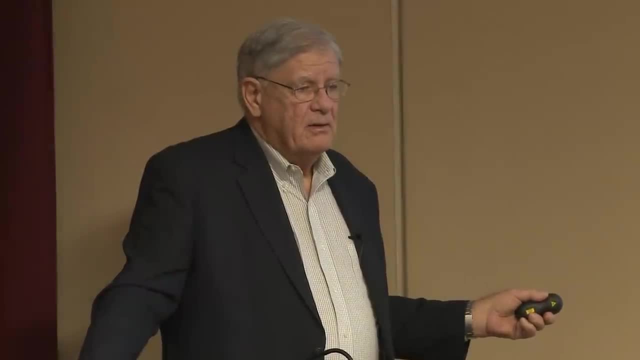 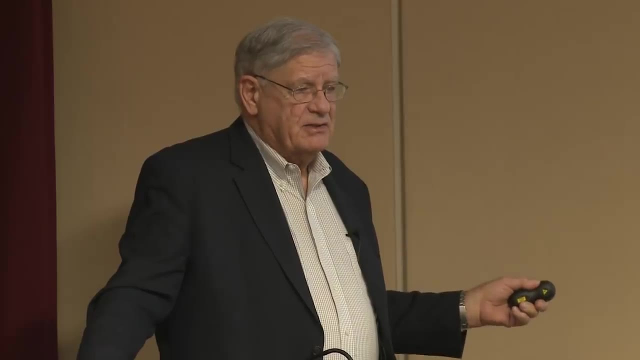 didn't fail. Yeah, Now there was a minor release of radioactivity. where did that come from? That probably came out. they have vents, they have stacks- OK, Where they have to do normal- Through the containment buildings, Yeah, OK. 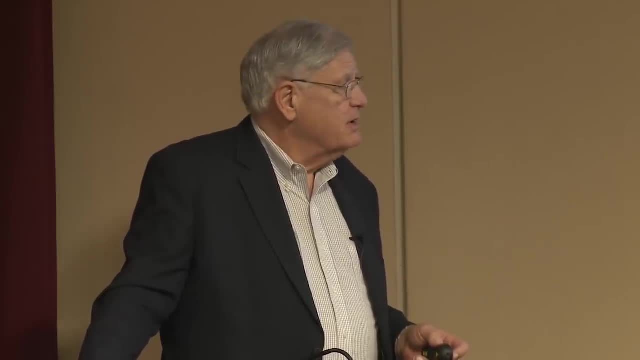 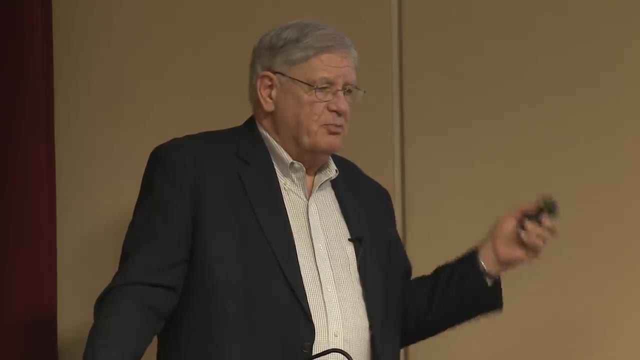 Because there are. there have to be penetrations going through the containment buildings And there's been a lot of controversy on exactly how much was released and everything You know, and there were reports of, you know, giant dandelions five feet in diameter and 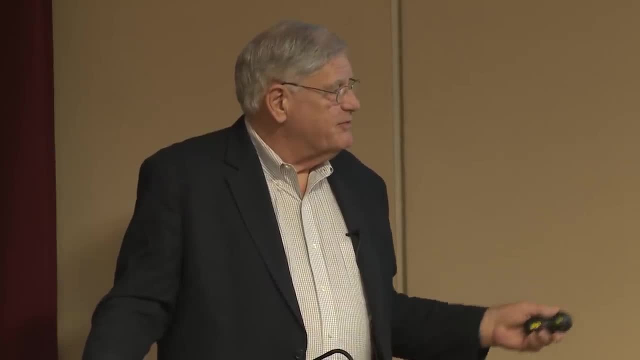 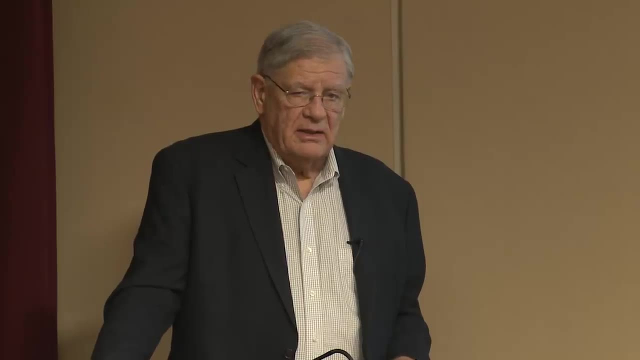 all sorts of stuff there. I was up there right after that. So anyway, this was a defining moment for the nuclear industry and the NRC. very much for the people up there. Yeah, I can't remember the company actually that ran it at the time, but pretty much every. 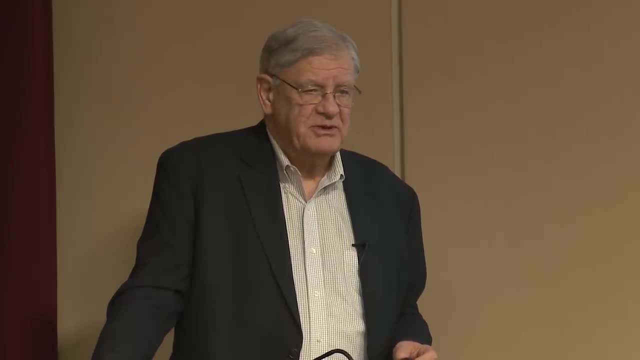 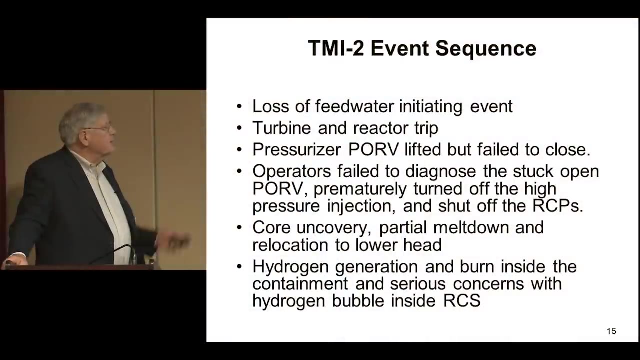 time you know you get a nuclear accident and you know pretty much everybody's you know in the management level is going to get fired. OK, and they did. They all left Anyway, but it was a loss of feed water. initiating event. 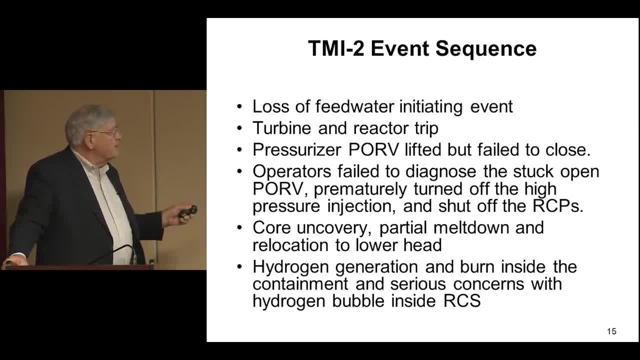 They had a reactor and a turbine trip Their pressurizer pilot-operated leaf valve lifted, failed to close. The operators failed to diagnose the stuck-open valve. They prematurely turned off the high-pressure injection. which is war. It's the water, that's the safety system. And they turned off the reactor cooling pumps. This caused a core recovery, partial meltdown and a lot of the molten core relocated to the lower head. They had a hydrogen generation and then a burn inside the containment And there were serious concerns about a hydrogen bubble inside the reactor cooling system itself. 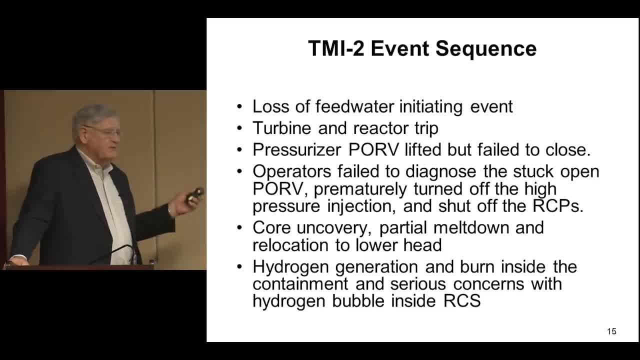 In other words, there was worried about – this was kind of a false concern, Because – In order for hydrogen to burn you have to have air, And there was no air in the vessel, But people were worried about this – about a hydrogen bubble in the top head of the reactor. 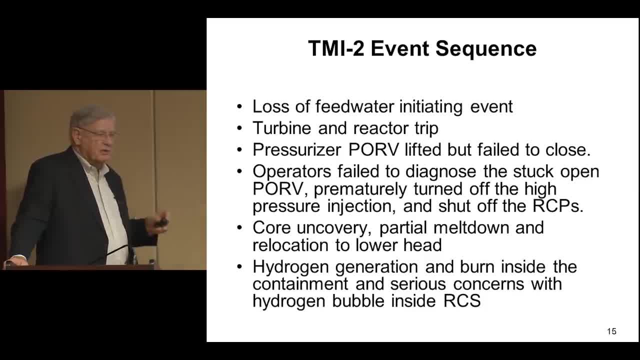 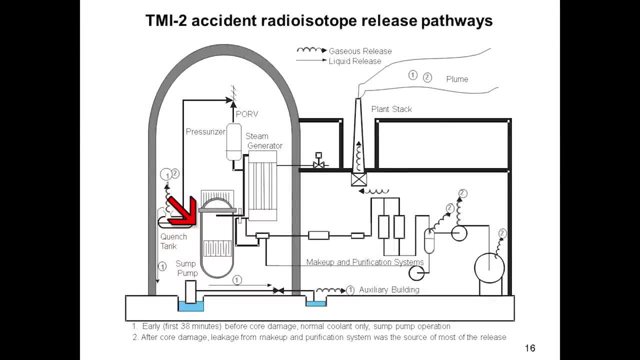 vessel actually, you know, thinking it could explode or something, And there was a lot of worry about that. Here's the reactor, Here's the core. OK, The way this works real, simply, is that you pump water in to the reactor. OK. 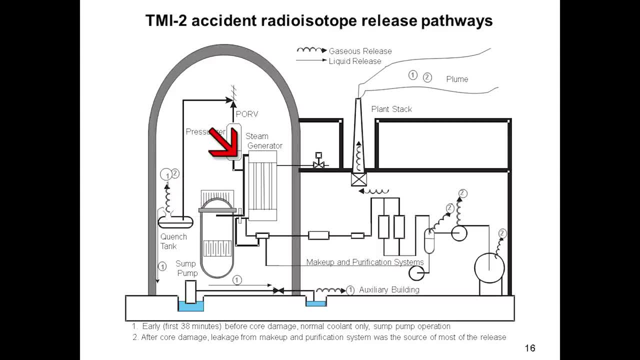 It goes through. the core Comes up, Comes up here. This hot water goes into a steam generator, Goes down the generator, Comes out, Goes through a pump- OK. And then back into the reactor On the steam generator side. the water on the secondary side here goes through, OK. 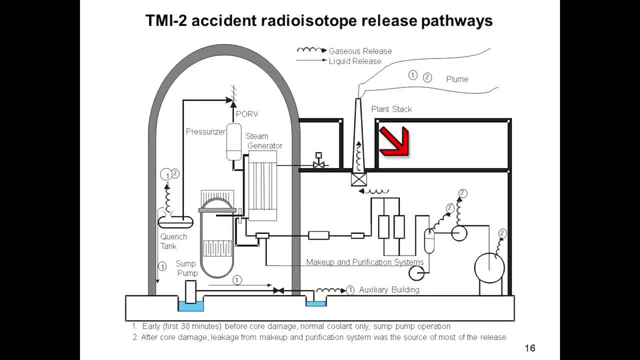 It comes down, The steam coming out goes into a turbine, Then it goes – which turns the generator, And then it comes down and it goes back into the steam generator. OK, once it's condensed. So it's a two cycle, It's a two loop. OK. 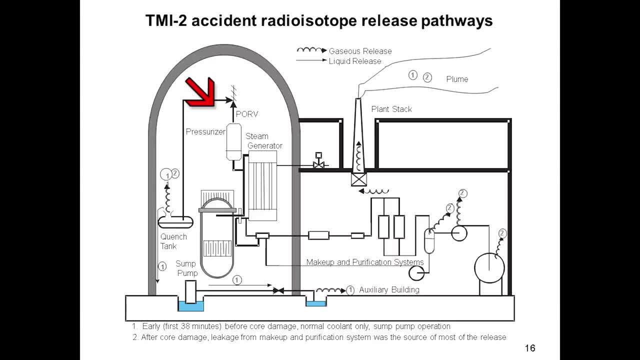 What happened here was this is – the PORV is up at the top of this tank, here this thing called a pressurizer, which is where the safety valves are also, And that valve opened and stuck open, And what happened is that, once it's stuck open, the water comes down into what's called. 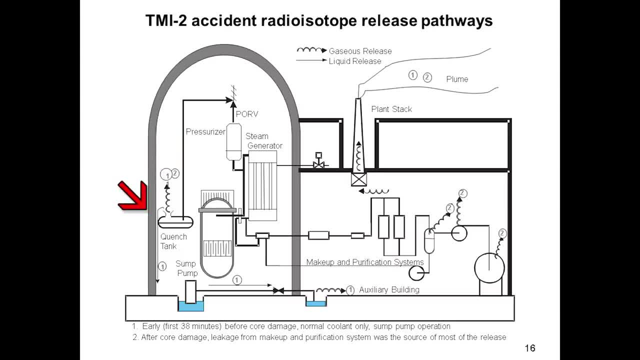 a quench tank. OK, because that's steam up there. So what they try and do is, if it does open, they want to condense the steam, So it comes down. But they – what happened is they filled up the quench tank to the point where it ruptured. 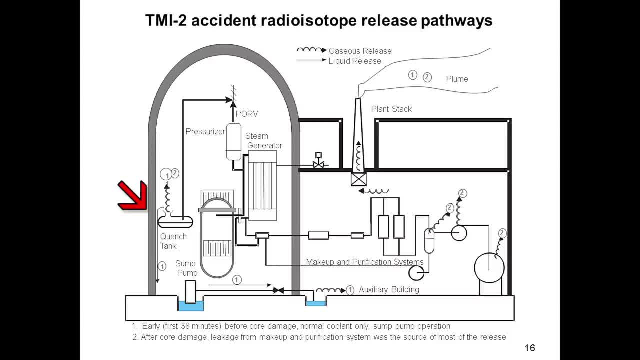 And then you can see. that's how a lot of this material, steam and everything got into this upper area of the containment. In all of this, where was the original valve that stuck? The valve that stuck open is right up here at the top of this pressurizer. 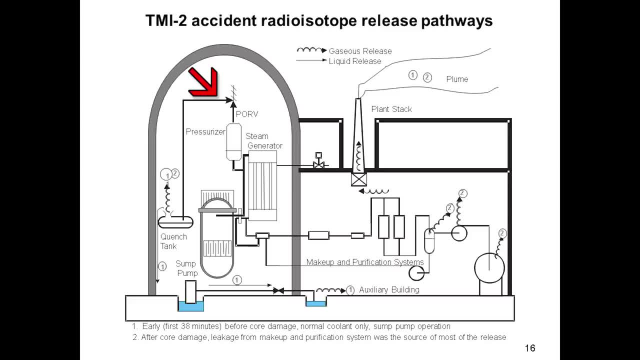 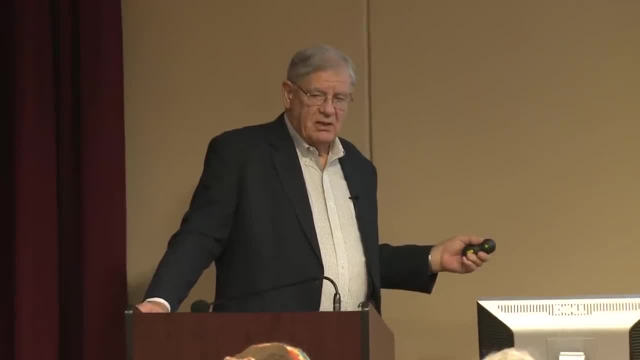 What really caused it was the fact that the feed water system failed and that was because they had some condensate polishers that clogged up. And when the condensate polishers clogged up, that shut down the pumps in the feed water. 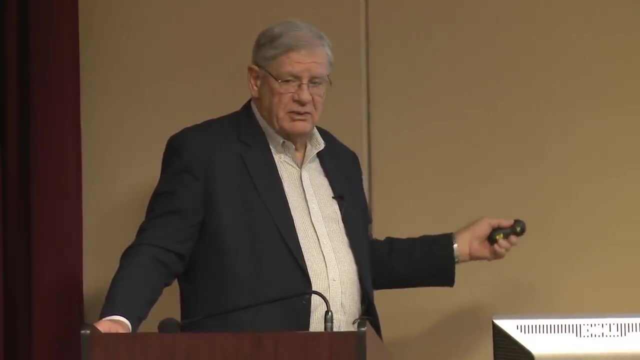 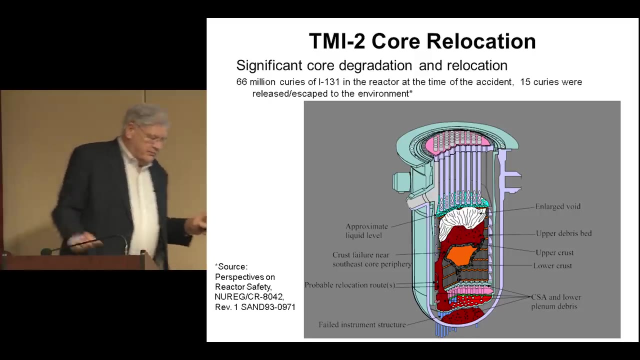 system. That's what caused the feed water system to stop putting water into this generator. This is a picture of the reactor core. I don't know if you can see it there. This is sort of what I call a chocolate-covered cherry approach. 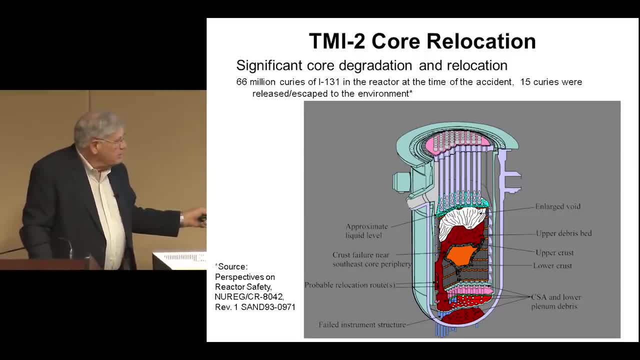 This is the – in the center part. there, that's the molten material. Then there's a crust which is basically – it's like it's material that basically started to melt, But it's crusty, It's thick, It's not molten. 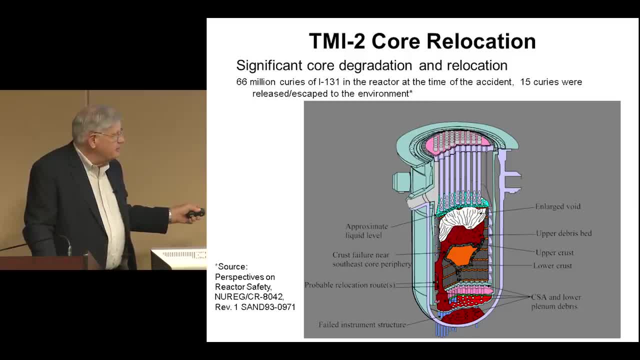 Then you got a crust failure over here on the southeast core periphery. It actually got to the point where it burned through. Then what happens is this molten material was able to run down and accumulate down here in the bottom of the vessel. How thick is the steel in that vessel? 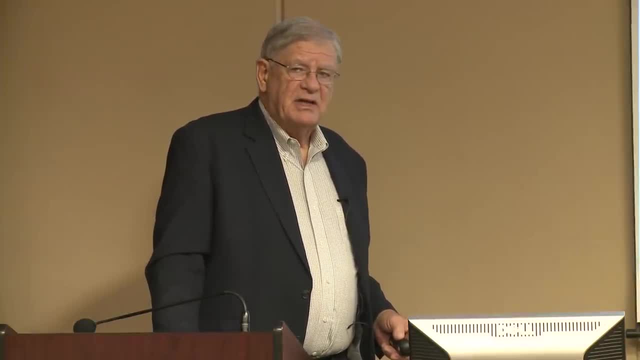 You said it didn't go through in the bottom. The vessel is – I think they're about – Four or five inches. No, they're eight or nine inches thick. They're about four or five inches thick, Four or five inches thick steel. 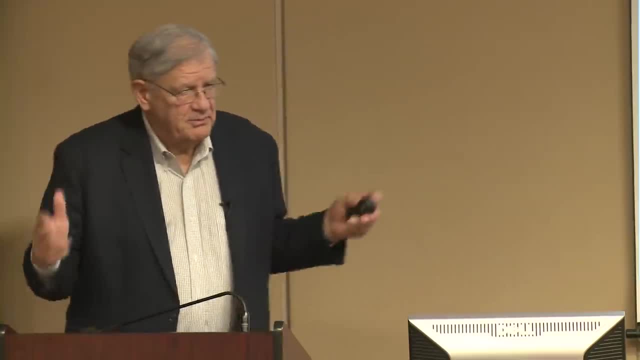 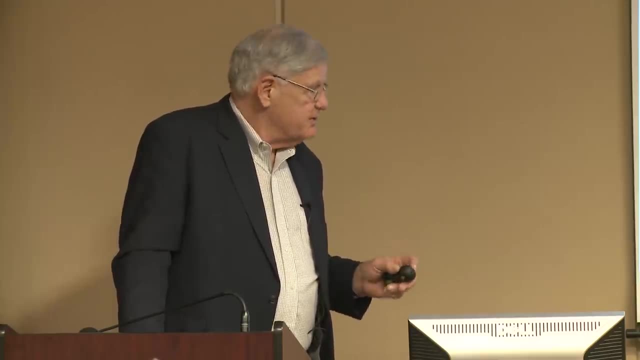 I mean, these things are massive, Yeah, and I'll talk a little bit about it when I get to Chernobyl- because they did not have the capability to build these big steel vessels, which is why they had what they did at Chernobyl. 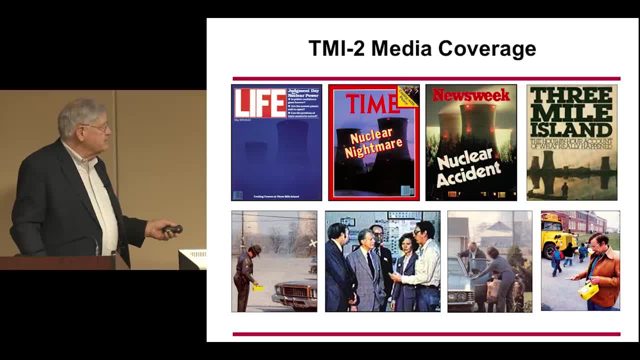 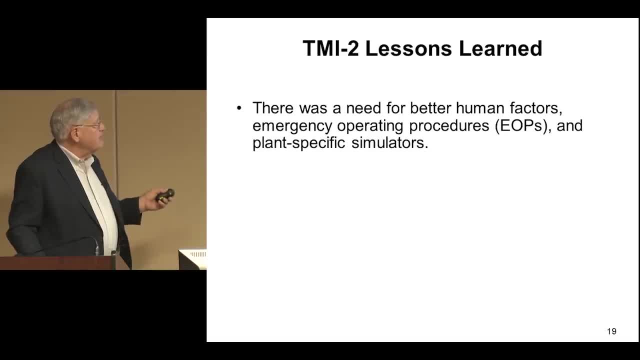 This is just some of the press that went on at the time. It was pretty scary. Lessons learned: There was a need for better human factors, emergency operating procedures and more plant-specific measures. In other words, we needed to make sure these operators were trained for a host of different 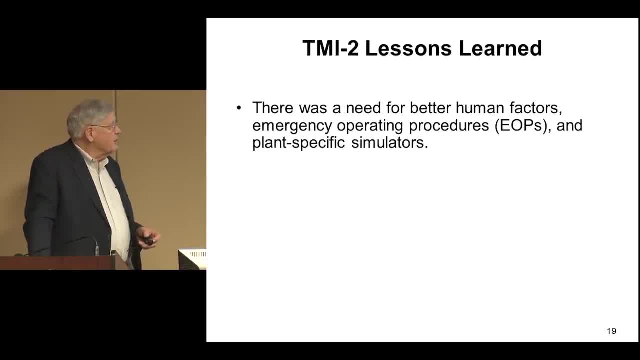 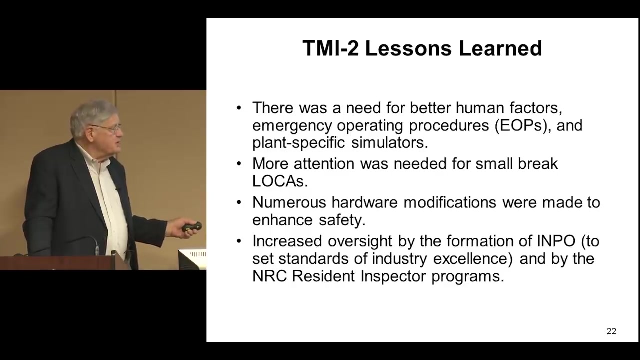 scenarios, and not just these design basis ones. We needed to focus more on the smaller breaks, which were considered to be a much higher probability and much more likely. We made numerous hardware modifications to the plants to help protect against this. The industry itself increased oversight by the formation of INPO. 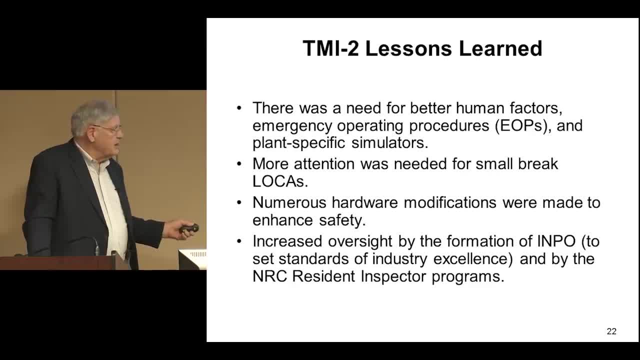 Which is the Institute for Nuclear Power Operation. They're down in Atlanta And they basically were required to set standards for industry excellence in terms of training and the like, And they went out and they would actually test plants and operators to make sure that they had the proper training programs. 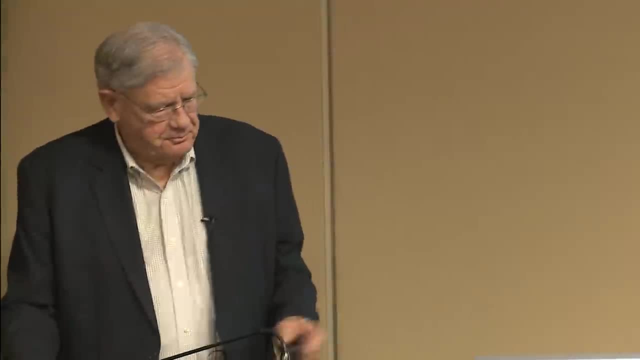 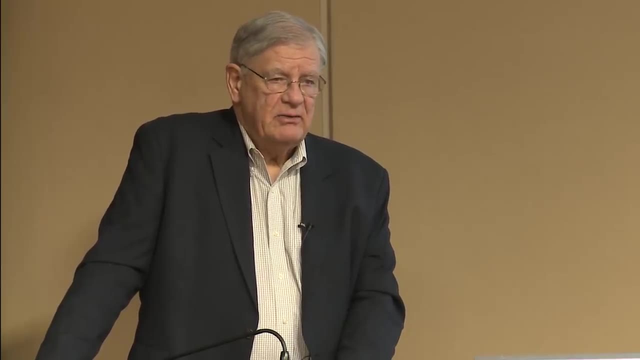 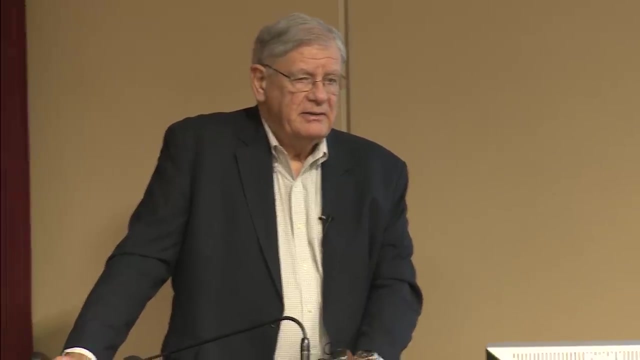 We also created the NRC Resident Inspector Program. Before TMI there was no NRC presence at the plants on a continuing basis. After TMI we now have resident inspectors. They actually live in the area, They have offices on site and they are constantly walking around the plants doing inspections. 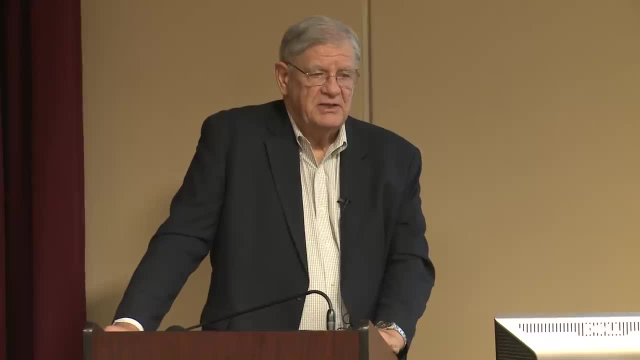 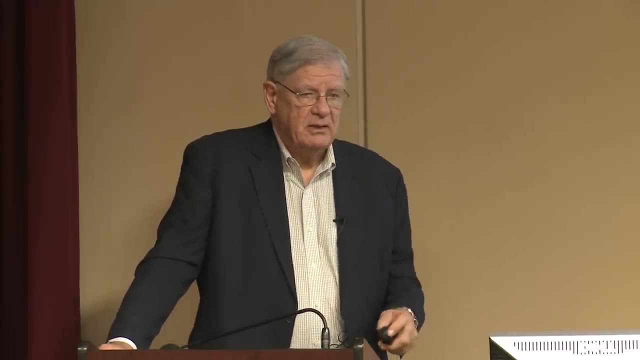 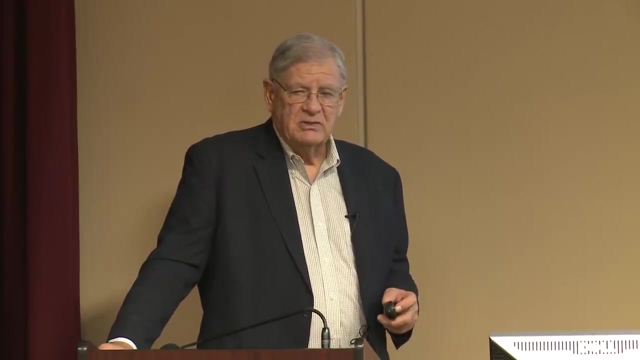 And if they find violations of our regulations they cite them and the like. So we have now at every operating nuclear plant across the country. we have inspectors on site every day. So if you have any concerns you can actually call right to the site and these people are. 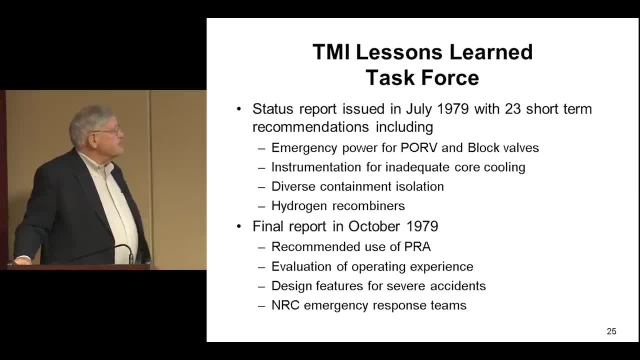 there There was a Lessons Learned Task Force. there were a lot of task forces, But here's a. I won't- I'm not going to read these for the sake of time, But this just goes to show some of the some of the changes, the short term recommendations. 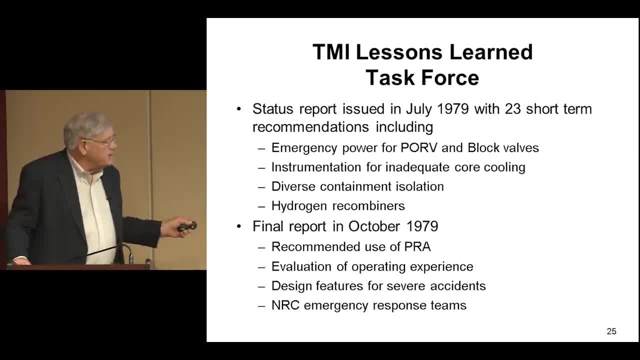 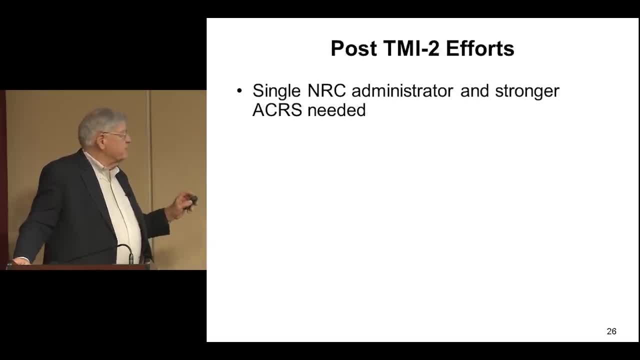 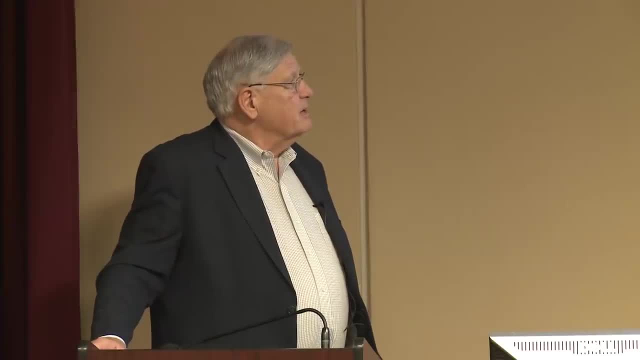 that were made. And then I'm going to go through the recommendations in the final report. One of the recommendations was for a single NRC administrator and a stronger advisory committee on reactor safeguards. No one adopted the NRC single administrator because we have five commissioners at the 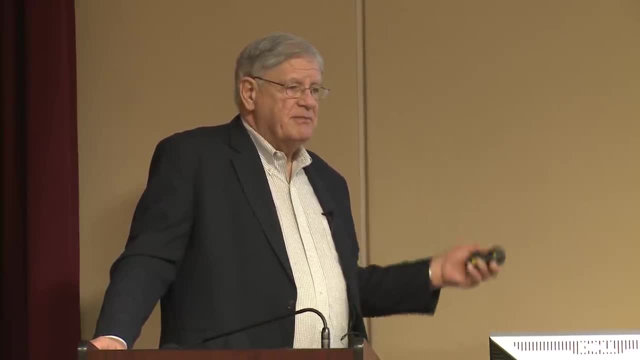 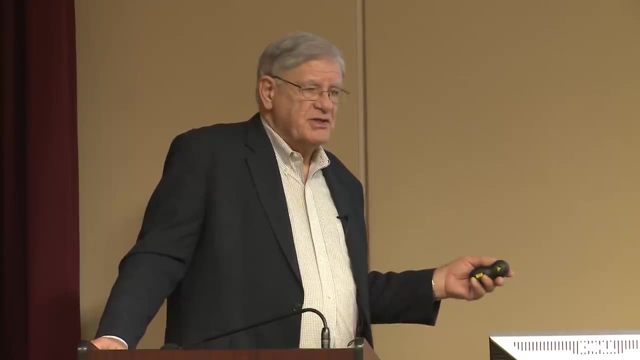 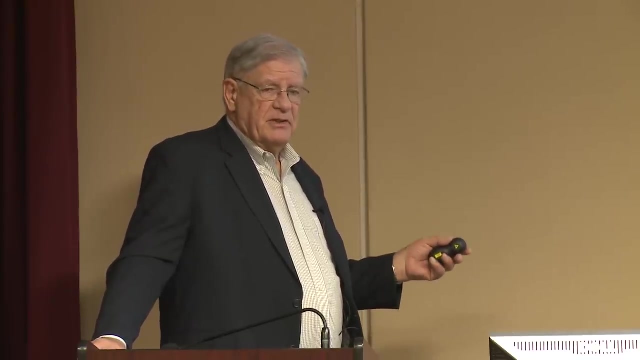 NRC and they like the collegial atmosphere. It also prevents somebody from having a political agenda Trying to We're a safety organization. Our job is to determine whether or not a plant is safe to operate, And we should be. the agency needs to be apolitical. 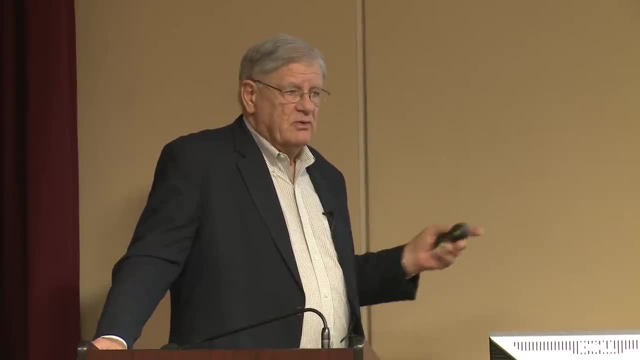 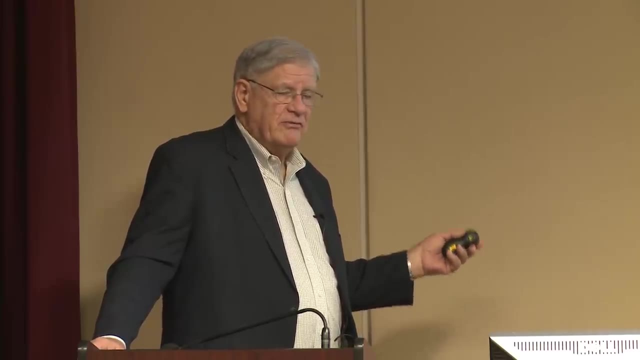 And so we felt having five commissioners, and the way the rules are is that no more than three commissioners can be of any one party. So if you have three Democrats and two Republicans, you have a Republican president- I'm sorry, a Democrat president and a Republican goes off the commission. 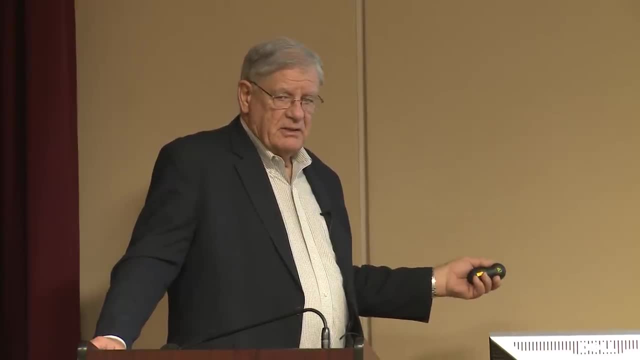 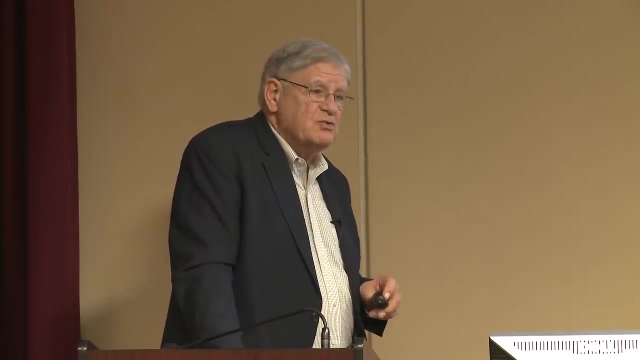 The president cannot do anything. The president cannot do anything. The president cannot do anything. He has to nominate a Democrat. He has to nominate either an independent or a Republican, and vice versa. Over the years I've been there, I would probably say I only thought there was one or two commissioners. 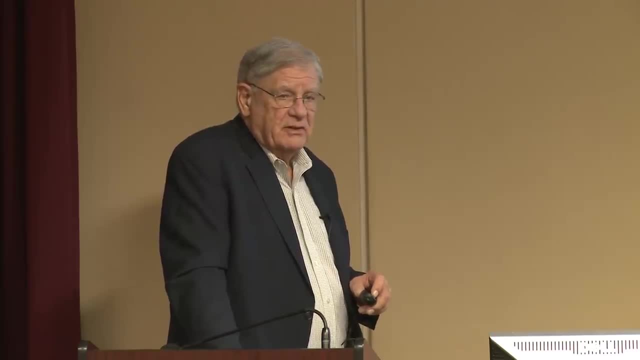 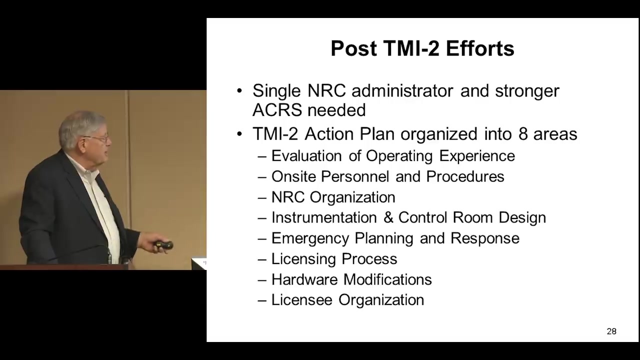 that I think came in with political agendas. The rest of them, I think, were pretty much apolitical, despite who nominated them or the like. They pretty much focused on safety. I won't talk about the action plan. You can read that. These are all the areas that we focused on, though. 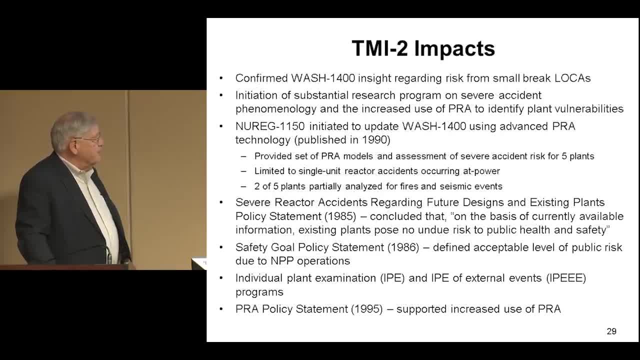 These are the impacts. As I said, pretty much it told us that we're focusing on the wrong accidents. PRA became a big tool for us after this probabilistic risk assessment as a way to identify what the most common or most probable accidents are. 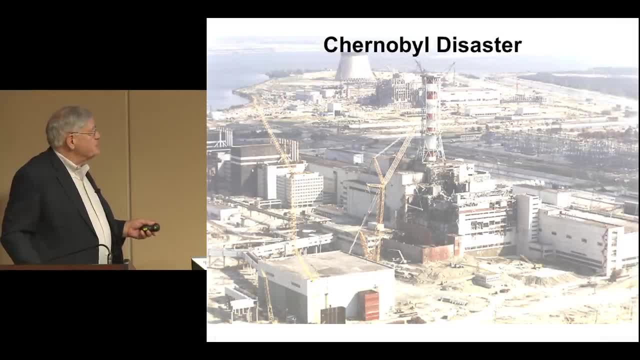 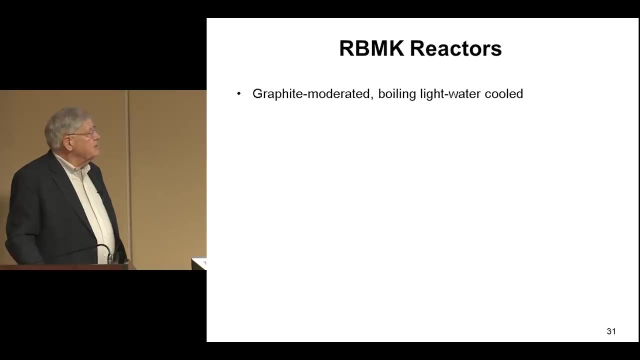 Okay, Let me skip now to Chernobyl real quick. This happened in. I think it was April of 1986.. They have different reactors than we do. We have pressurized in what we call light water reactors. They have what's called an RBMK. 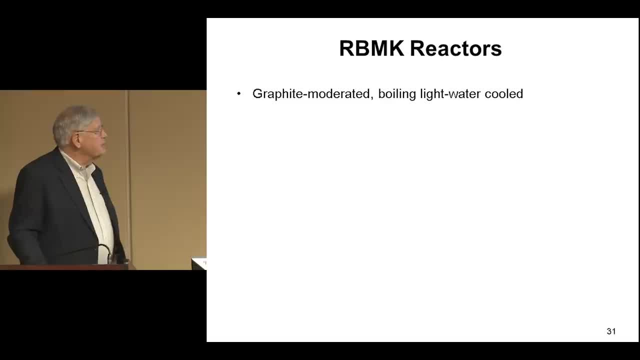 I can't remember what the acronym is in Russian on that, but it's basically a graphite-moderated boiling water, Boiling light water, cooled pressure tube design. They don't have these big containment buildings around them, They have pressure tubes. They have UO2 fuel with zirconium alloy cladding. 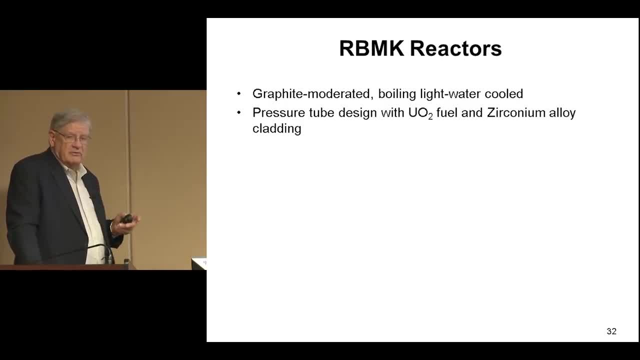 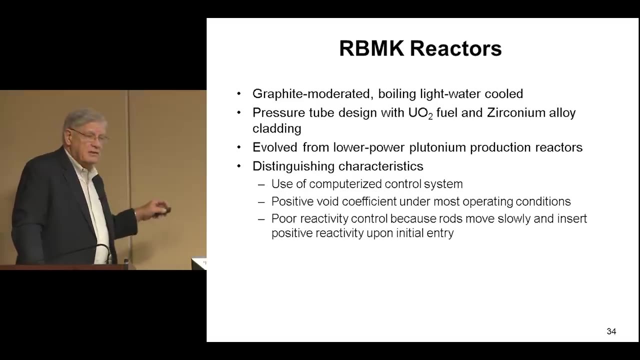 But these are embedded in graphite. Graphite's a good moderator for neutrons. These evolved from lower power plutonium production reactors. They had a computerized control system. They had a thing called a positive void coefficient, Which is scary. That is not something that could not be licensed in this country. 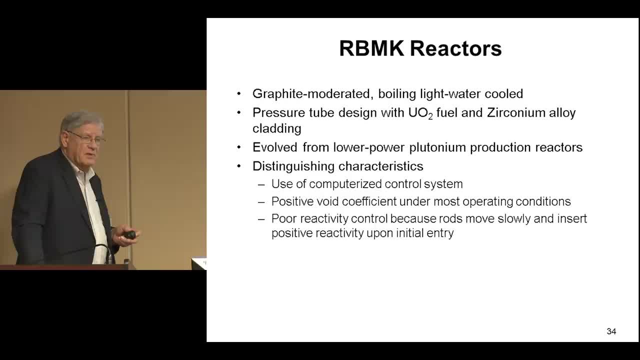 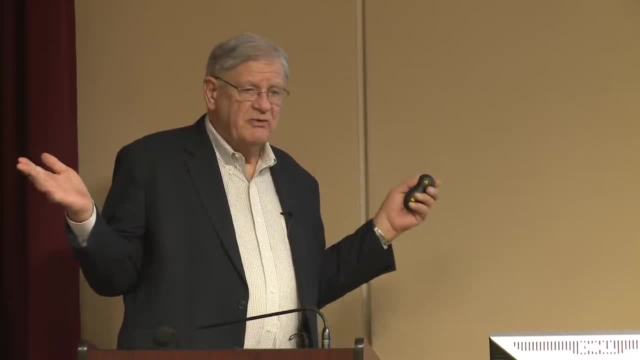 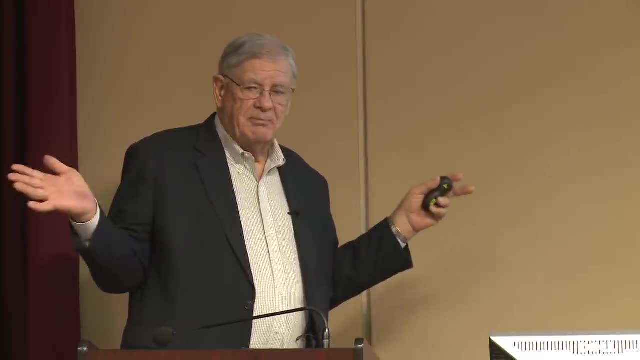 Positive void coefficient. What that means is that when you change the power in a reactor- okay, you change those of you that remember your physics- okay, the nuclear cross section changes with temperature. It broadens- Okay, It's called the Doppler effect and the like. 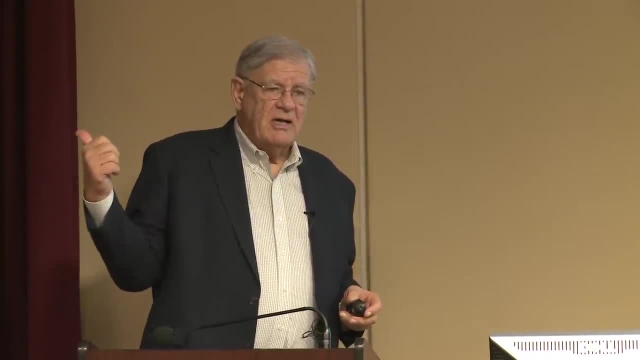 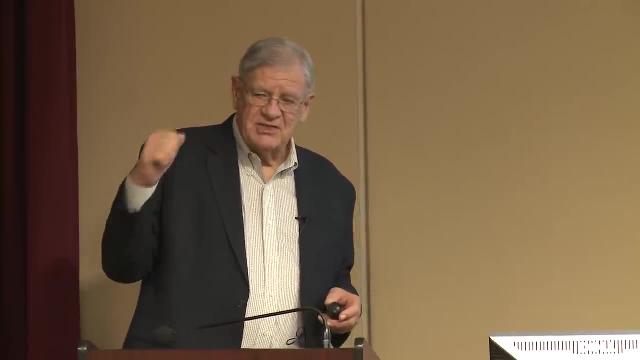 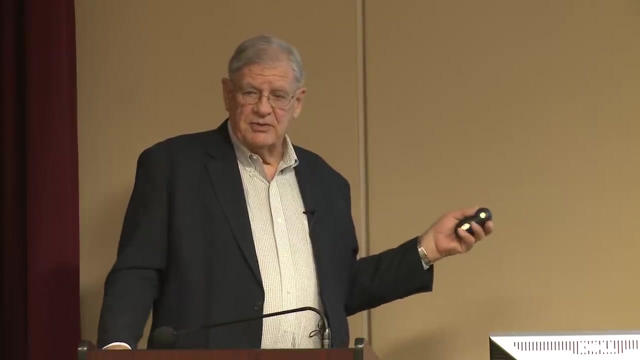 And what happens is that, basically, as you raise the power in a reactor, okay, It provides negative reactivity feedback. okay, So it tends to stop the power from going up. okay, When you have a positive void coefficient or a positive reactivity coefficient, what? 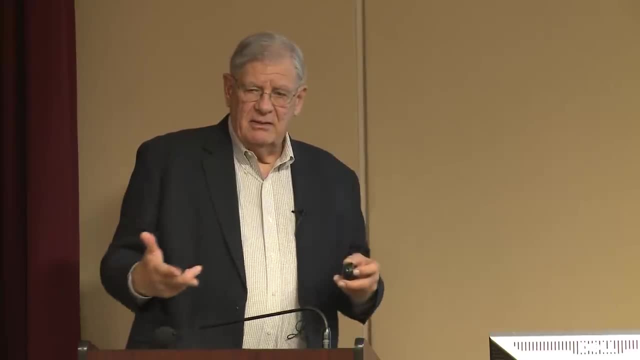 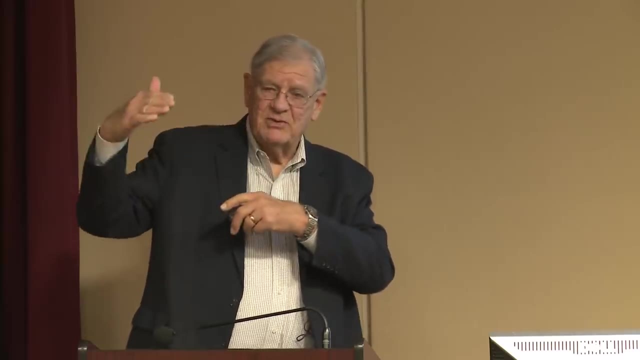 that means is when the power goes up, it increases the reactivity, In other words, it tends to make the power want to go up even more. okay, And what happens? when the power goes up even more, The positive reactivity goes up. 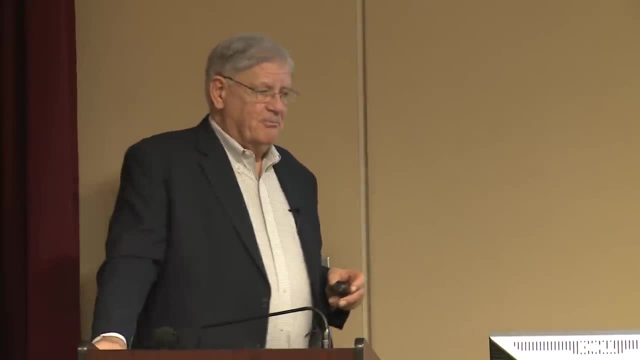 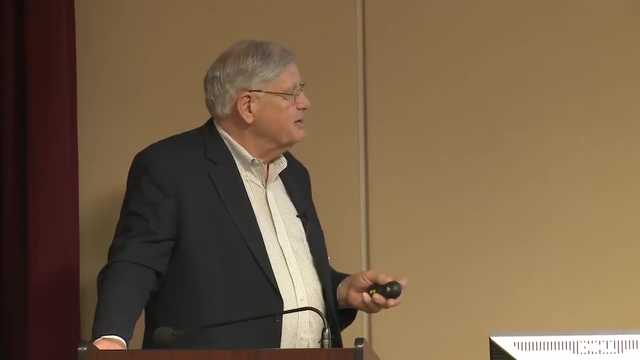 So it's sort of auto-catalytic. Okay, Positive feedback, yeah, exactly, And that's what this reactor had, which was not something that was very good, And they had poor reactivity control because the rods, their control rods, moved very slowly. 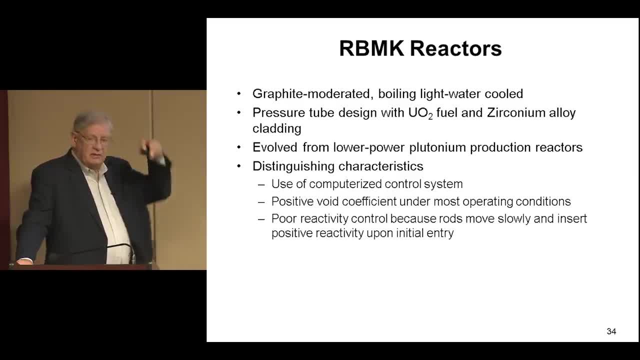 And they actually inserted some positive reactivity when they initially went into the core. Then, once they got further in, they had negative reactivity And they had a very low coolant to fuel ratio. which means that if you, if you, you know. 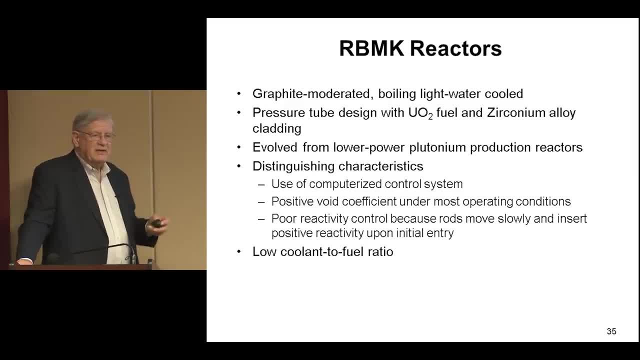 if you you don't have a lot of coolant in there to absorb heat. okay, especially if you start to lose it. okay, And most importantly, they did not have a containment building around it. They had what was called a confinement. 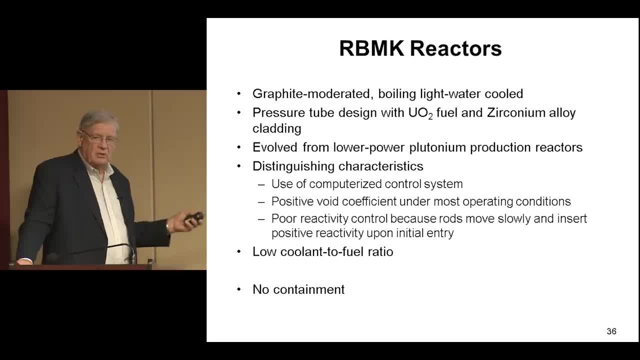 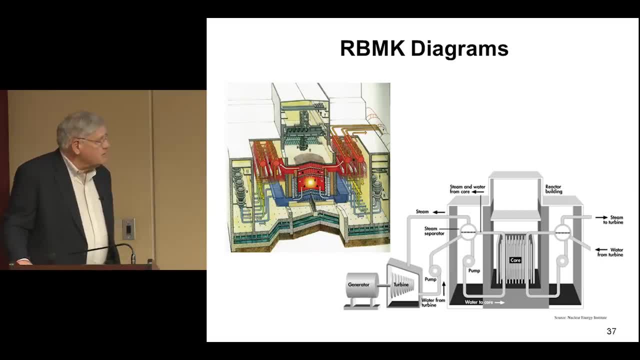 It was just a structure, but it doesn't have the strength and the leak requirements that a containment structure like we use in the US does. This just shows you kind of a cross-section of what these reactors look like. They were big, massive things. 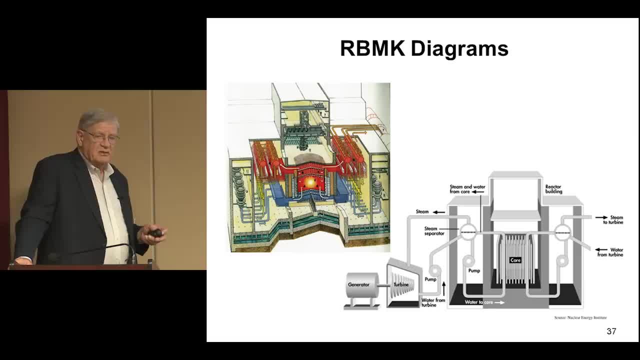 So I said, the reason they went to this design is they did not have the technical capability to produce large pressure vessels like we do. There are only a couple countries in the world that can actually produce these large pressure vessels with eight-inch thick walls that are rolled and welded and everything and the like. 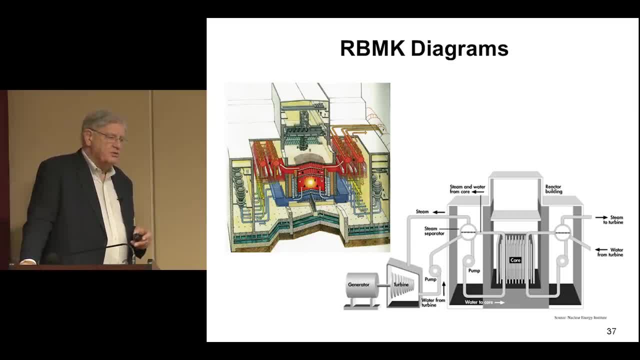 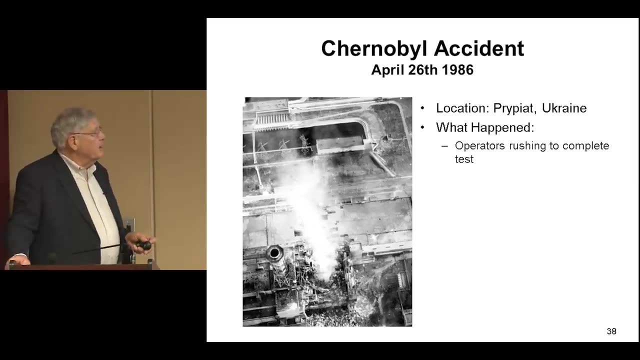 Japan, the US, I don't even know whether we have the capability anymore. It used to be Chicago Bridge and Iron up in Chicago, but I don't think they do it anymore. I think Japan is the only one right now, Now that I'm aware of that's actually making these pressure vessels. 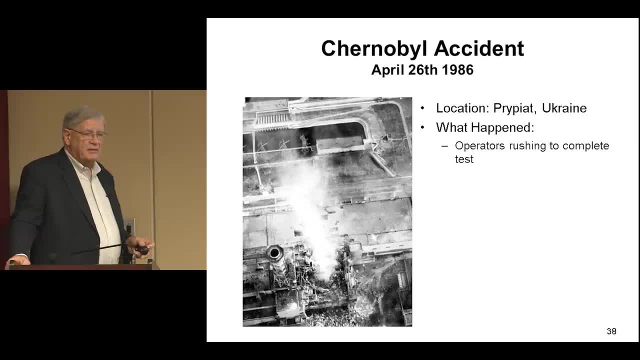 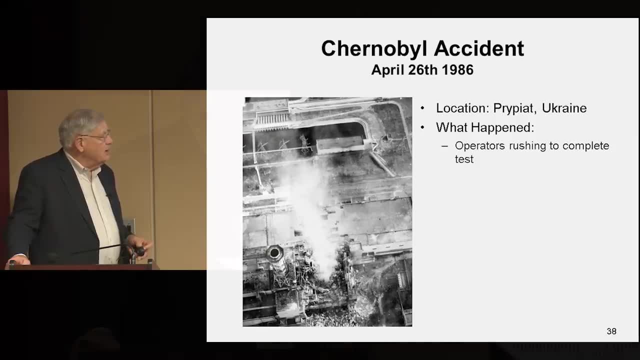 What happened? the operators were rushing to complete a test. They were going to go into a shutdown. They wanted to do this one test and get it over with. What they were trying to do is to see is if they were to trip the reactor pumps, the coolant. 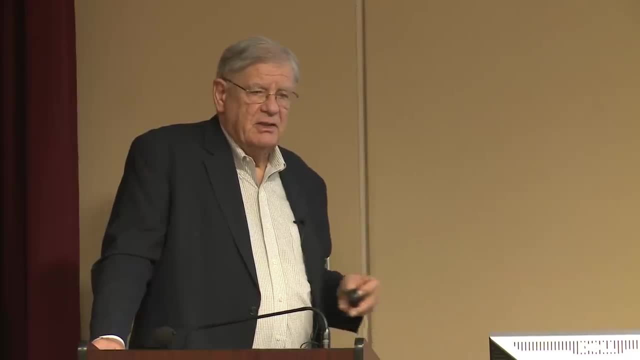 pumps. These are big spinning, these things are huge, okay, Well, If they hooked them up to? they thought that if they hooked them up to a generator, as these pumps coasted down, they could turn a generator which would generate electricity, which would 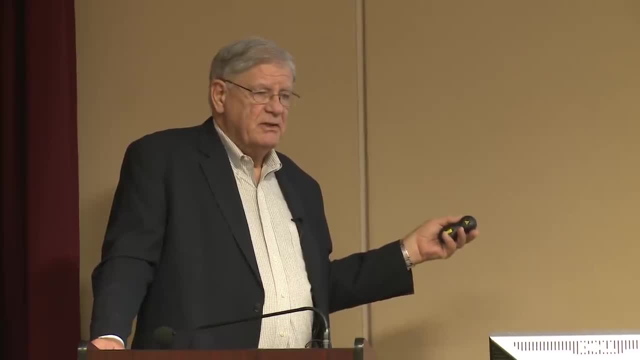 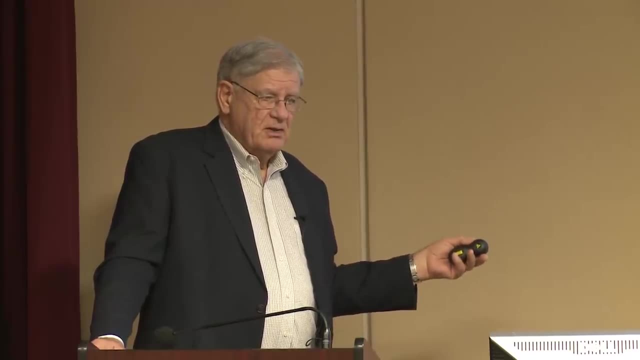 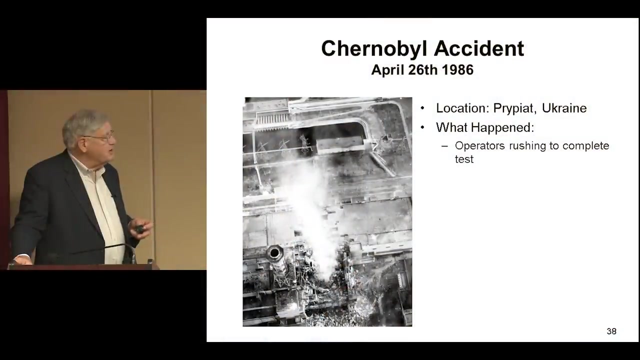 continue to basically energize the grid until if they had diesel generators, those diesels could start up and accept the load. So that was the whole purpose of this test was to see whether or not that would work. They were in a rush, They had complacency. 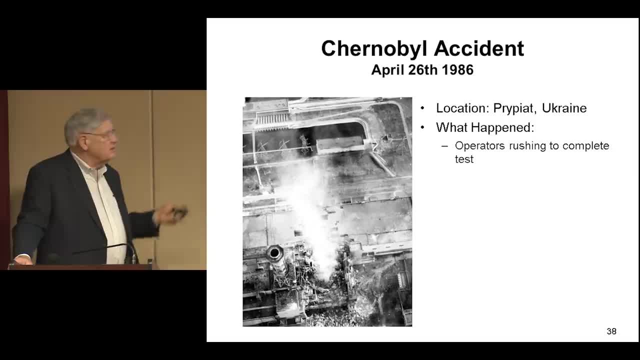 This was a good ready reactor. They felt they couldn't do anything. This thing's always run great. We've never had any problems. They didn't adequately analyze the test and the potential consequences. They turned off safety systems to run the test. What happened is when they did the coast down as the coolant flow through the core went down. What happened is that you generate more heat, more steam, because the flow's going down. So, if you think about it, it's because the water has more time to pass through the core. 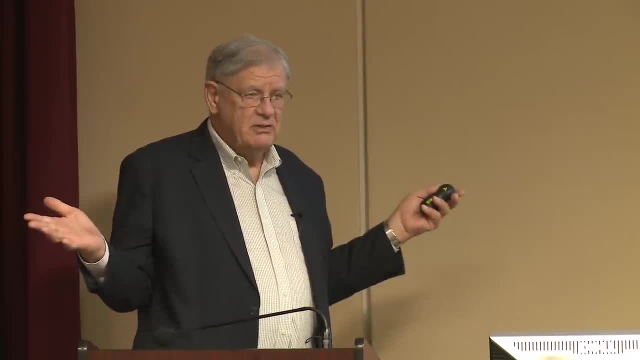 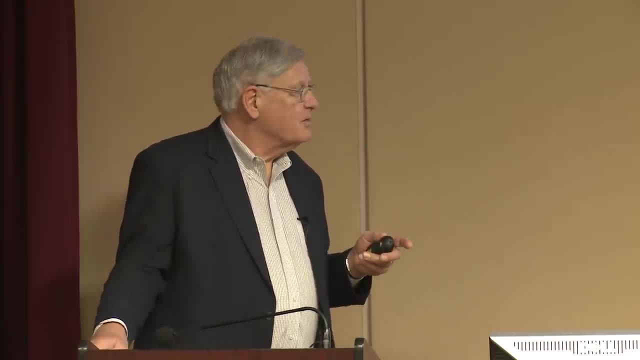 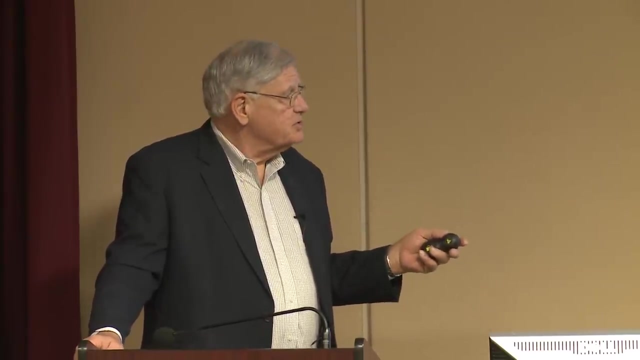 more heat can pass into it, so you can generate more steam. Remember the positive void coefficient? Well, guess what steam is? That's a void from the standpoint of physics. What they did is they generated a large positive reactivity insertion. Okay, This caused so much energy to go. you know, the fuel rods started to increase in energy so much. What happened is they start to expand because they give off fission gases and everything. They literally the fuel rods you know- kind of blew up and went into the coolant channel. 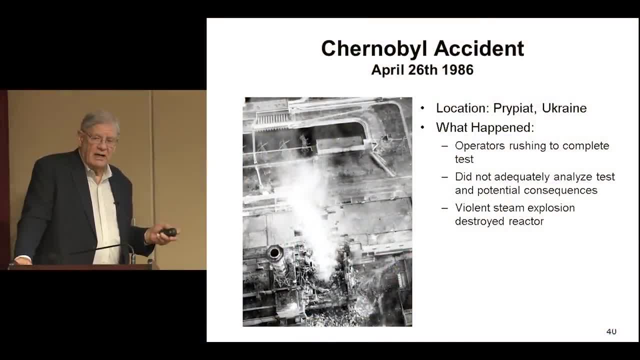 And if you've ever taken something that's very, very hot- you know thousands of degrees- and put it in water, okay, you get a little phenomena called a storm Okay, Okay, It's a huge steam explosion And that's what happened, we think is that they increased the power so fast. the fuel, 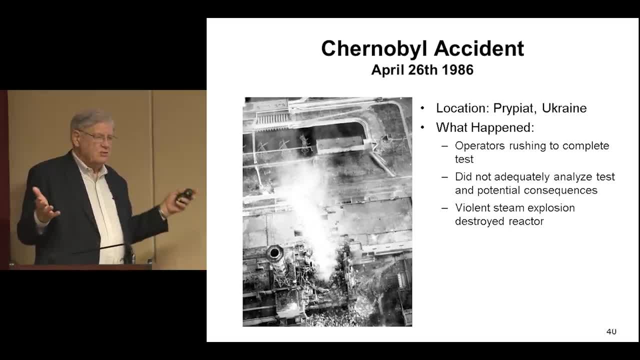 rods failed, They fragmented, went into the coolant channels, hit the coolant and caused a huge steam explosion. And what that is is what happens is that the fuel rods go in there, the water's around it, and all of a sudden you build up this vapor blanket around there and it literally 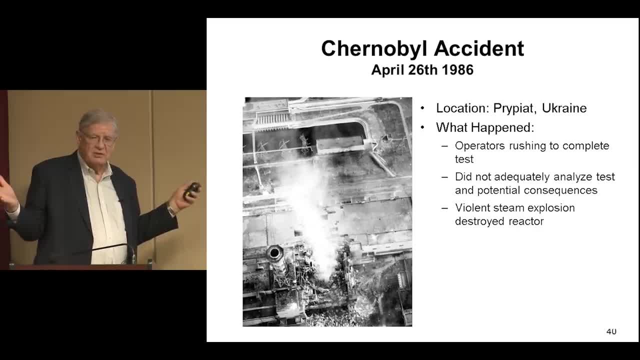 the steam expands so fast. okay, It's like an explosion, And they think that's what destroyed the whole reactor and the containment. Large amounts of radioactive material were spewed all over the place. There were pictures of firemen on the roof of the building trying to put out burning. 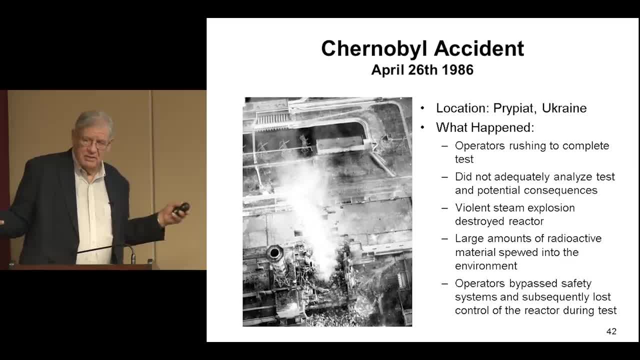 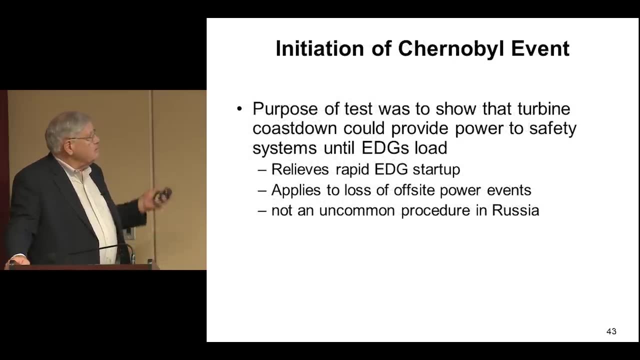 fuel rods standing right next to it with bare. they took off their fire suits because it was so hot, you know, and it was you know, and I think 31 firefighters died from radiation. As I said, the purpose of the test was to show the turbine coast down could provide. 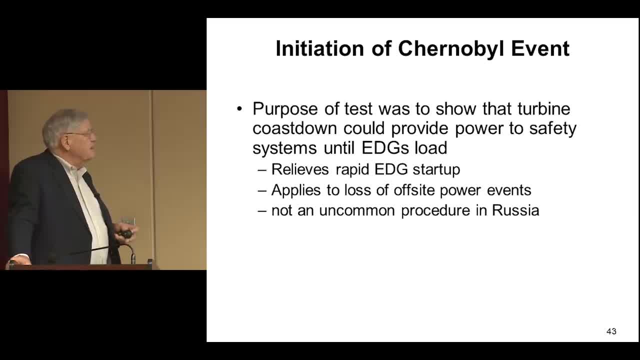 actually it was the turbine, I'm sorry, not the pumps to power the safety systems until the diesel generators loaded. And what that does is what you don't like to do, is you don't like to start these diesel generators cold and load them immediately. 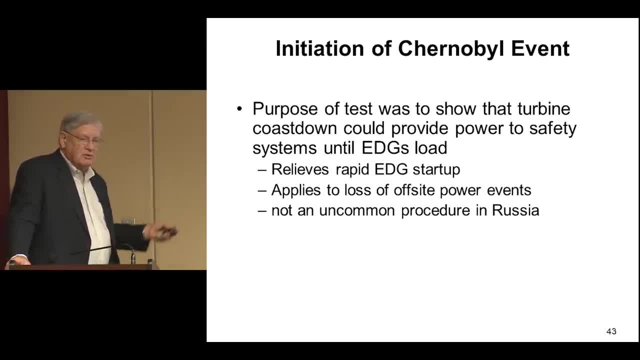 It's just like starting your car up in the morning. okay, You like to let it run and warm up a little bit before you go out there and get on the beltway and do 70 miles an hour. This was not an uncommon procedure in Russia, but they had virtually no additional safety. 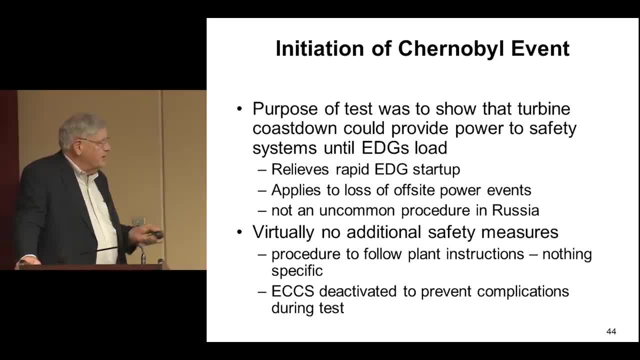 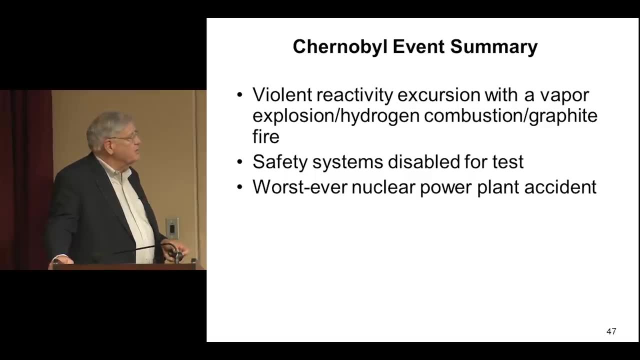 measures. They deactivated, as I said, the emergency core cooling system, the ECCS, to prevent complications during the test. They got a violent reactivity excursion with a vapor explosion and then there was hydrogen also generated and we think that contributed. 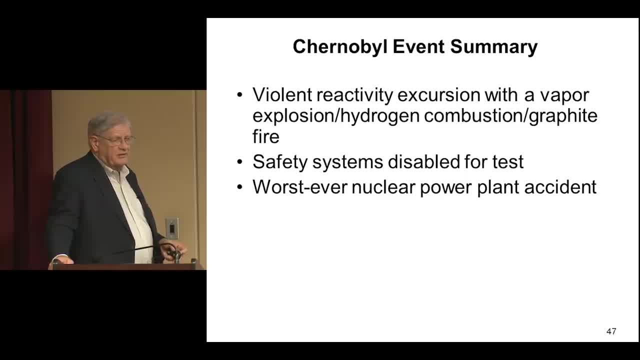 There were two explosions. The first one, we think, was a steam explosion. Nobody knows what that second one was. They speculated it was a second steam explosion. Others speculated it was hydrogen. Nobody really knows yet. The plume spread into Europe was first detected, I think, over Norway, and that's when people 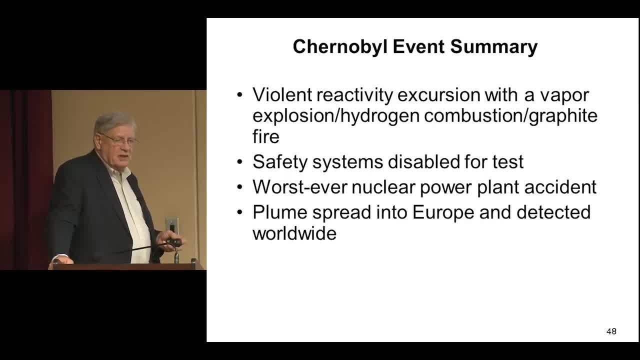 started asking questions. The Russians, I think, at first tried to deny it and everything and we couldn't get an any information And I probably spent about a week or two in our operations center and we were just trying to figure out what could have happened there, you know, trying to glean information from 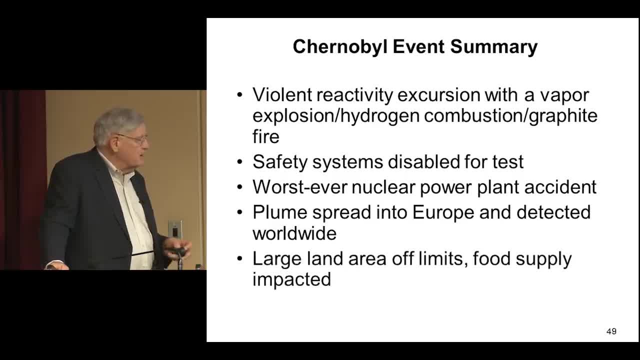 all our sources, overseas and the like, Contaminated large land areas, food supplies- I think there's still television shows on you can watch and it still talks about about a 30-mile radius areas that just basically deserted around there. And the other level of innovation was that we were putting out part of the nuclear reactor. 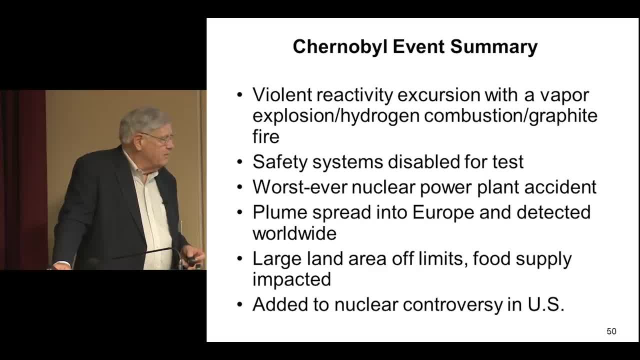 on top of those reactors in the US, Even though those reactors could never be licensed in this country, and we tried to explain that it did add to the nuclear controversy not only in the US but worldwide. I think I went over to Europe five times that year to write a report for the OECD which 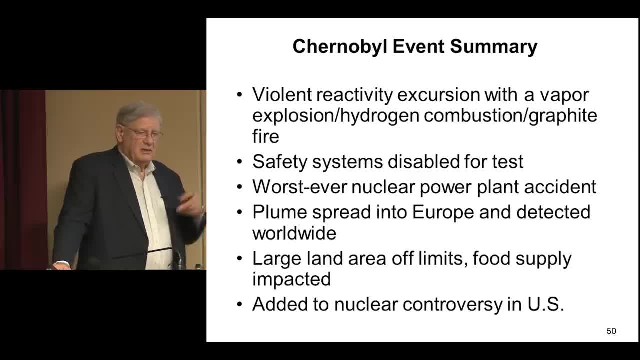 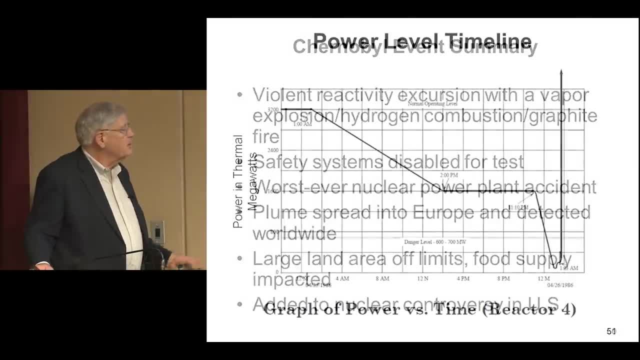 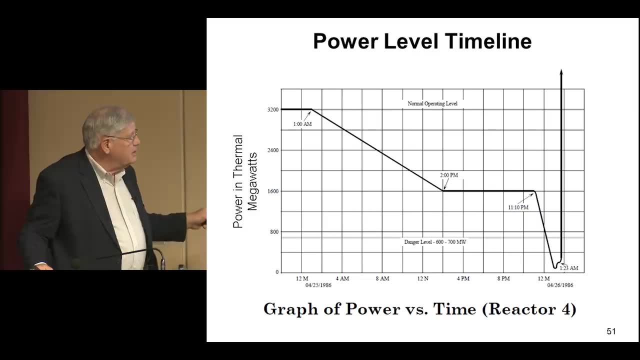 is the Organization for Economic Cooperation and Development on a report trying to basically between Western reactors and the Russian RBMKs. This shows just the power trace You can see. they were operating. The power came down. Then they tripped a reactor. 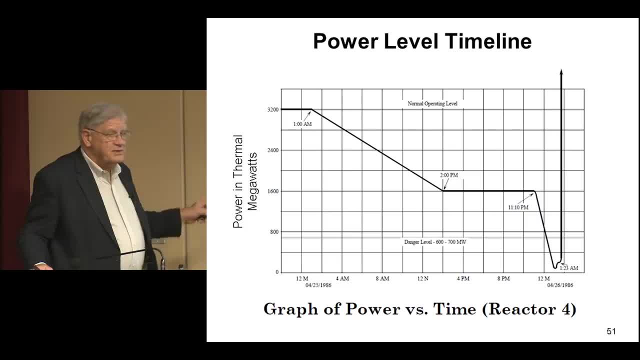 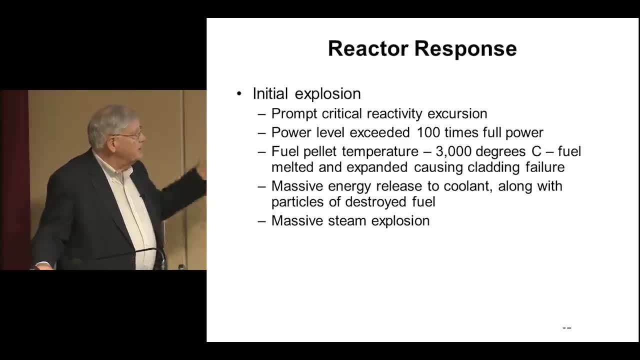 And then they had this power excursion And you can see what happened. It just went through the roof. I'm not going to just explain most of this, As I said. second explosion: it's possible hydrogen or carbon monoxide explosion, But that blew the roof off. the building started 30 fires. 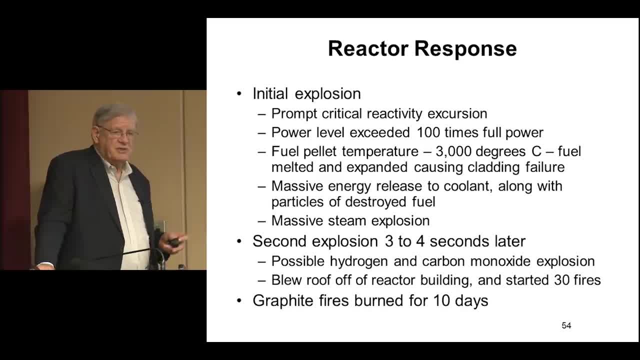 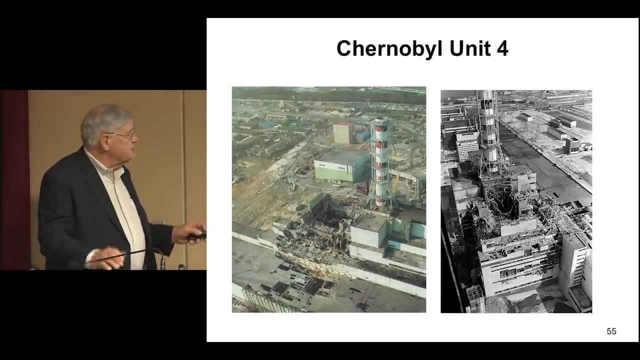 And they had graphite fires there for 10 days. This is when you see the pictures of the helicopters trying to drop sand on it and everything to put them out. These are some photos. This is the destroyed reactor. You can see how violent that was in these areas here. 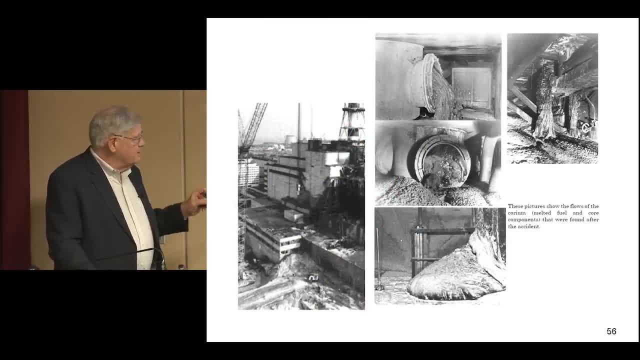 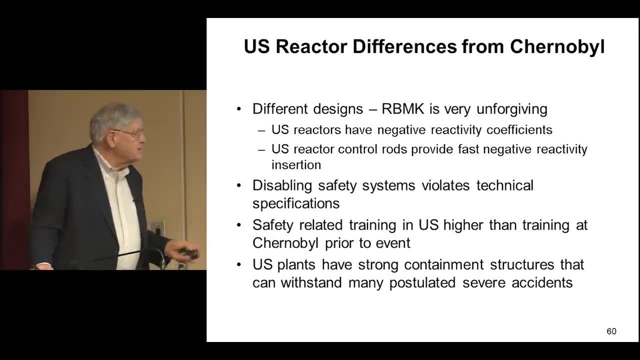 This was a four-unit plant. This is: This is molten material, molten core and material that they found underneath the reactor. I think these are robots that went in there. These are just a list of the differences, in summary, between US reactors and the Russian reactors. 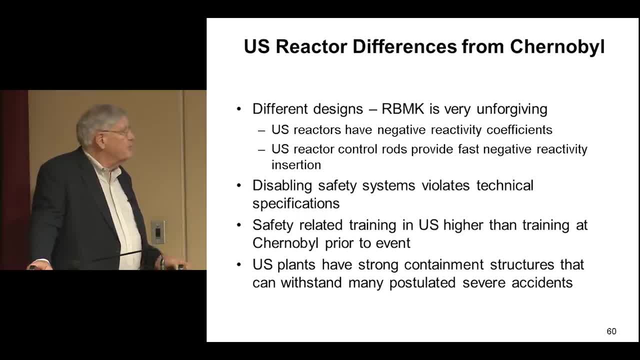 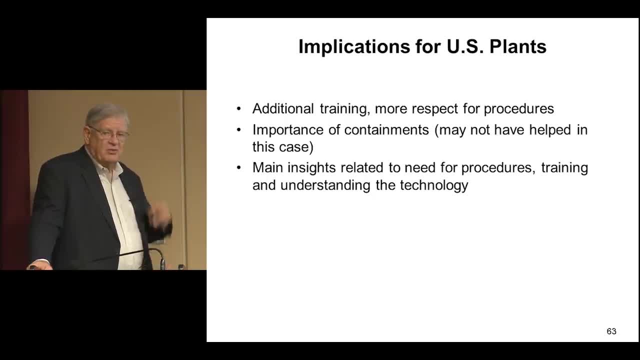 As I said, they're very different. They can never be licensed in this country. Implications for US plants: Again, this additional training. The biggest thing again was this whole question of complacency. These operators were complacent. They felt that they knew this reactor. 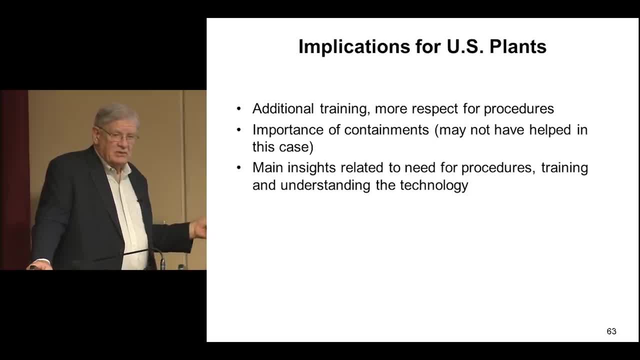 It can do no wrong. Three Mile Island was a little bit like that. The operators just felt comfortable. They knew what they were doing. We always tell people you can't become complacent with your reactors. All right, OK, One of our executive director for operations. 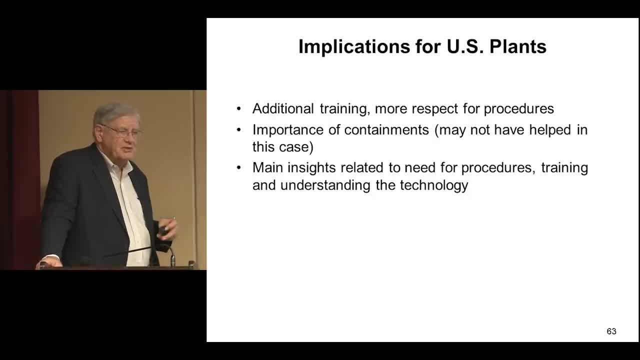 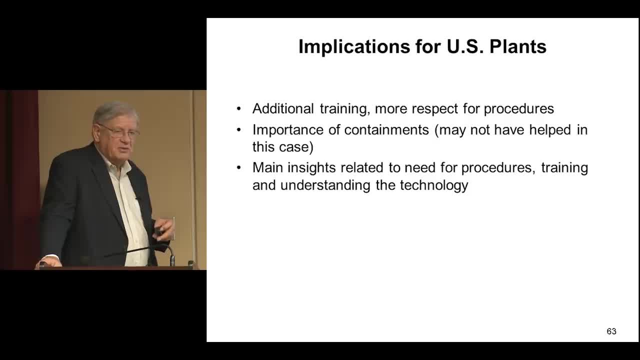 He used to say that the price of nuclear power is eternal vigilance. It's true. So, as I said, the human performance aspects were not unique. They were more focused on success rather than safety, Overconfidence in the facilities and lack of protection. 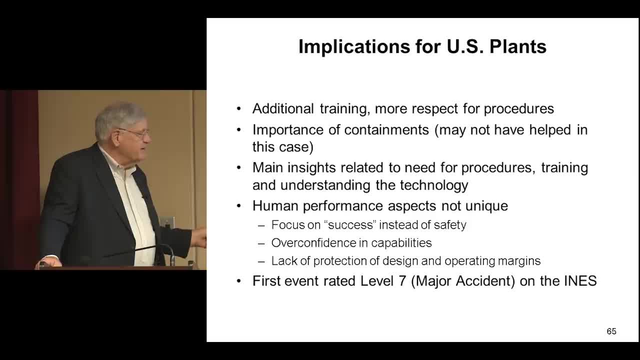 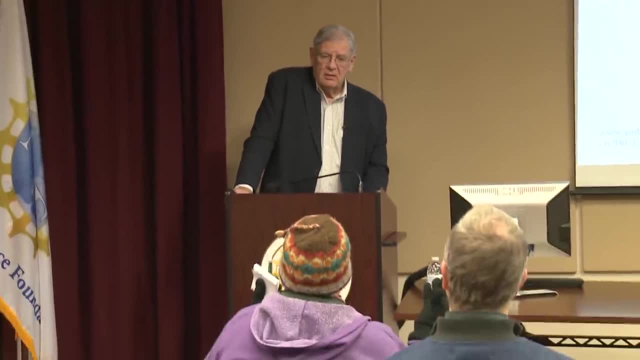 of design and operating margins. This was the first event that was ever rated a level seven On the international nuclear energy scale, which is the scale by the International Nuclear Energy Agency. How come it didn't just explode like a nuclear bomb, Like with a big mushroom cloud? 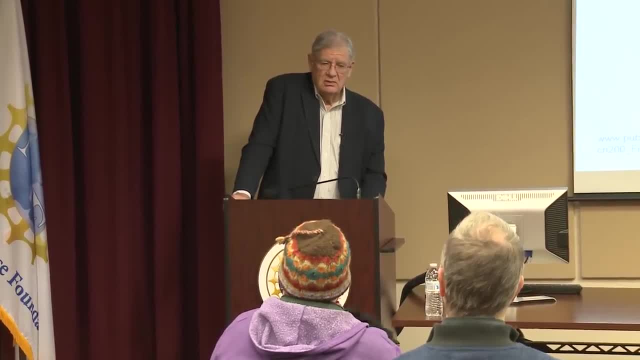 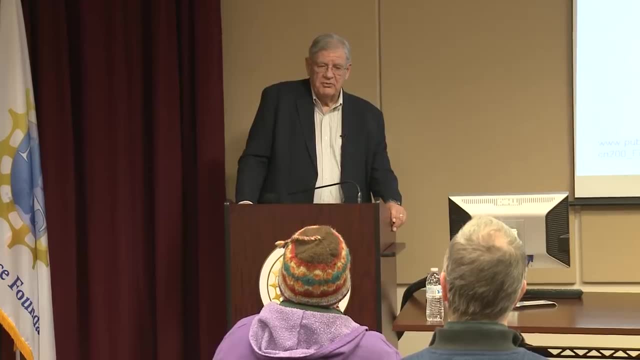 I'm sure it's probably two completely different things, But for somebody who doesn't know this stuff, it's: The physics are not there. There's not enough highly enriched uranium, OK, OK, See, that's the whole thing right now. For example, a lot of the utilities. they want to extend the life between refueling outages because that's money. Every time they go down for an outage, that's a month where the reactor is not generating electricity And these plants earn about a million dollars a day. Probably even more now, And so they want to extend the life or the time between outages. Right now it's anywhere between a year and a half and two years, And then they've got to shut down and refuel. Well, if they can go to higher enrichment. if they can go to higher enrichments, then they can burn up more fuel, which means they can have longer times between outages, which translates to money. Problem is that once you start getting into higher enrichment fuel, you have proliferation concerns and all sorts of stuff. 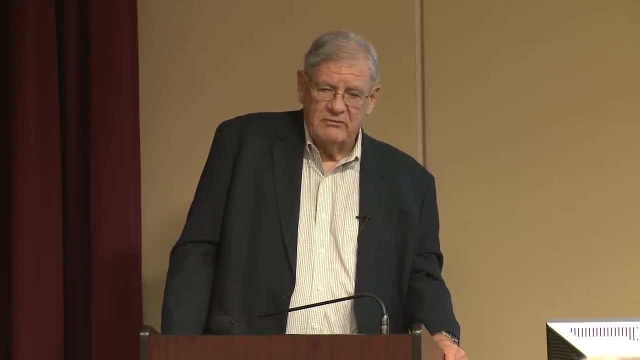 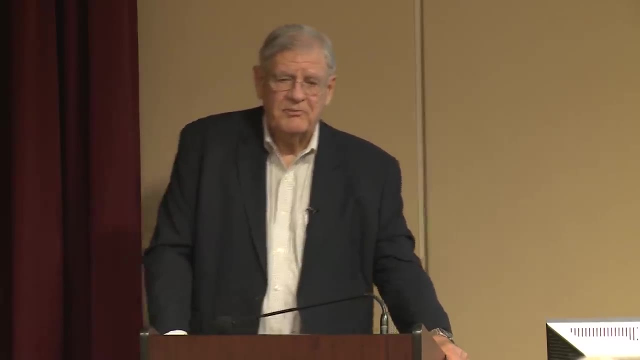 So right now we have a limit on the amount of enrichment. This is the percent of U-235 in the U-238.. And I think that's at 4% now. OK, Thank you, But you have to get up much higher than that. 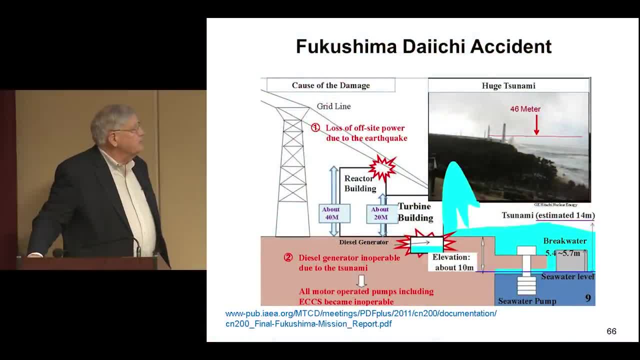 to get to actually where you have a bomb. With regard to Fukushima, OK, what happened? They had a big earthquake, Richter 9, out in the ocean, generated a tsunami wave. The wave was very high. They had a seawall that was, I think, about 20 feet or so. 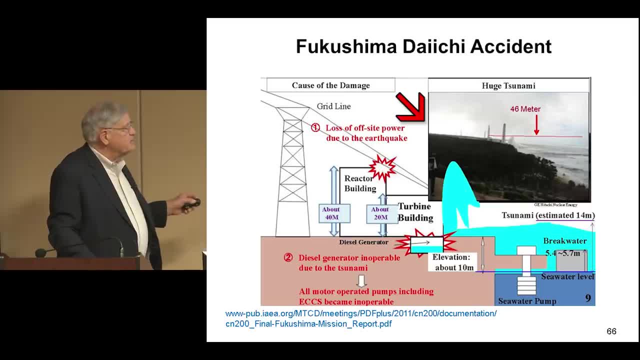 But anyway, the tsunami wave Just washed right over it. It was way too low, OK, And what happened is that the diesel generators were below grade. You can see right here they were below grade. Once that water comes over and they're below grade. 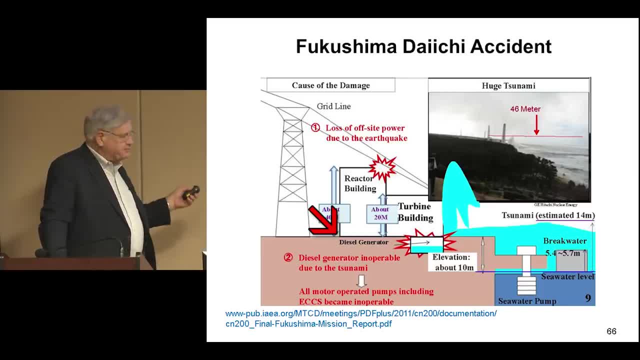 it just goes in and floods them out. So what happened is they shut the reactors down. It took out the transmission lines coming in. loss of off-site power: OK, There's no electricity coming into the plant from off-site. The diesels are flooded because the wave goes in there. 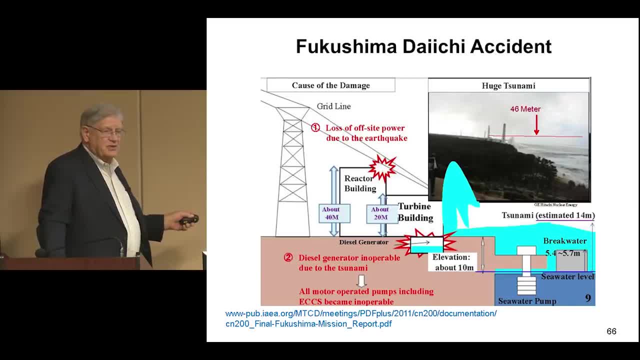 and just floods out the room. OK, So they have no diesels to start up And the only thing they have is batteries, And the batteries were below the grade level. OK, So the batteries were shorted out. OK, So they basically went into what I described before. 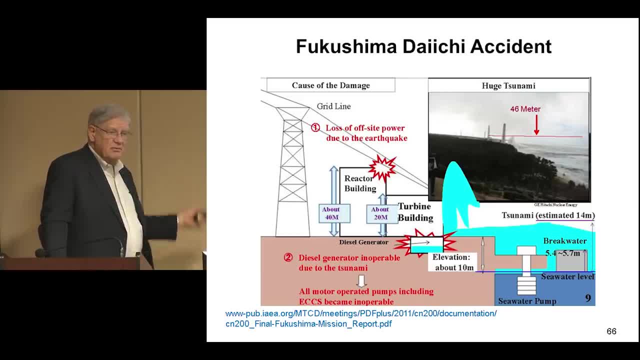 as a station blackout. In other words, I got a reactor there and I have no way to power pumps, valves, anything. I have no instruments, No lights And, as a matter of fact, some of the crew were actually running out to their cars. 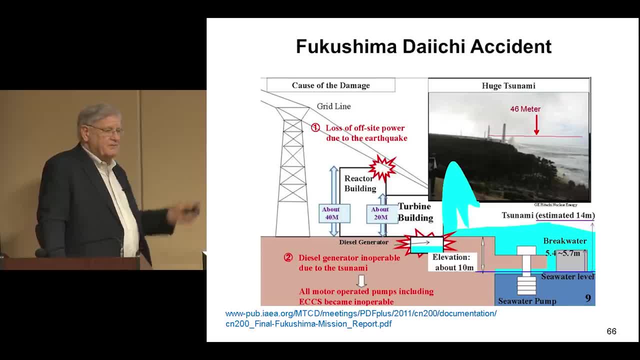 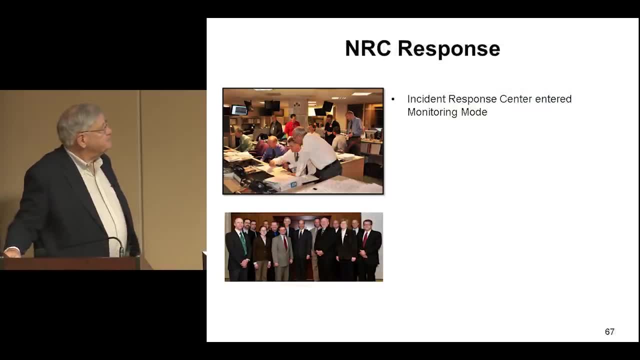 trying to get their car batteries out and trying to hook them up so they could get batteries, so they could at least get some instrumentation and figure out what was going on. We initiated our incident response center down in Rockville And we staffed it 24-7.. 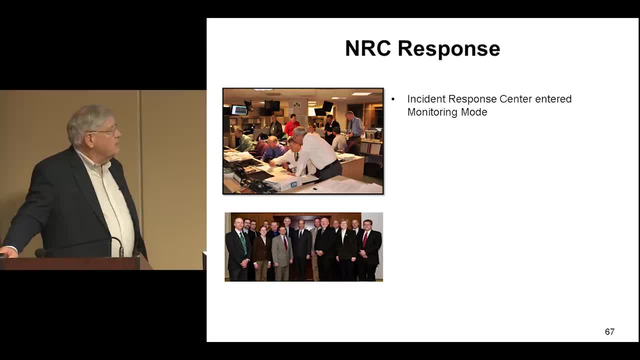 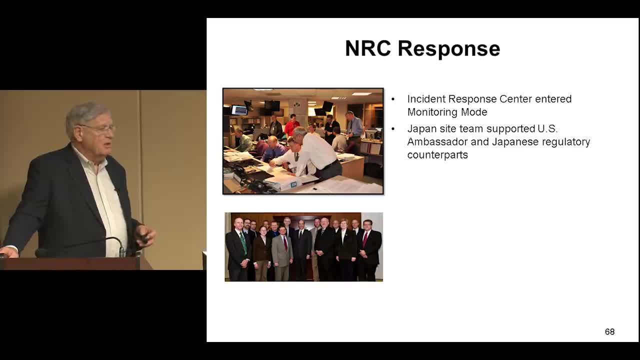 We had several, including some of my staff- went over and spent several weeks in Japan doing that. We had a near-term task force and we did a systematic review of what went on and whether we needed to do anything. Near-term actions included conducting additional inspections. 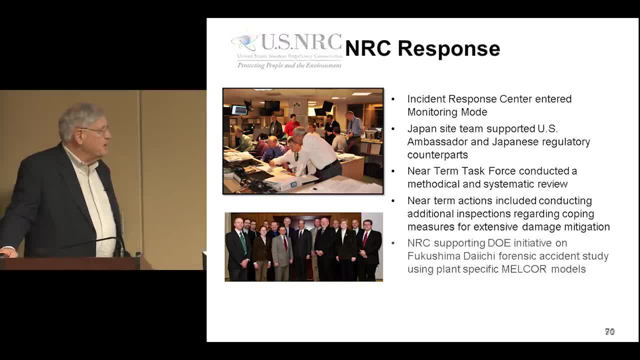 regarding coping measures for extensive damage mitigation. We supported a Department of Energy initiative on Fukushima Daiichi forensic accident study using plant-specific. MELCOR is a computer code that we had that the NRC developed on severe accidents. What we concluded for the US was that there 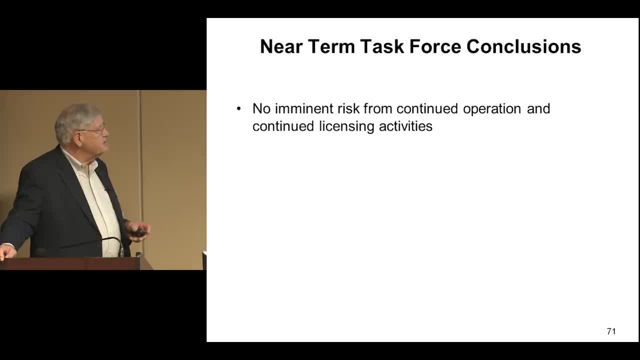 was no imminent risk from continued operations and continued our licensing activities. We said a similar sequence of events in the US is not likely. And what we did is we said, OK, can we get a tsunami that's going to flood out a plant? On the West Coast there's only two plants. There was Palo Verde- I'm sorry, not Palo Verde, Diablo Canyon and I'm sorry- And San Onofre, And San Onofre, And San Onofre, I think, is shutting down. 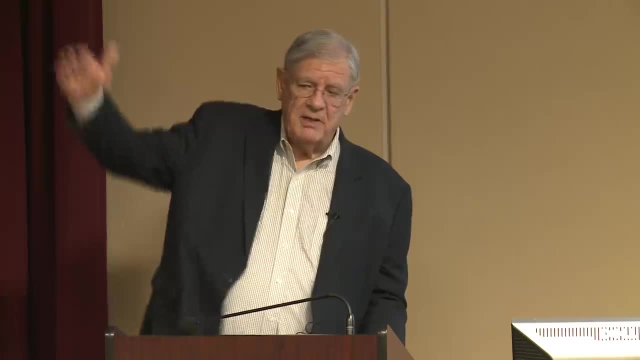 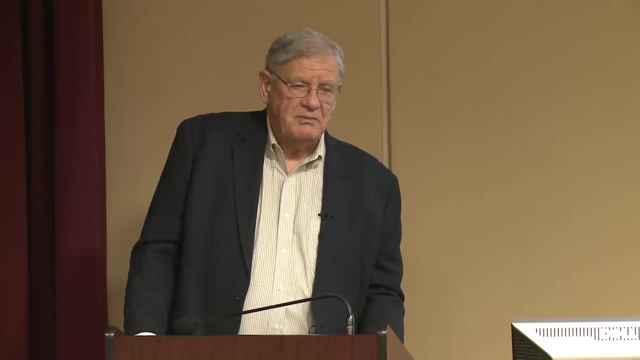 But Diablo. Diablo is actually. if you've ever been out there. it's up about on a cliff, on the side of a mountain, And if you had a tsunami that got up that high, you got bigger problems. Trust me, When you looked on the East Coast, where we have some plants, 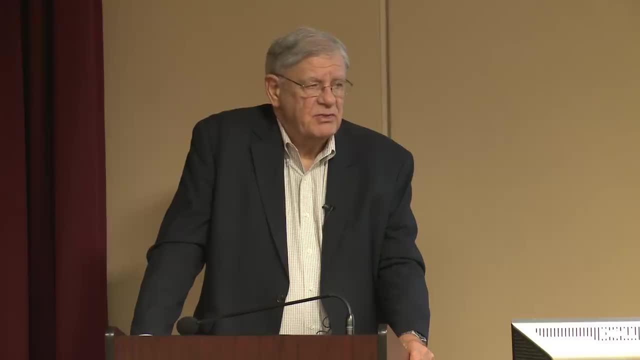 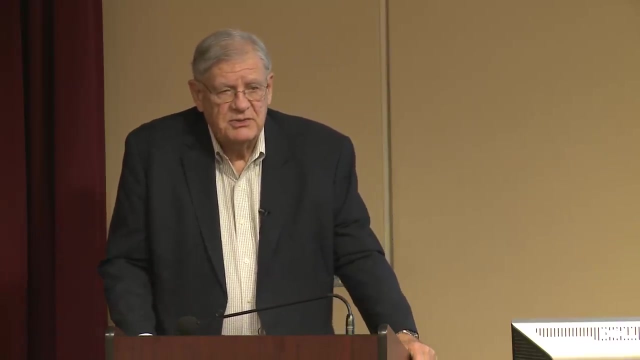 on the coast. what we concluded was that the biggest threat was not from an earthquake, but from an undersea landslide that could generate a wave like that, And what we concluded was that the waves from hurricanes on the East Coast and storm surges are actually much higher than what 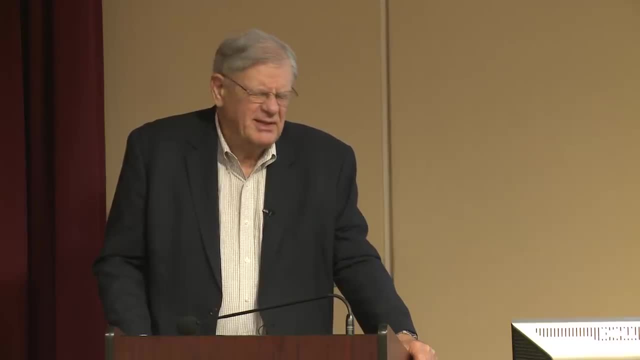 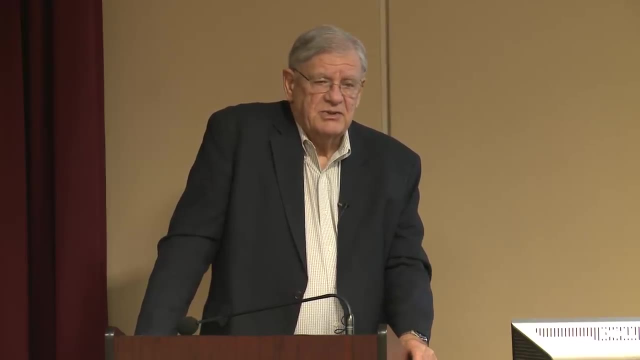 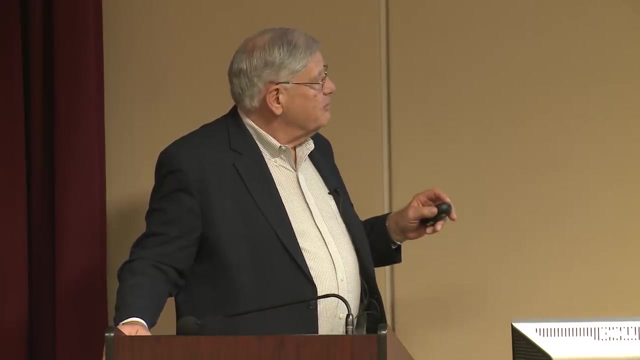 could be generated by an undersea landslide. So basically, what we concluded was that the US plants were still adequately protected and designed against the maximum type of event that could occur from non-rushable water. One of the things that really came about was the question of this, and it's not on here. 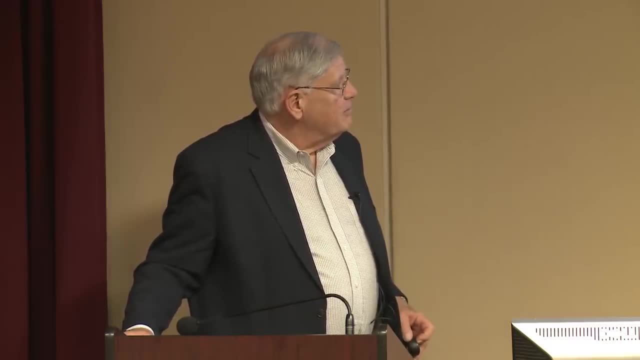 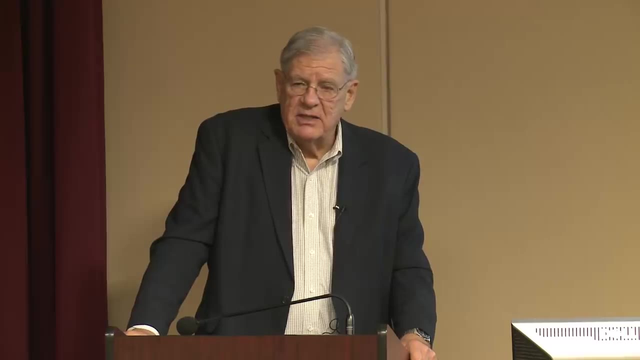 I don't think. maybe the next one was this question of the station blackout. US plants were designed to cope with a station blackout for about eight hours, And what that means is that they have about. if you lose off-site power, you lose on-site power. the diesels. you have batteries available that can power them, And they can power critical systems for about eight hours, And after that the batteries are dead and then you're up what's creek. But the thought is that you would be able to get equipment either started or operating. 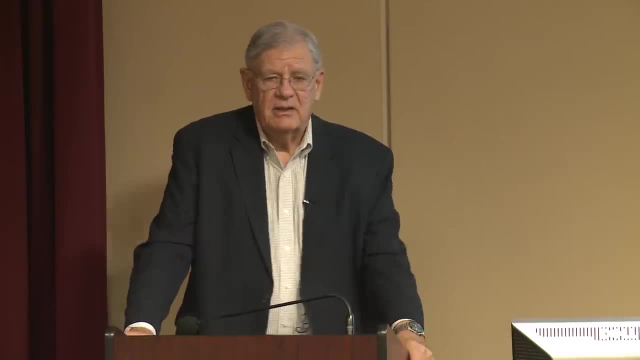 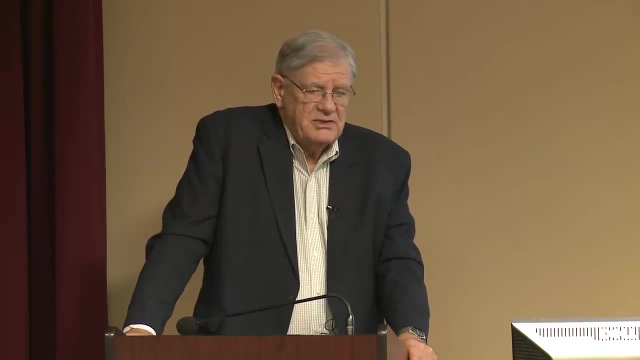 within that time period, And because of this, we started to scratch our head and say, is this really a good assumption? And so the industry picked up the ball. Right now, what they did is they've created these equipment centers around the country. 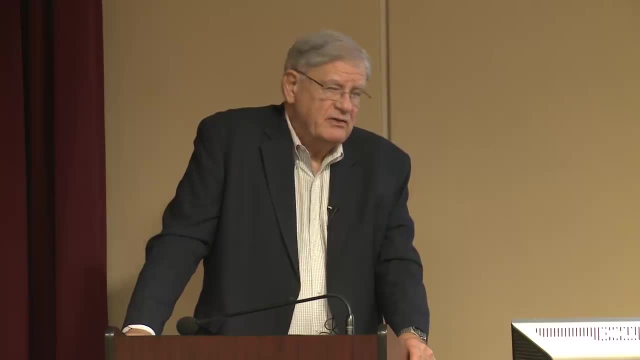 And if there is some sort of a catastrophic event that takes out off-site power at a nuclear plant and somehow takes out the diesels, so the diesels are gone, the plants have. there's a three-step approach now as a result of this accident. 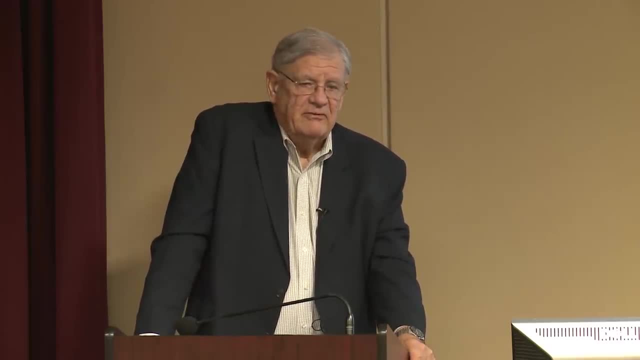 One is that they operate on the batteries that they have, which are hooked up and ready to go for about eight hours. Then they have to have other equipment on-site, either portable generators, portable pumps and the like, that they can bring in and hook up and temporarily. 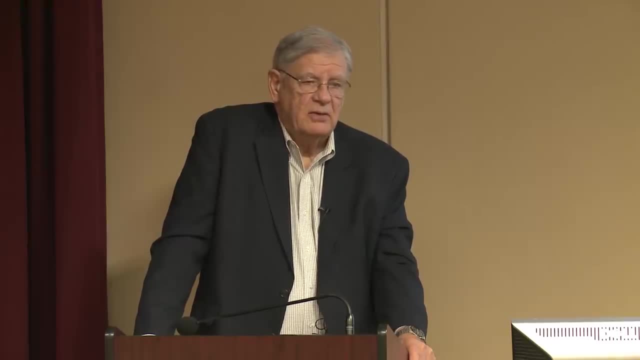 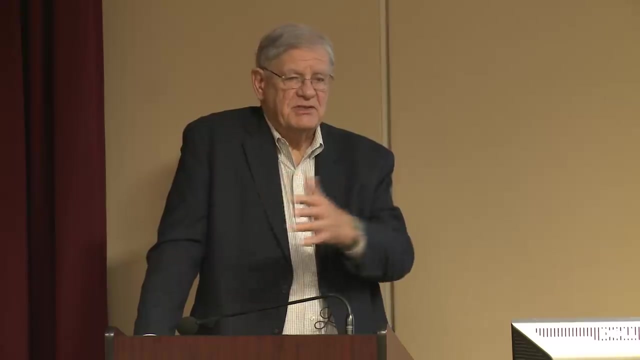 keep systems moving so that they can continue to cool the core. And then the last step is that the industry has these equipment centers around the country and helicopters and stuff, And what they would do is that before this temporary equipment that's on-site, you know, for example, 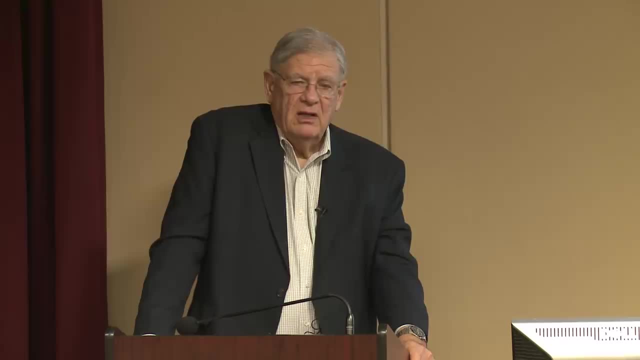 it needs gasoline to run before you run out of gas and all that. they would helicopter in this emergency equipment that could be hooked up to all the plants You know. they made sure that they have standardized fittings and everything, And these plants then could basically 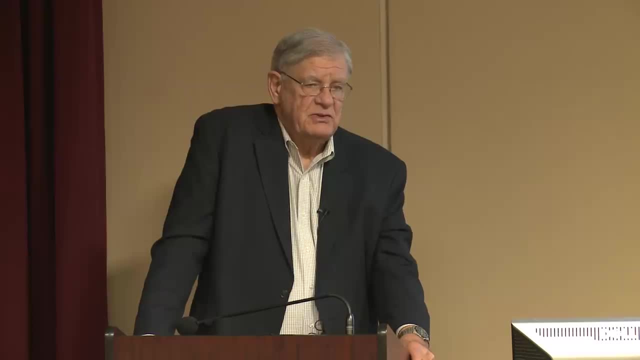 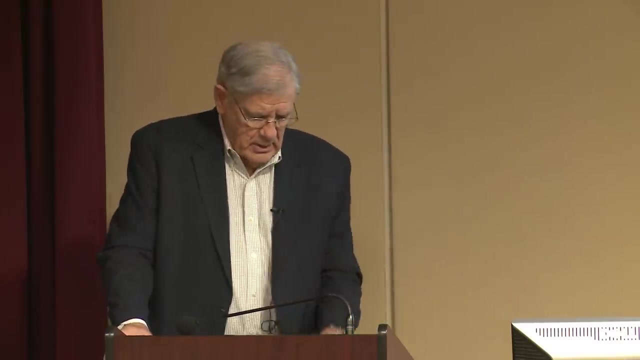 survive for an indefinite period without their diesels or off-site power. So that was one of the big lessons learned, and one of the big steps that we took following this event was to enhance the capability of US plants to withstand a complete loss of all electric power. 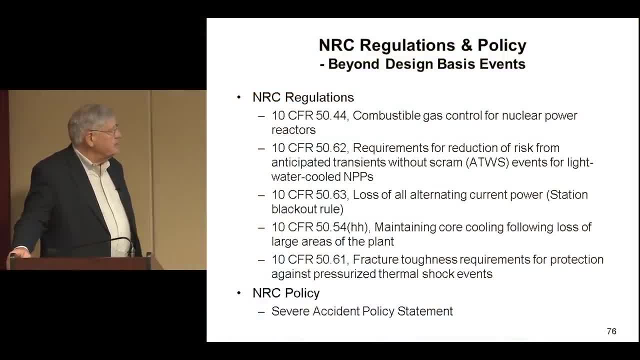 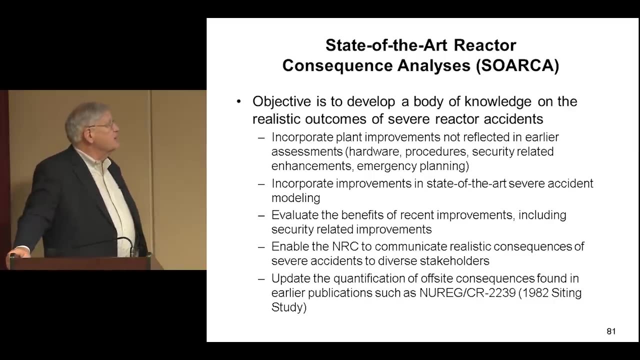 And these are just a number of the regulations that we we felt were applicable. I'm not going to get into all of them because of the time here. Now I'm going to just finish up here with what I call the state-of-the-art react to. 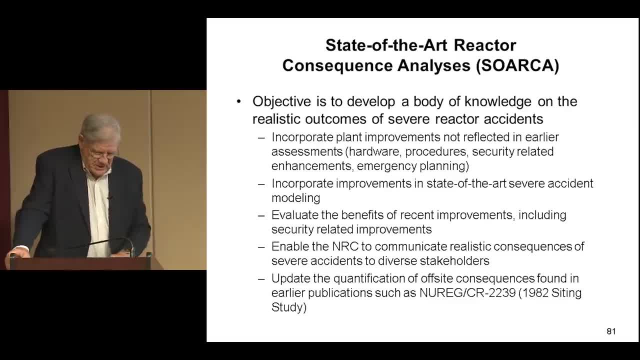 consequence analysis report and this was a study we did. The last time we did this was back in around 1990.. This kind of a study and we figured you know we've been doing a lot of research and testing trying to understand core melt. 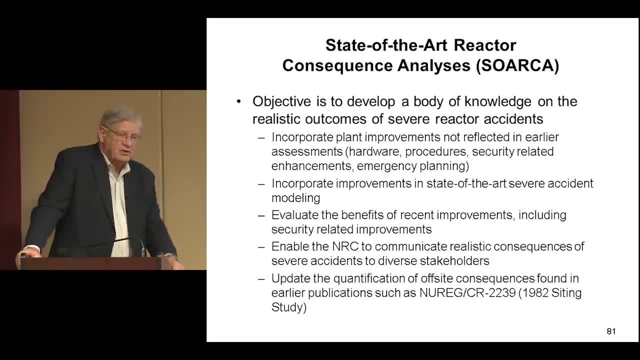 progression: fission product release, fission product transport. We've improved our analysis capabilities tremendously with our computer codes. with, because of the computer capabilities have gone up so much in terms of computing power, we can do much finer nodalization and the like, And so we decided we were going to take our best. 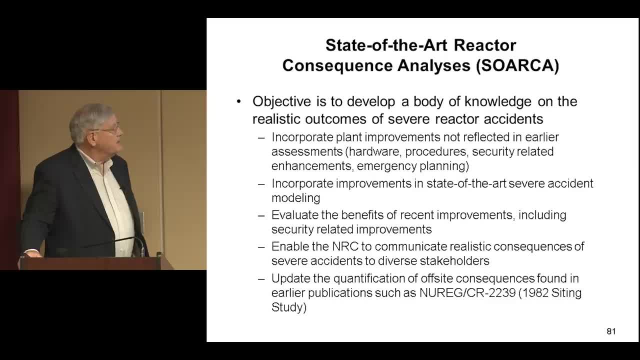 tools and our best knowledge and say: if we got a severe accident- which we call it, that's basically a core melt, something that happens, that melts the core- what is the most likely consequence? And this would also include all the safety related improvements that we made. 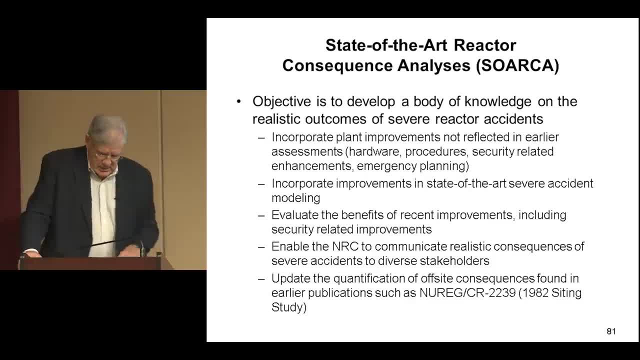 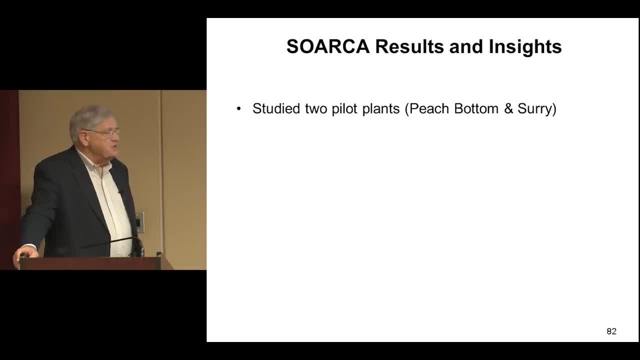 the plants over the years. Okay, and so what we did? we took two pilot plants: peach bottom and Surry. peach bottoms up in Pennsylvania and Surry's down in Virginia, down around Virginia beach area, And for scenarios that assume mitigation, which means that 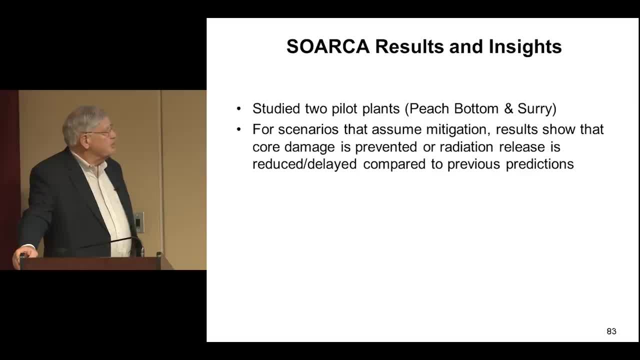 somehow they're able to determine the event. the results show the core damage is prevented or radiation release is reduced and or delayed compared with previous predictions. For scenarios that proceed unmitigated, which means that there's no action taken to try to stop the progression of the event, the results show that radiation release is reduced. 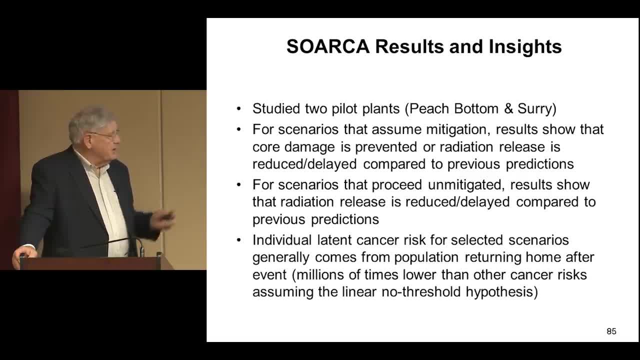 and delayed compared to previous predictions. The individual latent cancer risk for selected scenarios generally comes from the population returning home after the event. okay, which is millions of times lower than other cancer risks. assuming the linear no threshold hypothesis: okay, And that's controversial in and of itself. 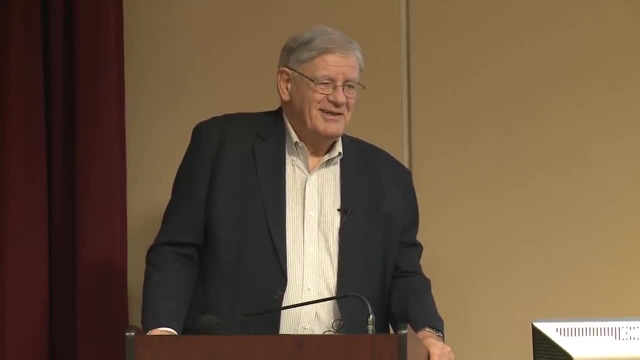 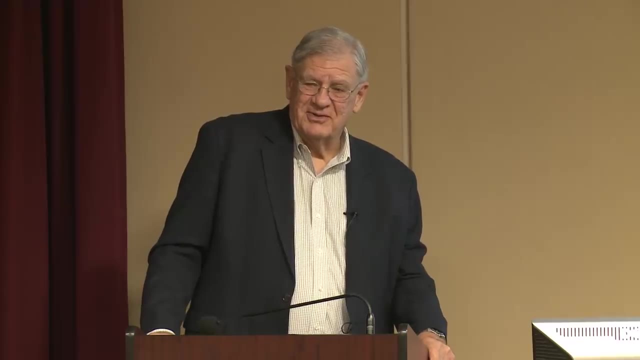 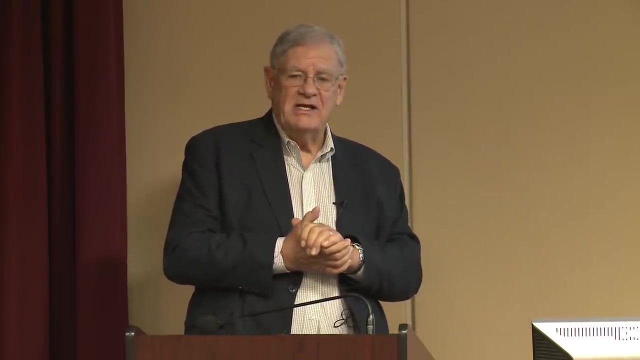 If you guys ever want to have a- you know a speaker, come in, have somebody come in and talk to you about the linear no threshold hypothesis versus other scenarios, Other theories in terms of you know, because people say the no threshold says that no radiation. 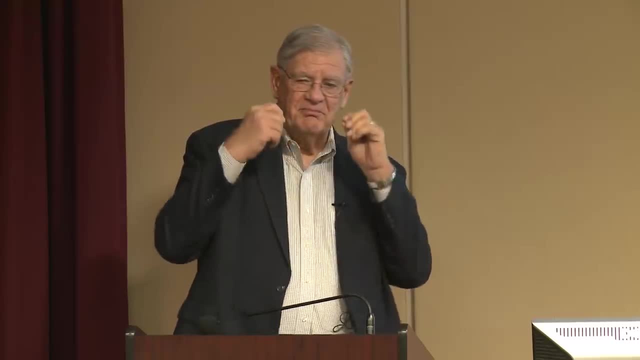 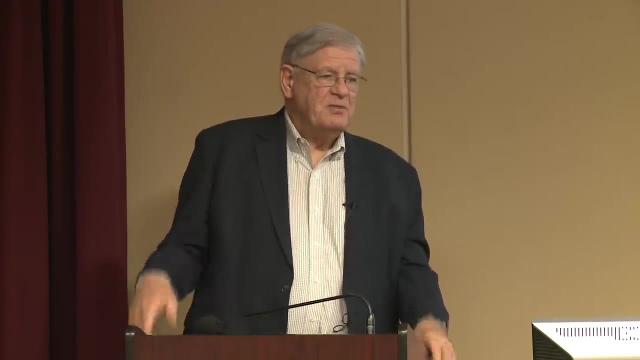 is good for you, okay. which means that even the minutest amount of radiation is going to predict some pop, some percentage is going to get cancer, okay. And yet other people say, wait a minute, we're exposed to radiation all the time, okay. 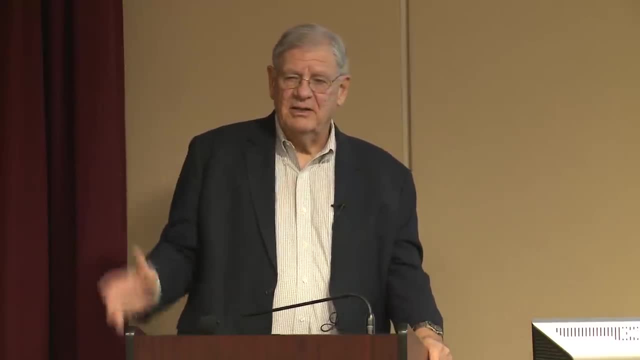 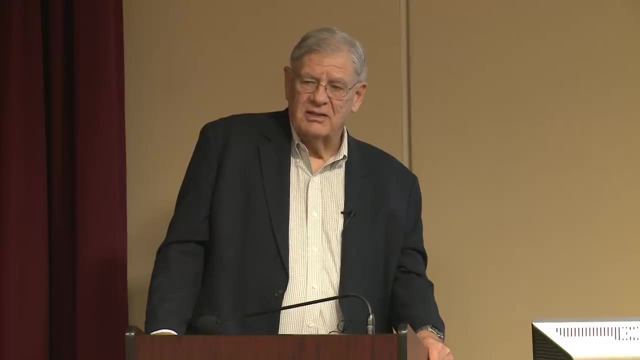 Look at the people in Denver. okay, They get much more. You know you fly in an airplane. okay, Everybody gets roughly 600 millirems a year of radiation: 300 from natural radiation, 300 from natural causing substances and about 300 from medical tests. 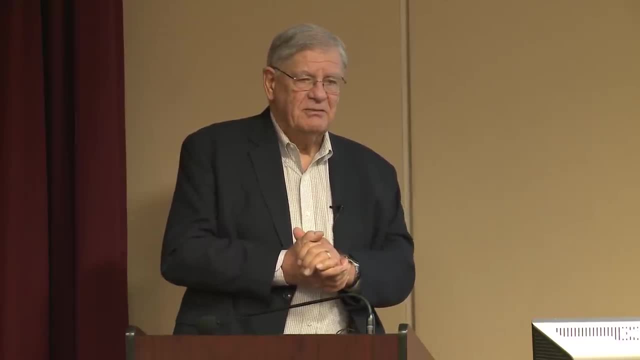 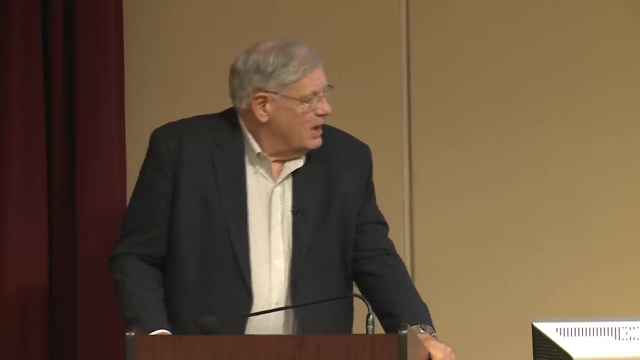 And so the point is is that you know well, people aren't dropping over from cancer because they get 600.. So maybe that's a threshold, you know, or maybe it's something even higher than that, But we used the linear no threshold, which says that even small amounts of radiation, 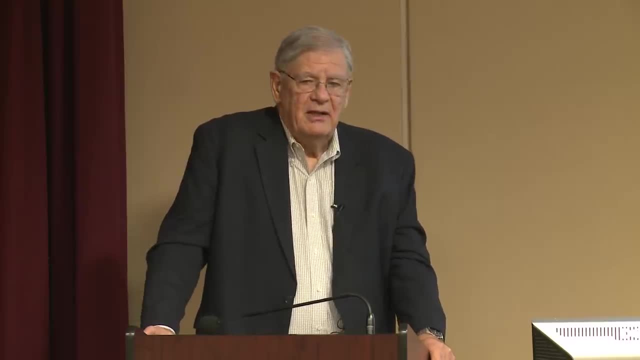 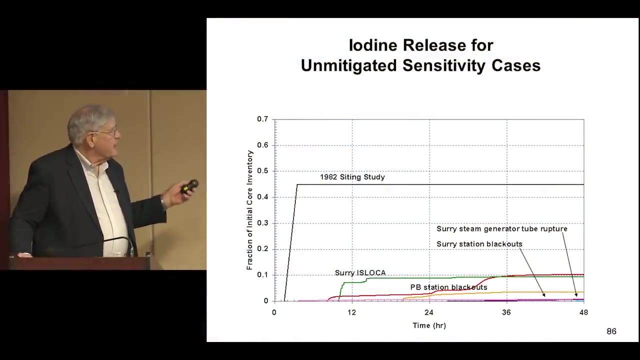 can cause cancer, And what we concluded was that: Okay. So what happens is in these events, and this will show you the: this is the fraction of the initial core inventory. okay, that's released. and this is the time- This was a 1982 study that was done. It was very conservative and it was admitted to be very conservative. But you can see here for Peach Bottom and Surrey: okay, Peach Bottom, you don't start to get a release until about eight hours. Okay, And it looks like Surrey, you get about at 10 hours you start to get a release, okay. 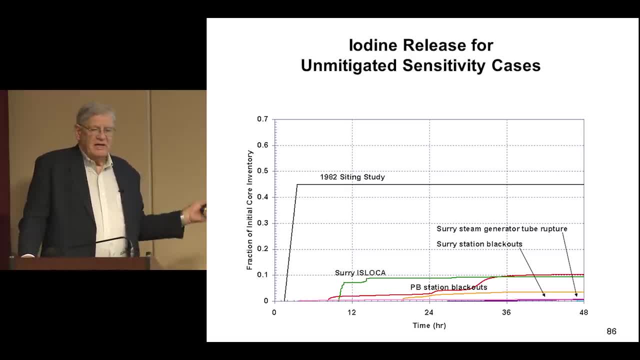 What does that mean? Okay, Well, if you have an accident, okay, what's the first thing the governor you're going to do? You're going to ask the governor, do I evacuate? Okay, Well, if you evacuate, if you assume you have an evacuation, okay, in eight hours most. 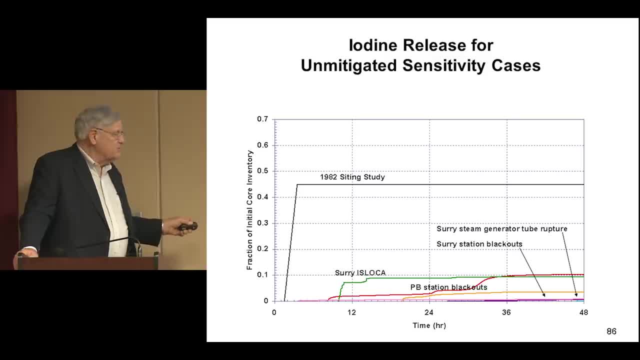 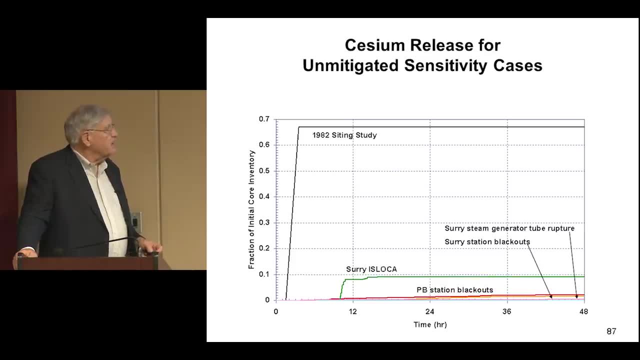 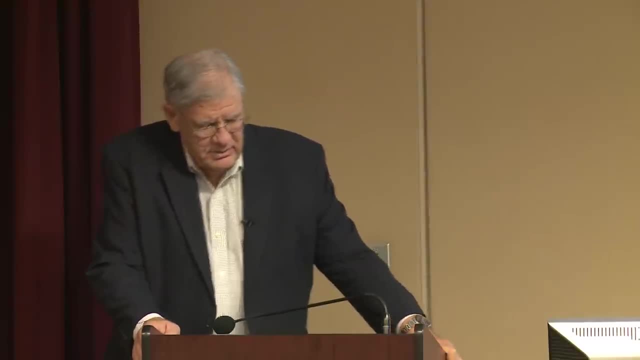 of the people are going to evacuate out of that area. Okay, In 12 hours, even more time, Okay. So when we do the study and we make assumptions about the evacuation, this is the cesium release, but what you conclude is that when the release actually occurs from the plant, in other words, 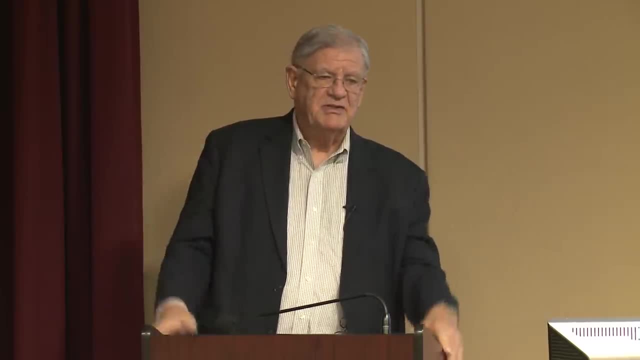 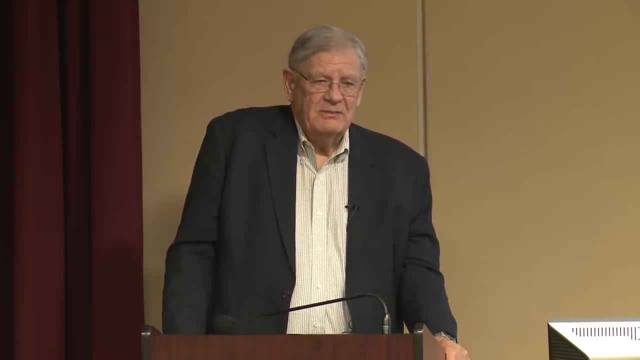 you assume that that containment finally fails and material gets released to the environment. everybody's gone. They're evacuated, Okay, They're out of harm's way, All right. And again, it's not a financial disaster, All right. I mean, you're still going to have contamination and everything in the land, okay, but nobody. 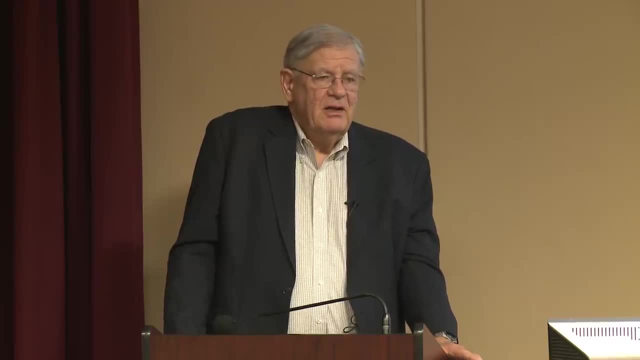 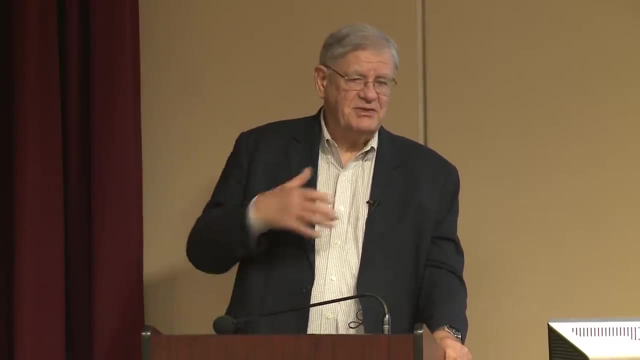 got irradiated, Okay, They're gone. Okay, They're out of there. And so what you conclude is that you know, and you know this gets into a controversy area with the NRC- and that is: do we just protect public health or do we also protect economic? 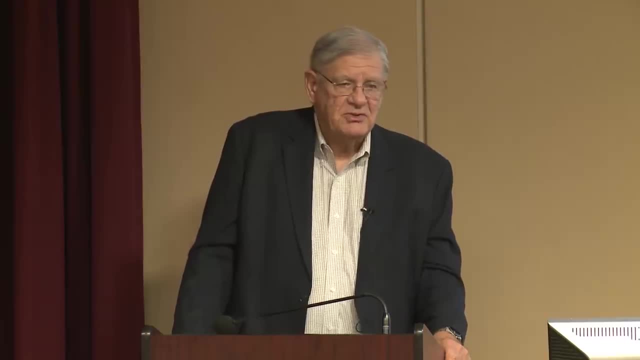 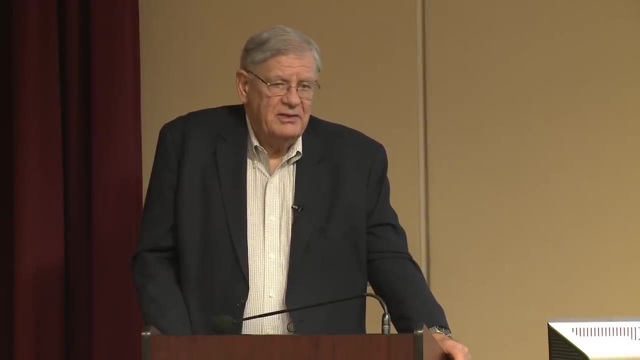 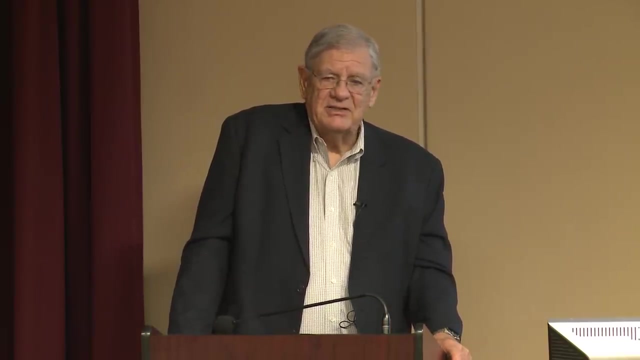 Okay, And that's sort of a policy issue our commissioners always debate, But But the conclusion was: is that people are gone, They've evacuated, So they don't get irradiated. So where is the concern coming from? Well, it's actually. it's not even NRC, it's EPA which sets the radiation standards. 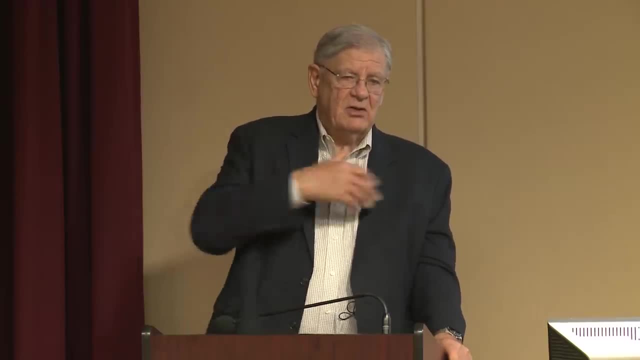 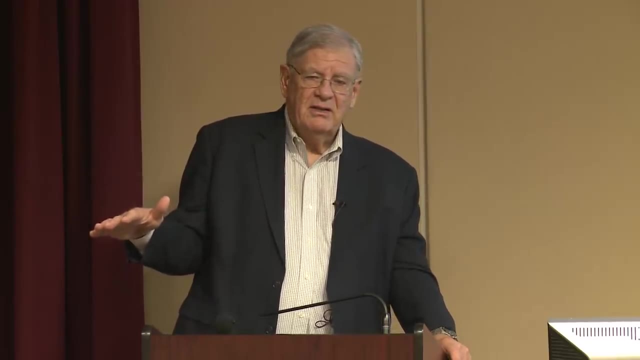 Okay, And it's- when you assume that they've done all the cleanup and that they've gotten the radiation levels in the contaminated area below the EPA limits- okay, that you allow people to come back in, Okay, And they're able to re-habitate the place. 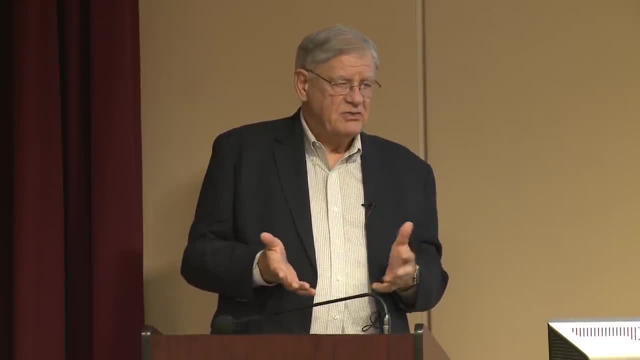 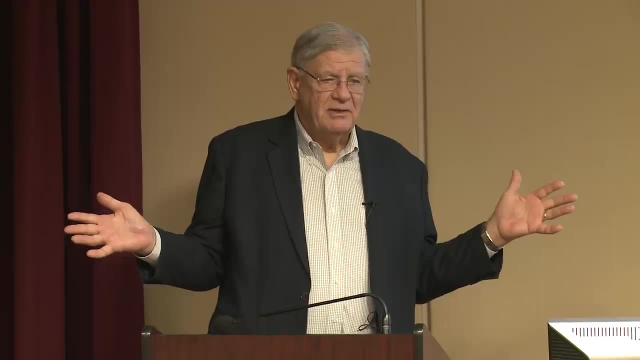 And what you do is you take a very low radiation dose, which is, you know, basically the EPA limit. You take a very low dose and you multiply it by a very, very large population and what happens is you will always get some calculated amount of latent cancers. 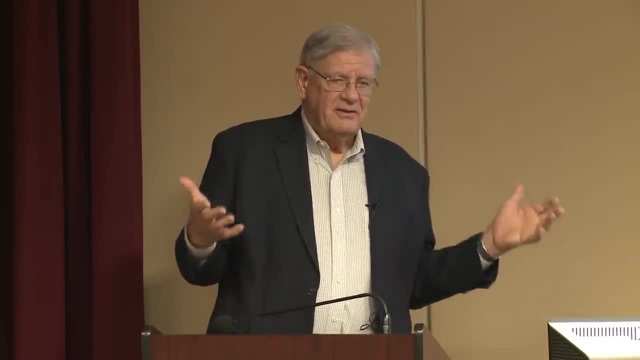 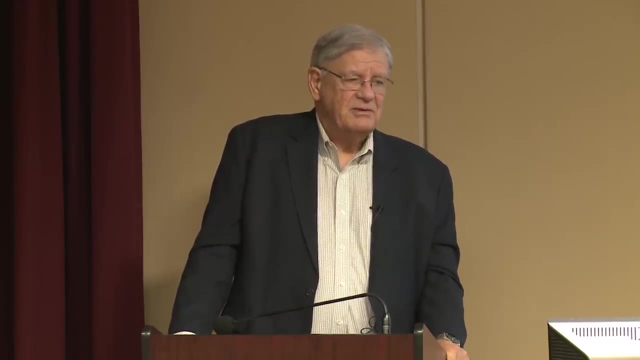 Okay, And that gets into the area of you know. do we believe the no threshold theory, or is there some threshold, you know, and is that a danger? Okay, But the bottom line we came up with was that nobody's going to get hurt from the initial. 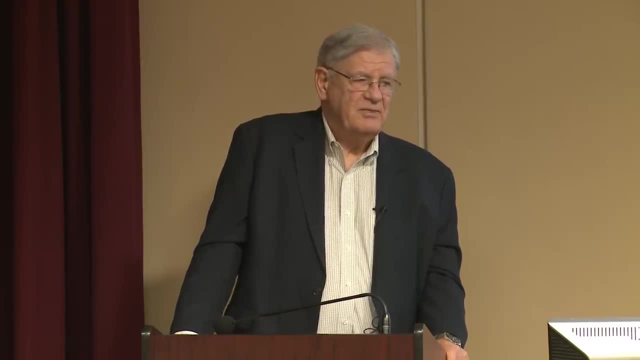 part of the accident when there's a release, because we have enough time to get people evacuated from the study, because these events progress much slower than what we had previously predicted and that the releases are a lot less, And the reason is because we know more now. 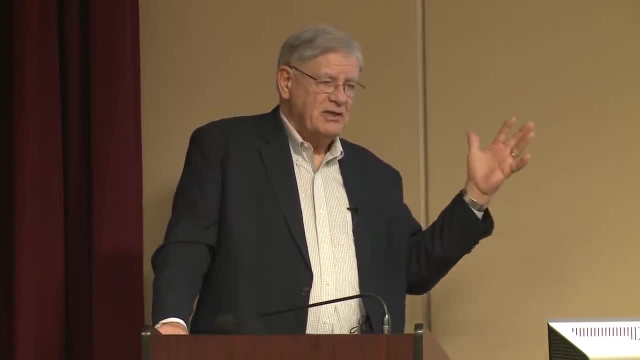 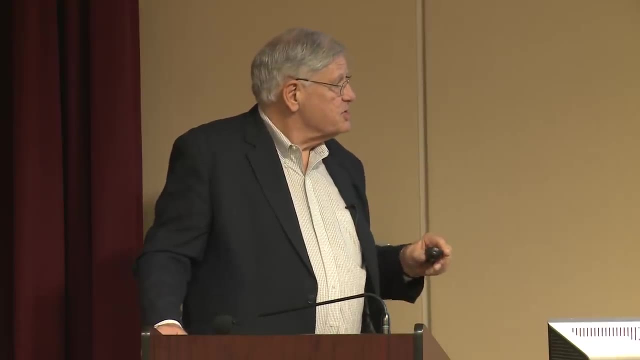 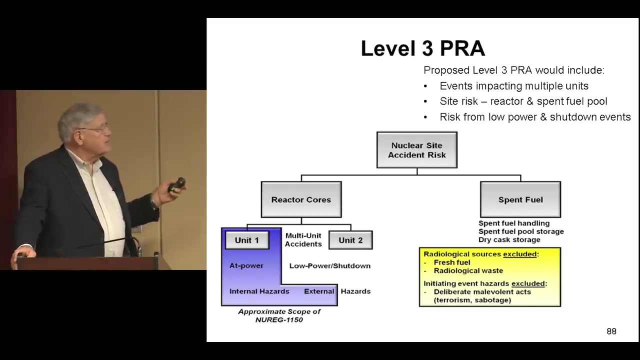 We know that material that gets released in the containment plates out on the inside of the containment- Radioactive material. It doesn't just hang in there and get released. Okay, It plates out, So you don't get as much released. And right now, when I retired the last thing we were going to start doing, I started this: 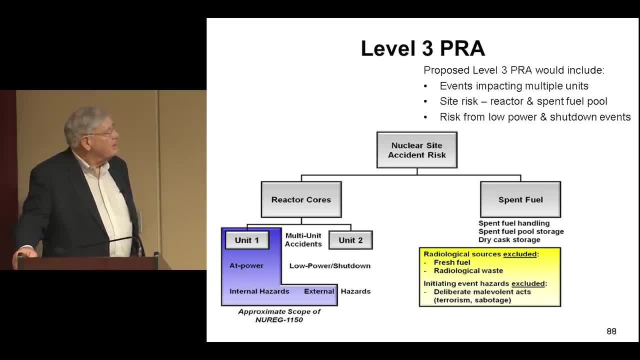 actually was to do what we call a level three PRA. Level one PRA is where you just calculate the risk of a core melt. So if somebody says what's the probability the core is going to melt, okay, you can give them a number. 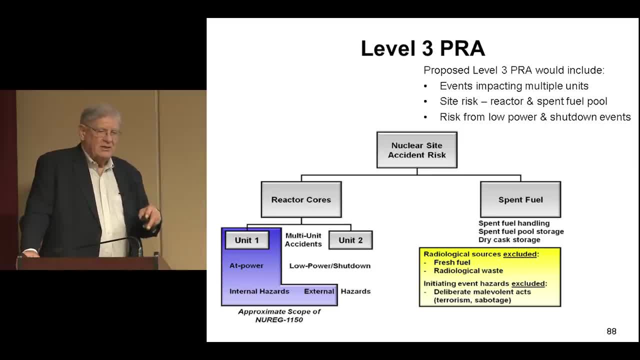 If you do a level two PRA, You not only calculate the probability of a core melt, but you also calculate the probability of a release. What's the probability that core melt will ultimately lead to a release? And then, if you do a level three PRA, you go the full nine yards and you say what's? 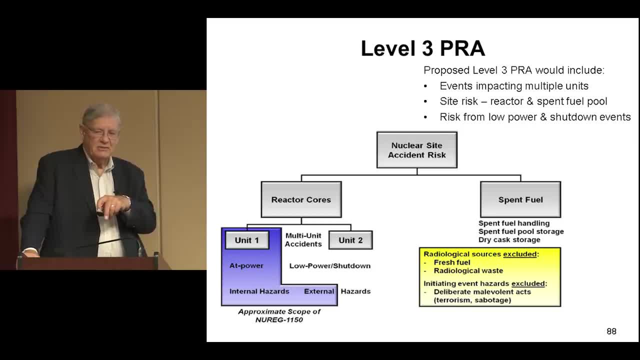 the probability somebody is going to die or get latent cancer from that accident. okay, So we're actually doing a level three PRA. We want to look at two different things. What we've always done in the past is just the reactors. 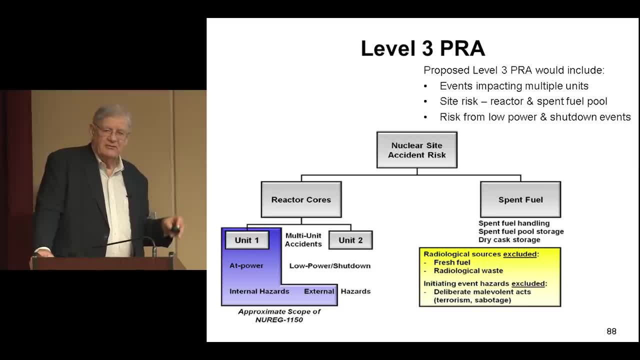 We always said: what's the risk per reactor year. full power reactor year, That means if the reactor was operating for full power for one year, what's the risk of living next to it and getting cancer or dying or whatever? But there's a lot more to it. 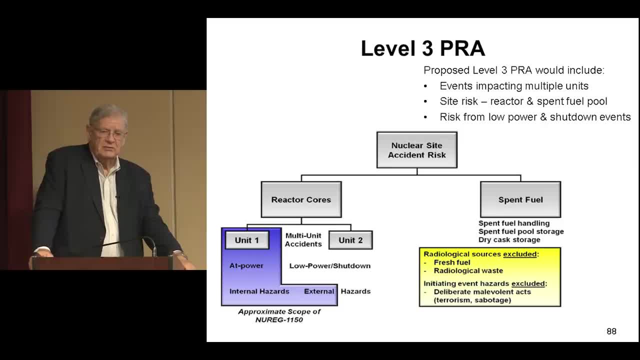 One is that most plants are multi-unit sites. they either have two or three reactors there And you might speculate and you say, okay, you know well, if whatever caused one meltdown, like a station blackout, won't that happen with the other two? 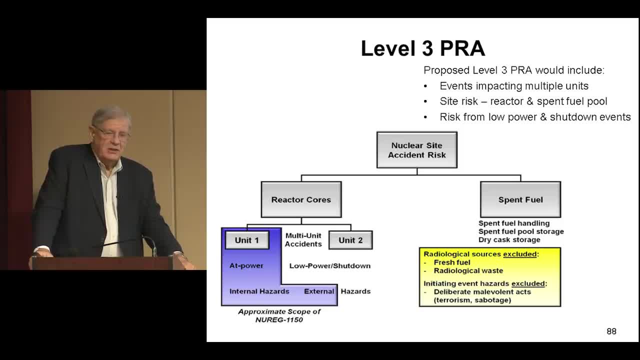 It might. So I wanted to do a study where we said: let's take into account the probability of not one reactor, but maybe if there's two reactors at that site, they both experience the same problem. What's that likelihood and what does that mean for the dose rate and everything? 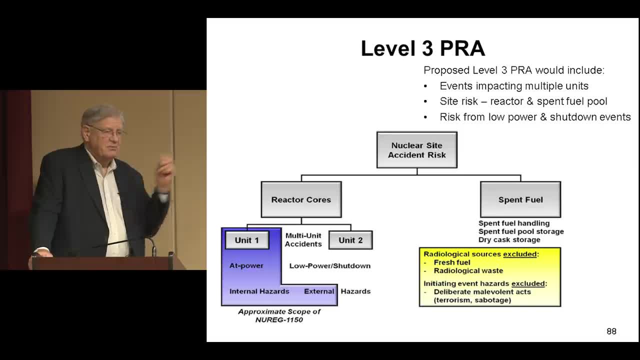 The other thing that's on site is spent fuel And that was a big problem. Yeah, That was a big concern at Fukushima. When nuclear fuel comes out of a reactor it's still very radioactive. It's still very hot, okay, physically, you know, thermally hot. What they do with it is that they put it in a spent fuel pool, okay, which is a big swimming pool. basically that, this water that goes in there And this stuff stays under water to keep it cool. It's got to stay there about five years, okay. 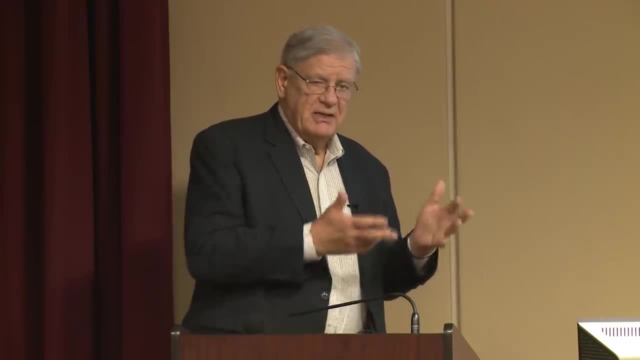 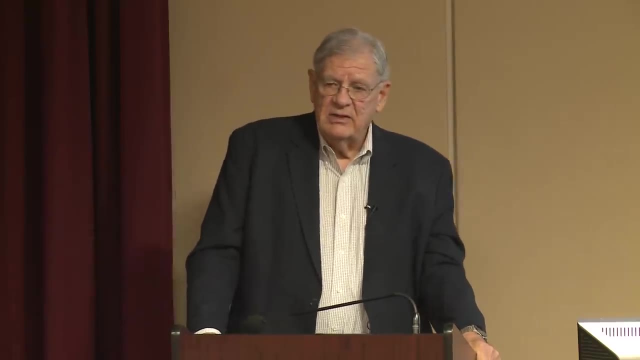 Once it's been in there about five years, the heat generation has decayed down enough that it can actually be cooled down. It can be cooled in air without overheating, And what they do usually after about five years is they can take it out of the pool. and put it into these big concrete cylinders called spent fuel casks And these can be air cooled. They have holes in the bottom. They just use natural circulation air And they put them in these big concrete containers. They're about 20 feet high, 10 feet in diameter. 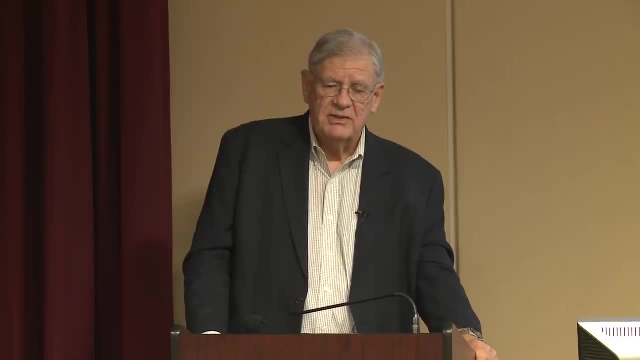 They hold, I don't know, maybe about a dozen or a couple dozen fuel assemblies. They seal them up and they put them out on a concrete cask near the plant, And now they're just waiting for the government to figure out where they're going to dispose. 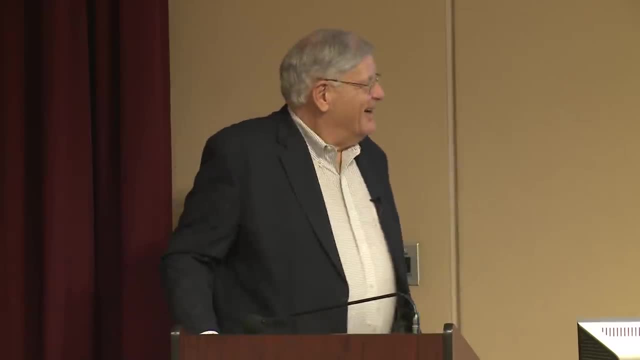 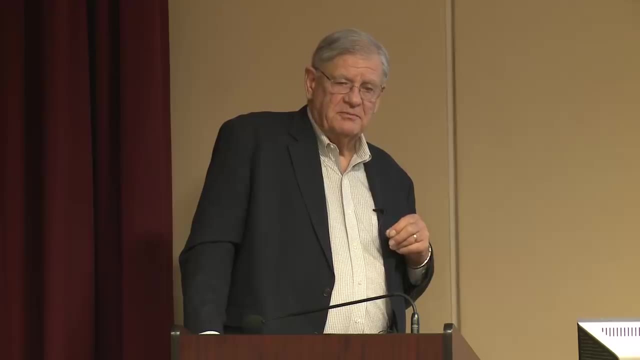 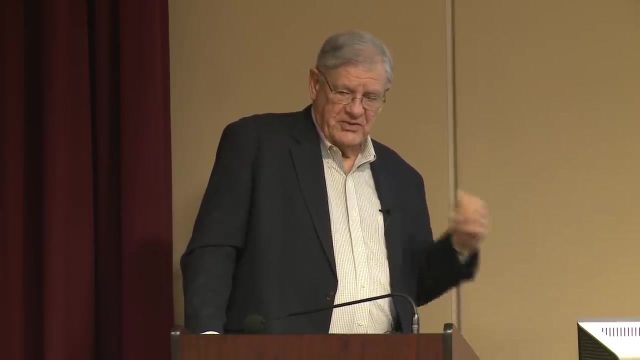 it. Okay, And that's a whole other issue I won't even discuss. But there's always a concern of, well, what happens if you lose cooling to that spent fuel pool? Okay, Turns out that there's so much water in those pools it would take forever to boil it down. 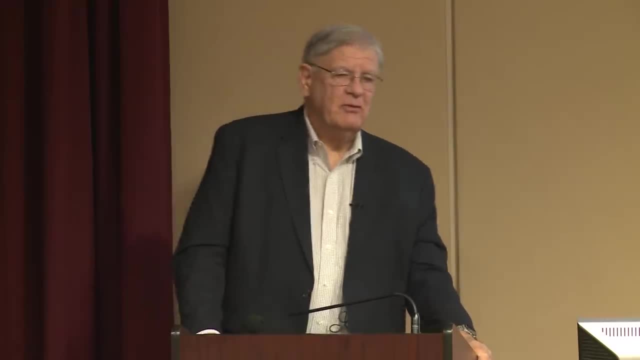 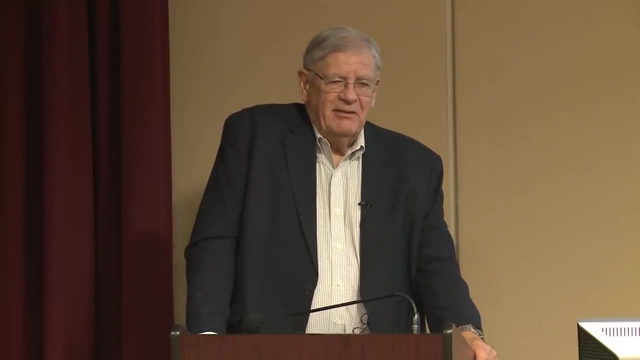 just from the heat. So then we get into the question of: well, what about a terrorist? What if they dropped a shape, charge down and blew a hole in the side and everything? It's like. you know, one of the things NRC does not do is come up with a risk of terrorism. 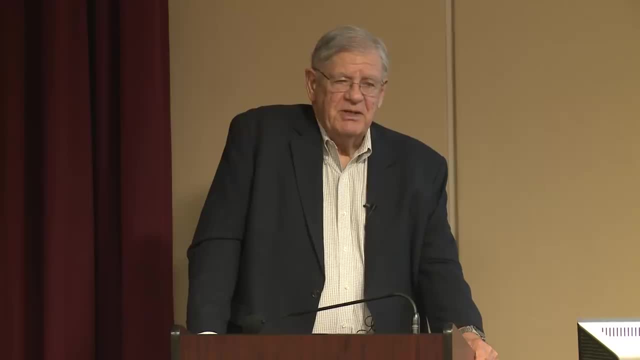 or a terrorist event. Okay, And the reason is: is because we don't know what the probability is and we don't know how to put a probability on a terrorist event. Okay, What's the probability? someone's going to plow an airplane into a plant. 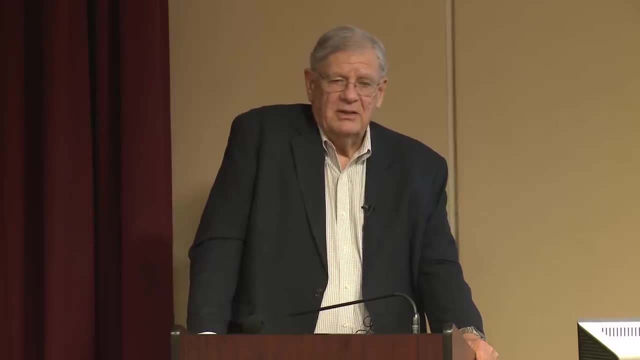 Okay, Or two airplanes, Okay, We don't know. Okay, We do have a design basis threat at plants. We have security forces there that are well trained to fend off any kind of an attack by terrorists, up to a point. But some people will say, you know, at some point, okay, those attacks become an act of 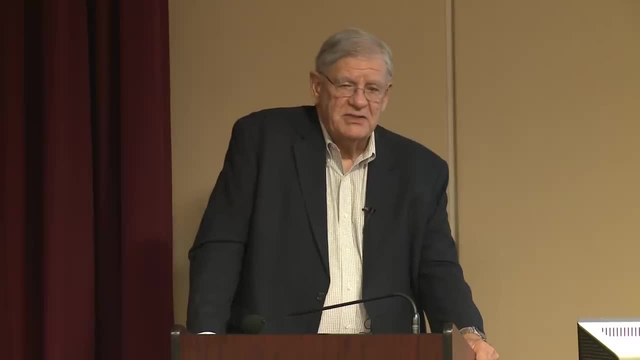 war and we don't expect a utility to defend the United States. Okay, At some point you have to say: you know, I can't expect You know, a company or utility to defend against some foreign adversary. That's when the military has to come in and take over. 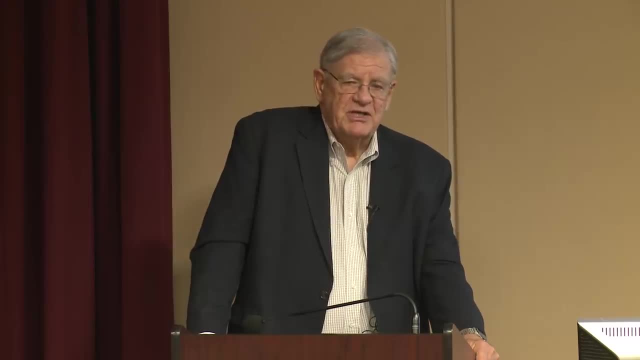 So we don't put probabilities. when we put these risk assessments, they don't include anything about terrorism or anything or sabotage. What we do is we say we have a design basis threat and we test the security crews at the plants on their ability to withstand that threat. 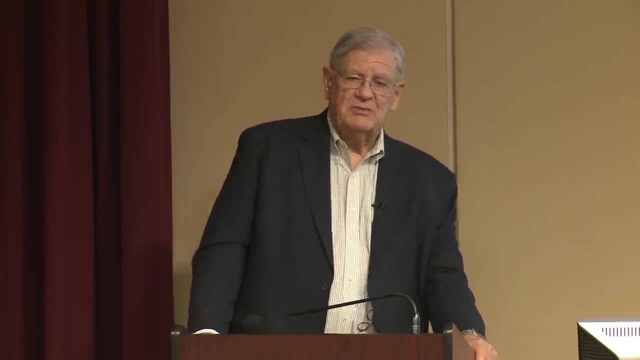 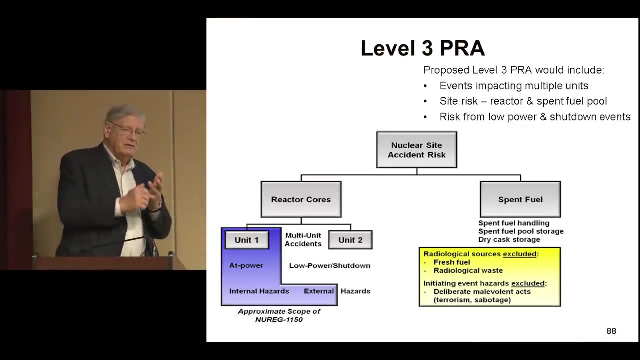 Okay, Where they have these actual rifles with lasers and stuff and they actually try and infiltrate a plant, you know, in a drill to see how well they do. But what we're doing is we're trying to combine all of the risks from a plant, from the reactor. 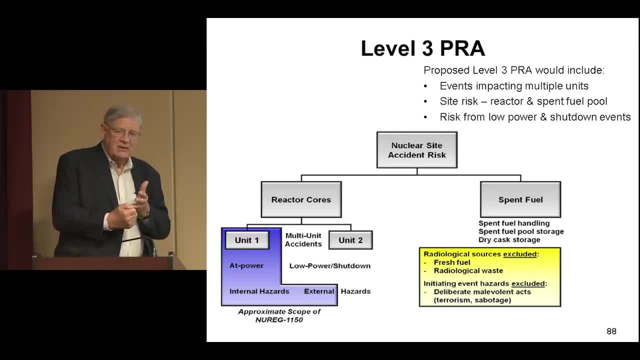 when it's running from the reactor, when it's shut down. When you shut a reactor down, you turn a lot of safety systems off. you have a lot of doors that are supposed to be normally closed, wide open because people have got to get in, and